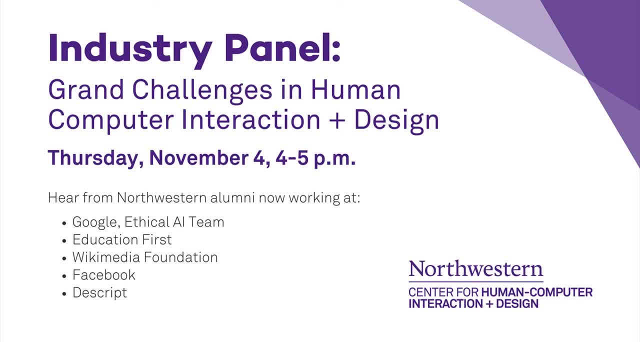 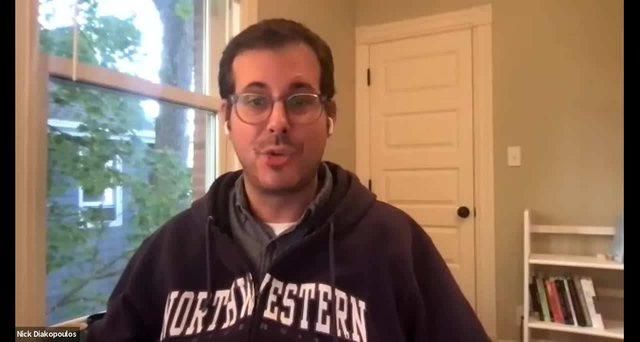 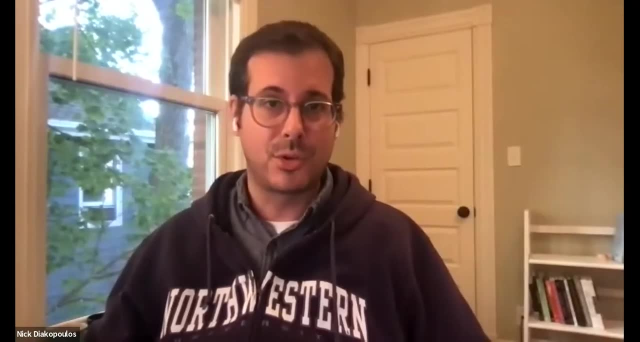 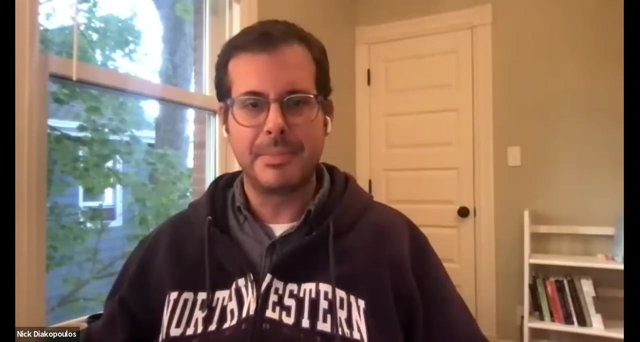 Welcome everyone. Welcome to our industry panel on Grand Challenges in Human-Computer Interaction and Design. My name is Nick Diakopoulos. I'm the director of Northwestern's Technology and Social Behavior Program, which is our joint doctoral program in computer science and communication, And I'm very happy to do my little part to help co-host today, as we're 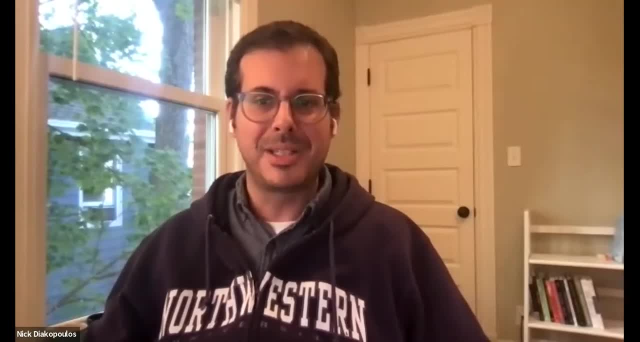 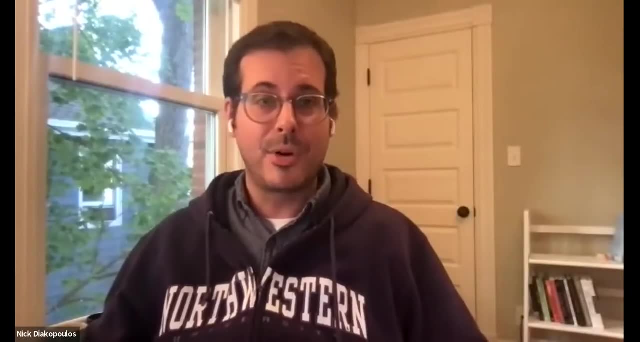 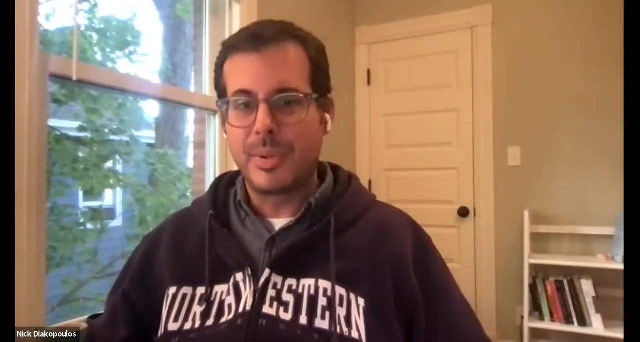 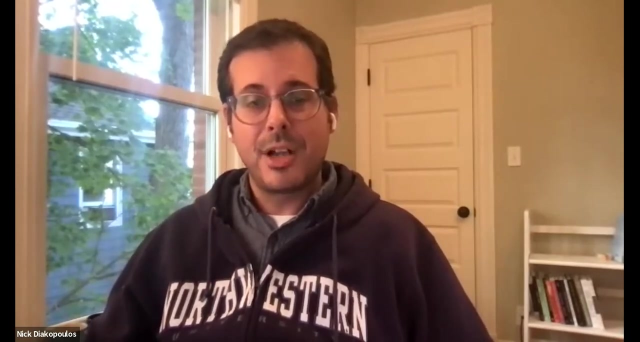 all extremely proud to see all of our alums from all of our doctoral programs playing such prominent roles in industry, And today we are looking forward to a very exciting hour of conversation with our distinguished panel. We have representatives from Google, Facebook, Descript, Education First- and the Wikimedia Foundation. Just as a reminder, we invite you. 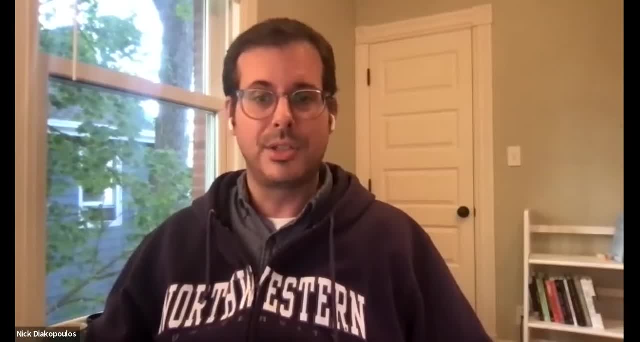 to submit questions in the QA tool in Zoom Throughout the panel, and we'll channel those to our moderator, Liz Gerber. And it's now my pleasure to introduce you to Liz. She is the co-director of Northwestern's Center for Human-Computer. 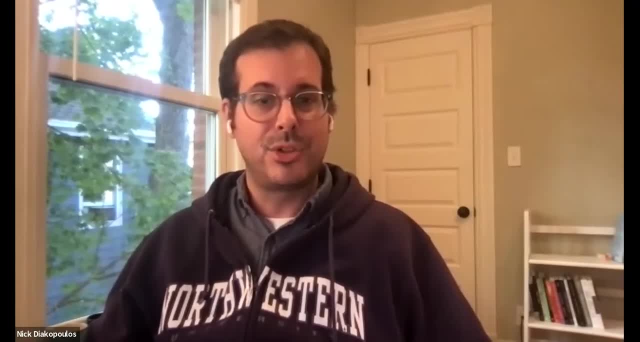 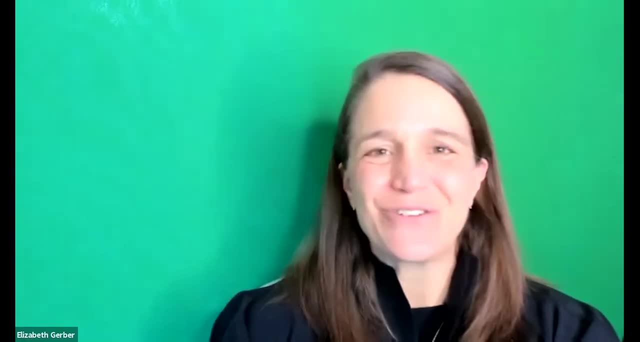 Interaction and Design, And she will introduce you to our distinguished panel and moderate the conversation in QA. So take it away, Liz. Thank you so much, Nick. Like I said, this is just so fabulous to have this wonderful panel with us. I'll give brief introductions. 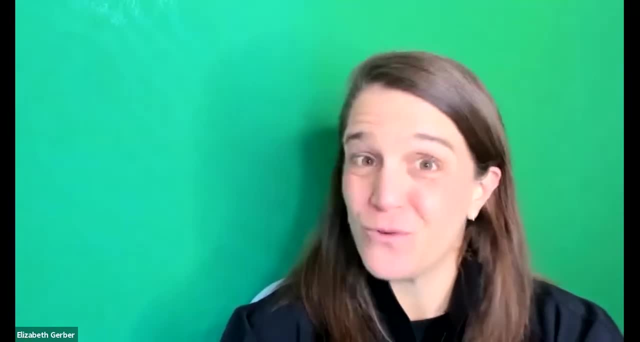 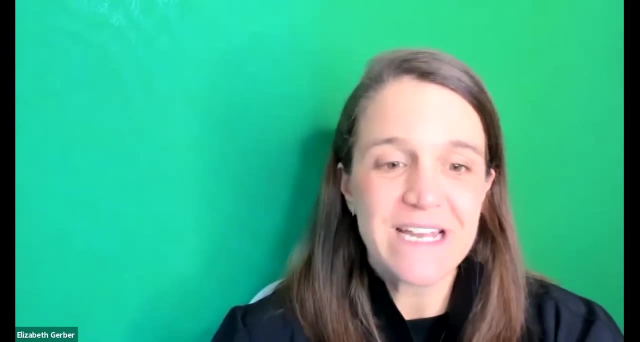 I could talk for hours about each of these people, but we'll keep it simple for now. We'll start with Mark. Mark is a research scientist on the ethical AI team at Google, where he examines the origins of values and social biases in data sets and their influence. 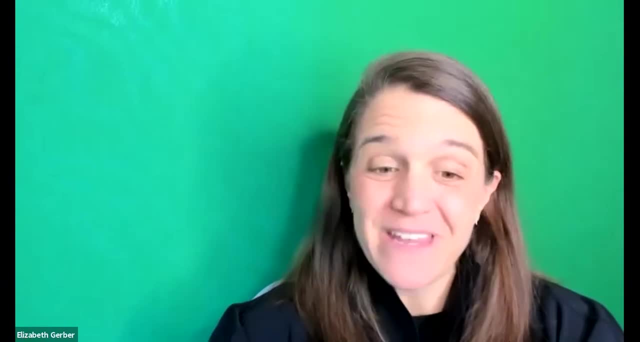 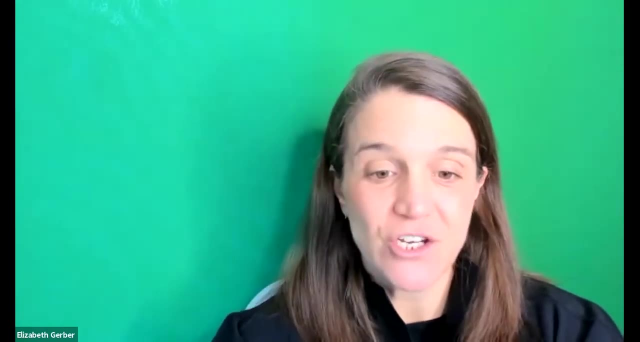 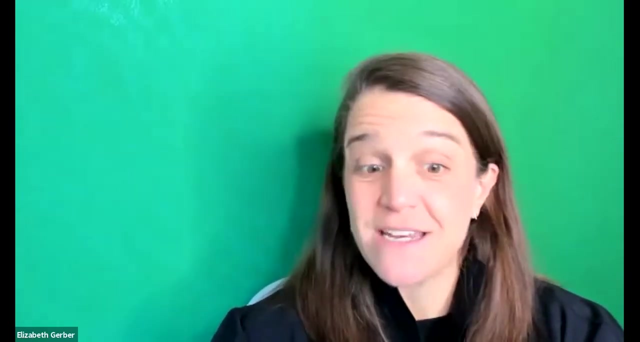 on algorithm performance. Emily is the director of Emerging Technology and Innovation at Education First and a co-founder of Brave Initiatives, a nonprofit which is training women in coding and design in prisons. Prem is a research scientist at Descript in San Francisco, where he creates machines that can. 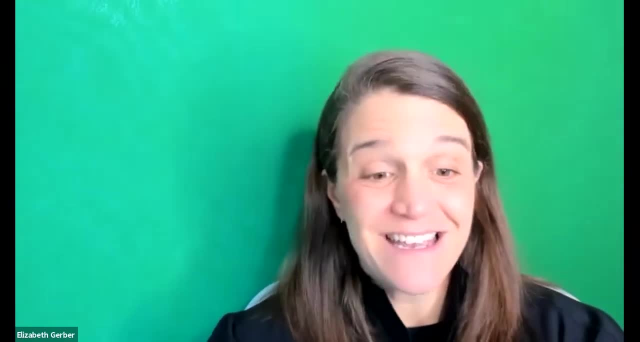 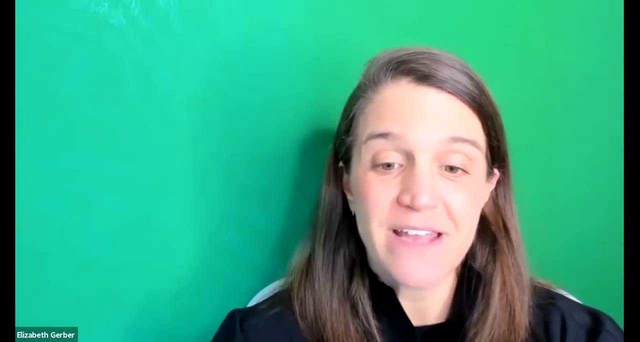 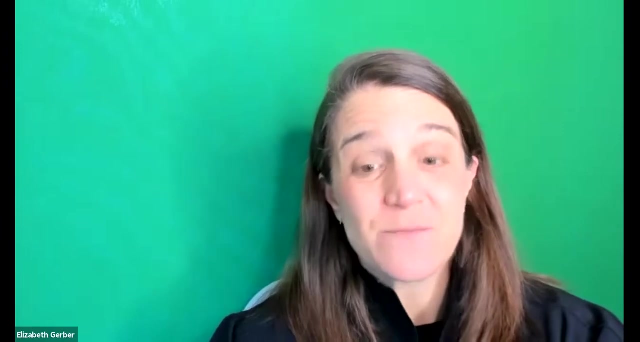 understand the auditory world. Isaac is a research scientist at Wikimedia Foundation, where he's working to understand and address how structural inequalities find their way online and into algorithmic systems. And finally, Lauren is the director of research at Facebook, where she leads the news feed and stories research team, which focuses on understanding how to best support. 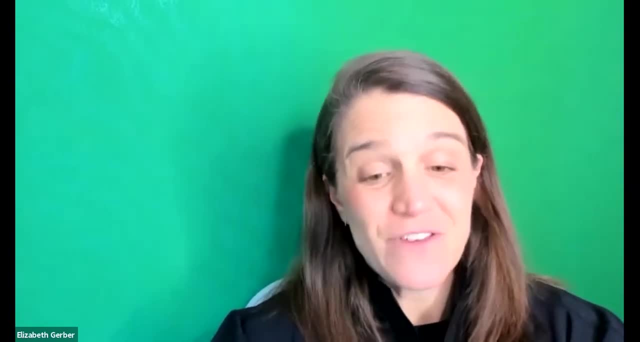 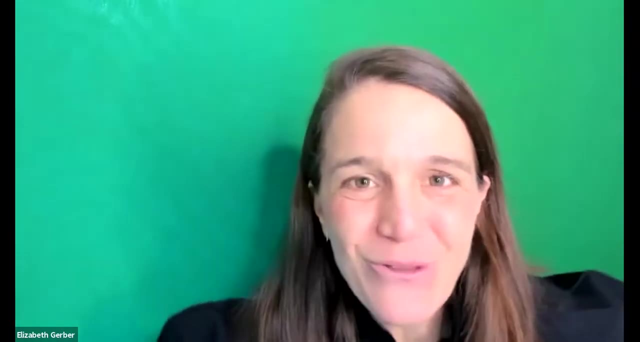 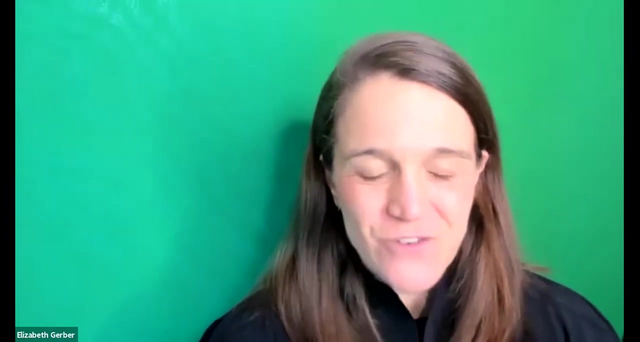 human-computer interaction. And finally, Lauren is the director of research at Facebook, where she leads the news feed and stories research team, which focuses on understanding how to best support human-computer interaction. So you can find all the resources in your tocl farther. 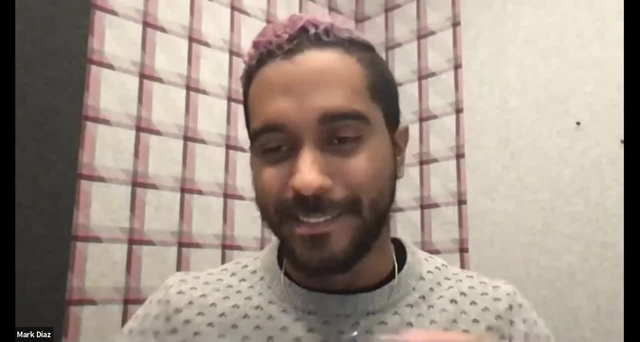 Yeah, I'm going to be a little bit biased in my sort of just like world view. I'm focusing: uh, a lot of my work right now has to do with a lot of my work has to do with large-segmented, big small-systems, Walking Address and going to work across nation. uh, Commerce and International Affairs- Our abonnement skulle be been happening this fall, So I defined my goal for the floor will be one of others years. 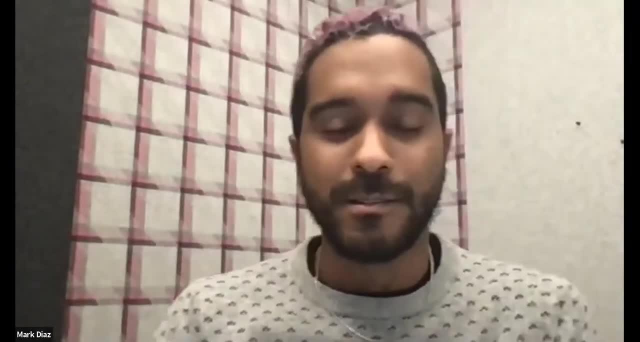 So you could maybe say your needs can be defined in your workflow. a little bit bias in my sort of just like worldview focusing of next level problem, language models, different kinds of algorithmic systems And, I think, one of the biggest challenges. 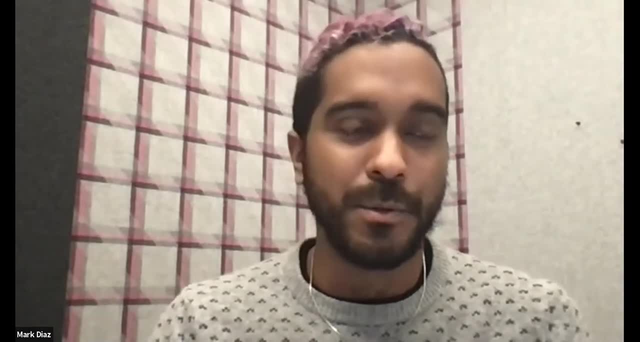 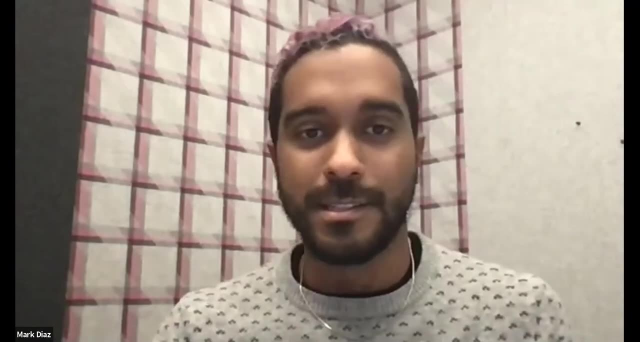 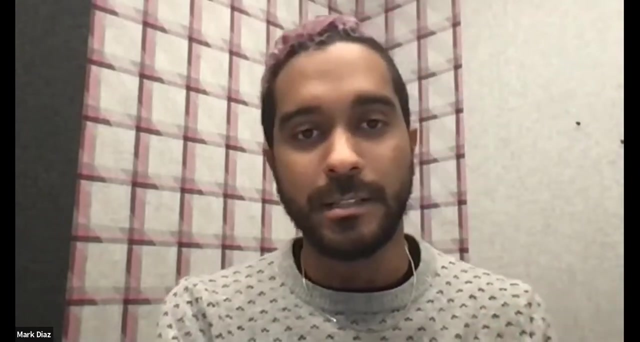 that we are thinking through is how to broaden participation in the creation of these systems. There's a lot of different challenges, ranging from sort of norms and culture around who usually gets to do work on technology broadly, but also AI. There's also challenges speaking across disciplinary. 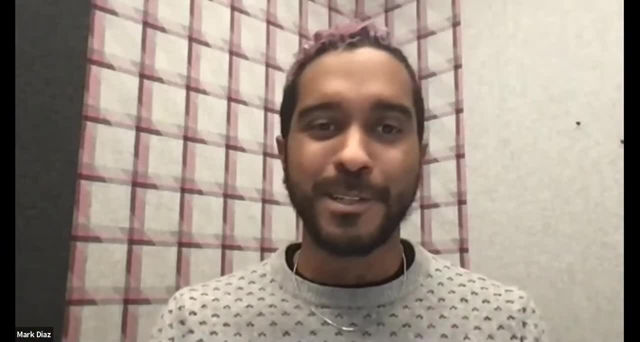 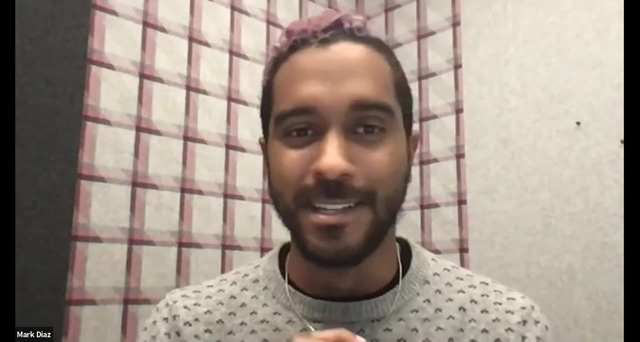 boundaries which, very weirdly, I run into all the time. I work with a lot of people who are very traditional machine learning researchers and sometimes I'm looking at them with a blank face, they're looking at me with a blank face, and then we just gotta push forward. 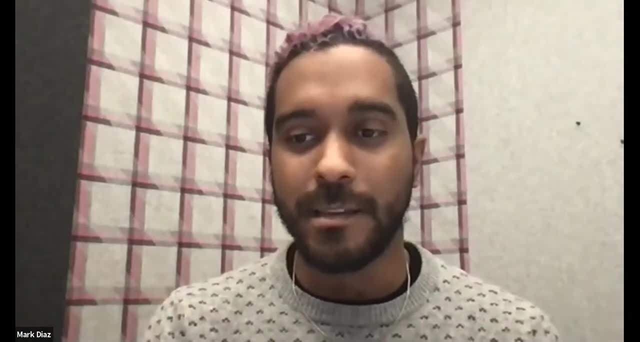 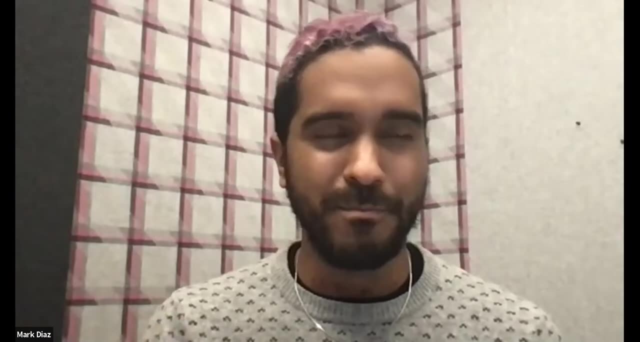 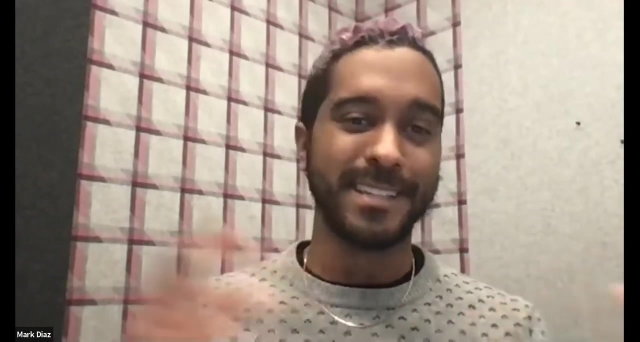 somehow, but also ultimately trying to get perspectives from folks who are gonna be using systems or are not necessarily users but stakeholders in some other way, and that they're offering or not offering, but their data is, by different processes, part of data sets that we use. 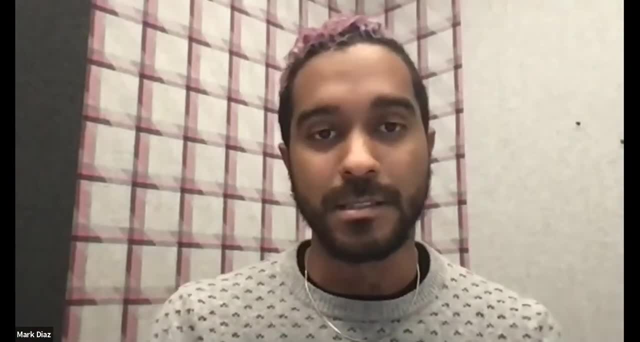 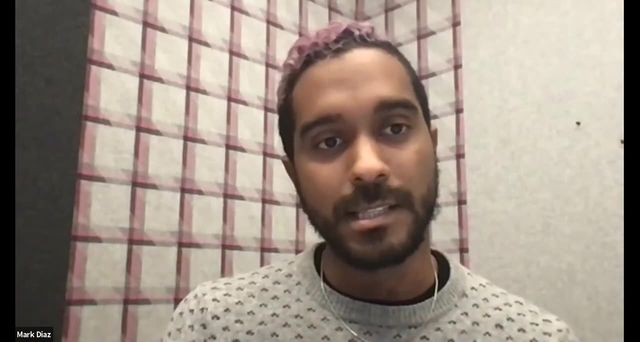 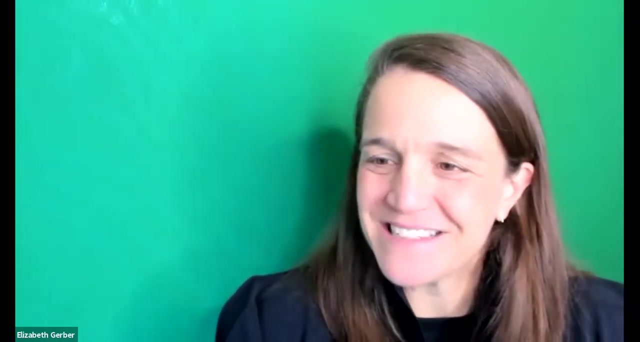 or they're otherwise impacted somehow, because systems are used at scale, And I think that last group of people getting their perspectives, is one of the biggest challenges that I see. Thanks so much, Mark. So broadening participation in some. Next let's hear from Isaac, and then followed by Emily. 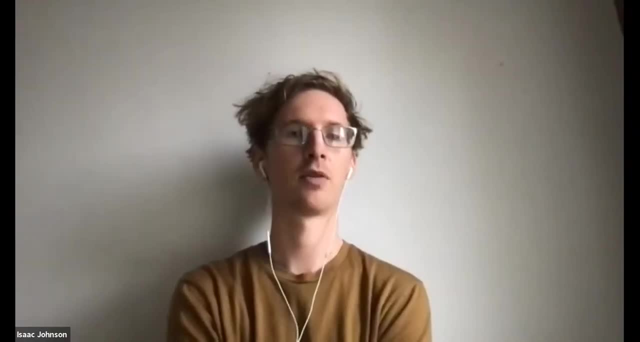 Thanks, Liz. I just wanna give a little bit of background on Wikimedia Foundation too for those who aren't familiar with it, to kind of understand where I'm coming from. So Wikimedia Foundation is the nonprofit most notably we support Wikipedia, but there's a number 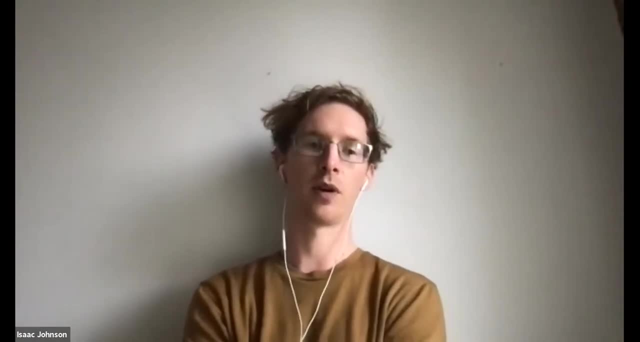 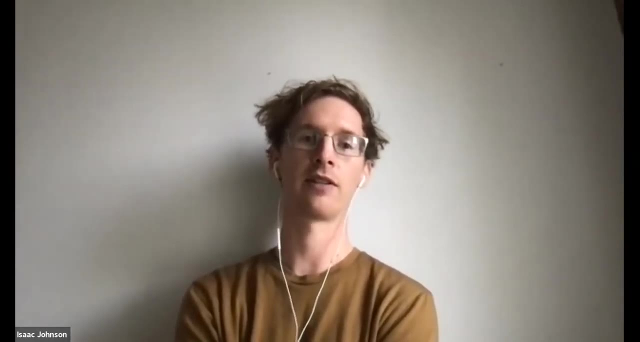 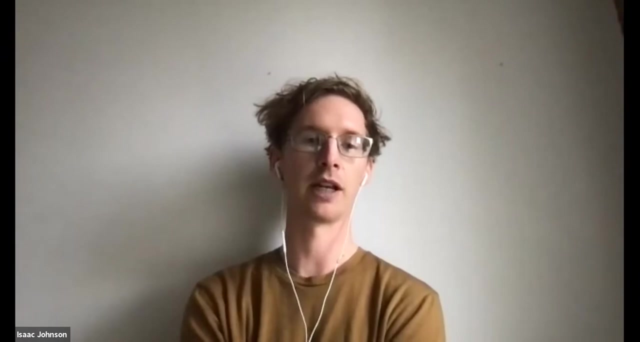 of other sister projects that we support as well, Where support means keeping the site running, building tools for editors, doing advocacy work, trying to increase access to free knowledge- essentially everything but the actual editing of Wikipedia, And so that's kind of what I'm bringing. 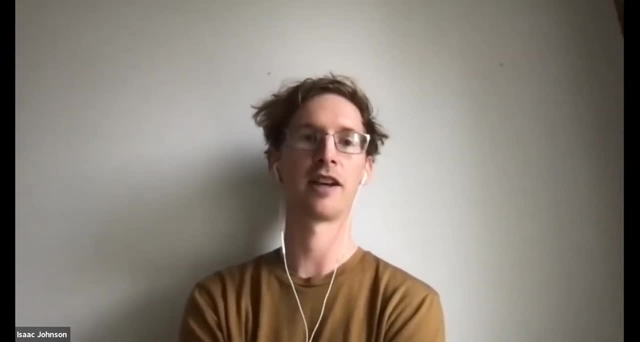 to this conversation today And I'm really glad that Mark said all the things he just said, because it makes my job a lot easier, because I wanted to talk about language equity, which I think is a very related challenge, And when I say language equity, I'm thinking 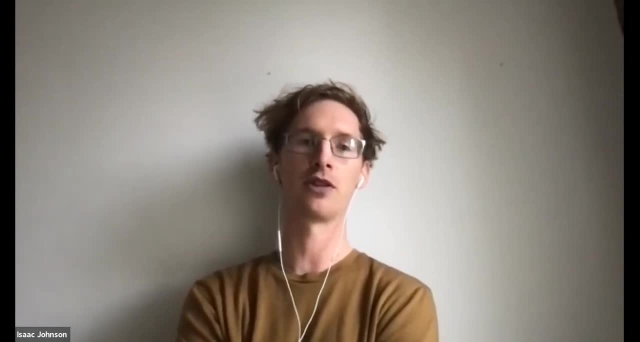 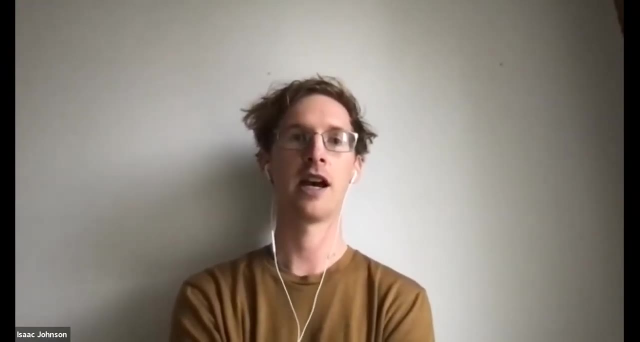 I'm talking about essentially like the language you speak shouldn't be a barrier to accessing of knowledge and tools, but obviously right now very much is, And within Wikipedia we have over 300 different language communities that have their own Wikipedia And obviously there's a lot of variety. 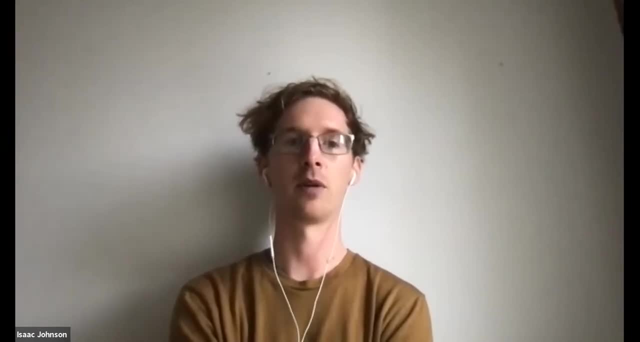 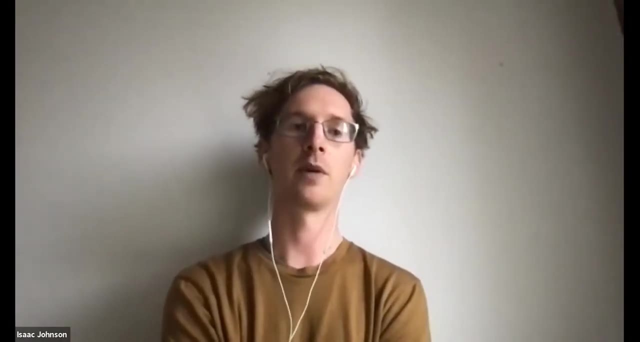 over the amount of content that's available and the tools that are available to these editors. So, within kind of design and HCI, when I think about this, I'm thinking about what language communities are we including in our research when we're doing computational social science type work? 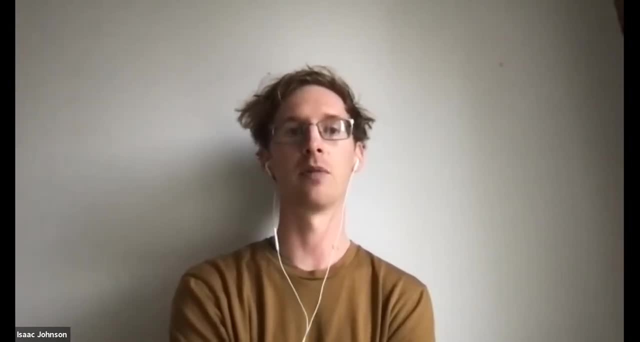 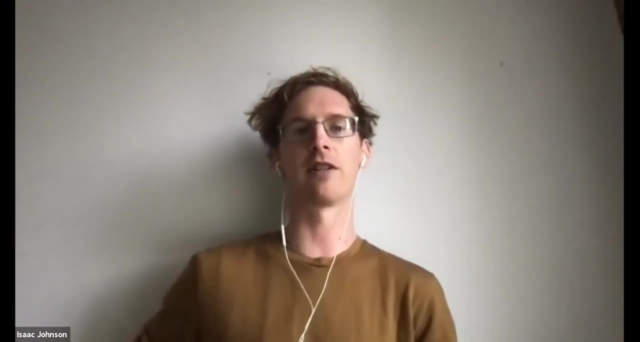 If you're a machine learning engineer, what sorts of languages are you? are you designing your natural language models to support? And, just broadly, whose problems are we prioritizing to support? In some ways, I think industry isn't super well-incentivized. 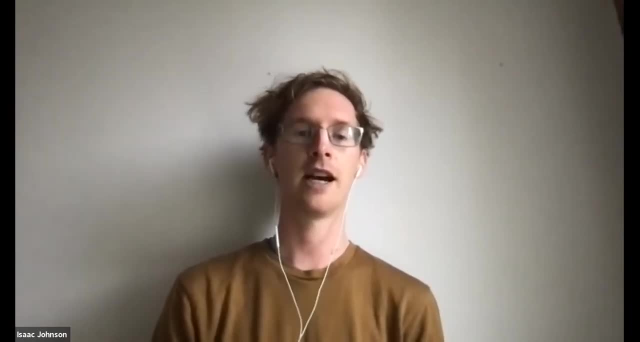 to do a lot of this work. Many of these language communities are small. There's not a huge amount of monetary return to some of these things And the work tends to be very slow. You're building up language resources that English has had. 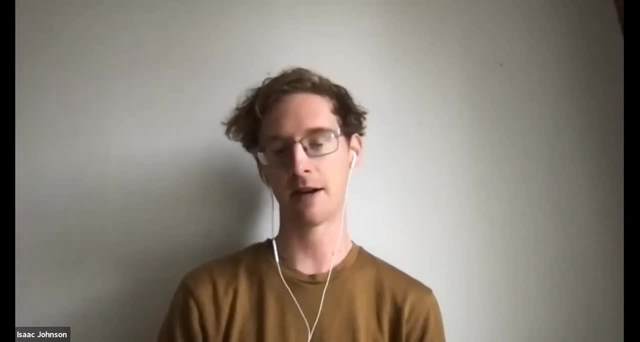 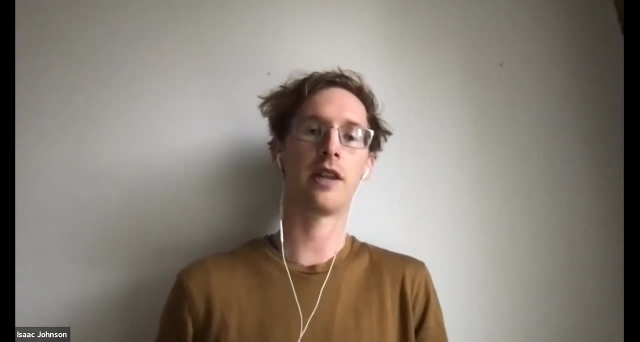 you know Years and years and years of building up online. So I think academia is actually in a really good position to be tackling some of these issues and pushing industry on them, And I don't think as far as skills. it touches on a lot of different areas. 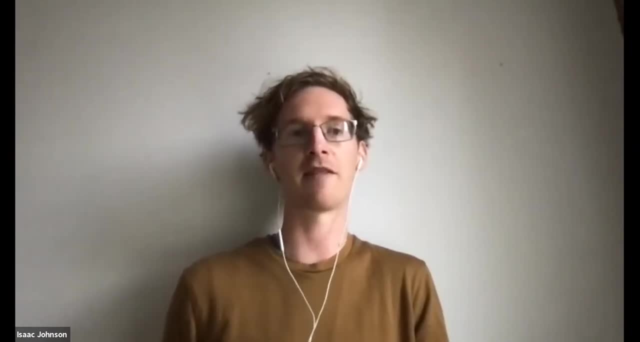 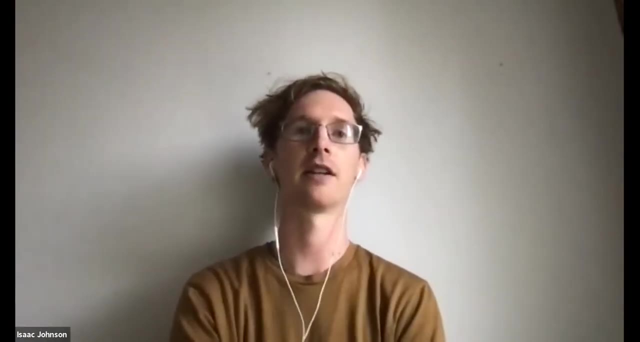 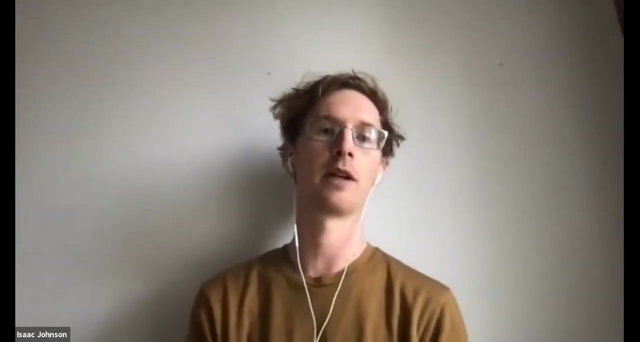 So I think the most important thing probably is having a diverse team of researchers that you're working with, so that you're thinking about these problems and have insight and connections in with other language communities. And I'll just say one last thing, which is I'm talking about language equity here. 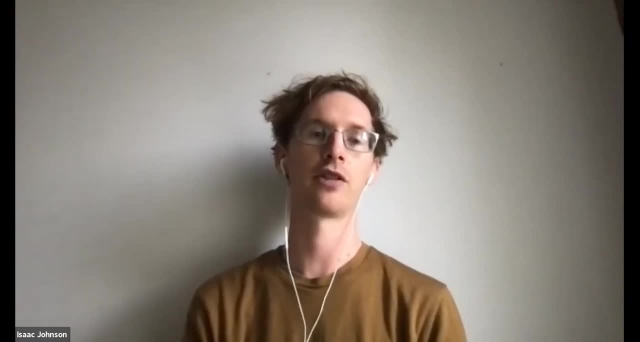 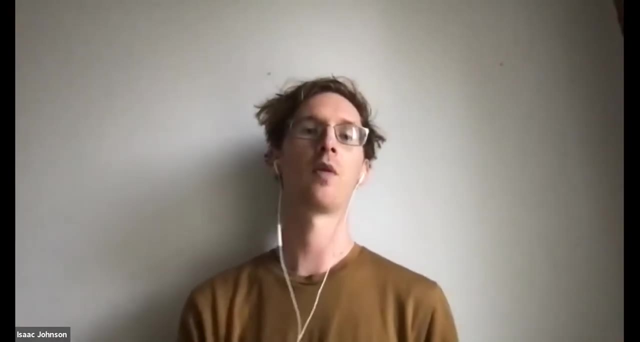 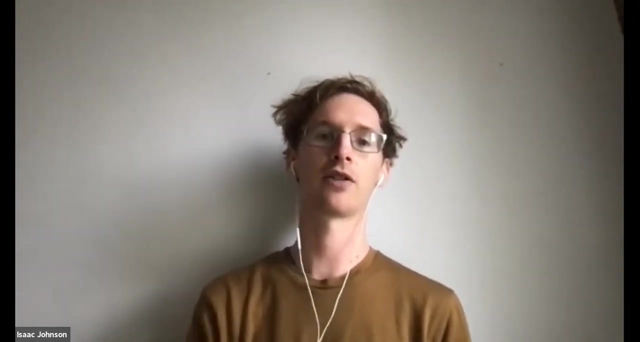 But I think more broadly, it's about building systems with constraints, So not just thinking what is the highest performing system we can build, but really thinking about what am I trying? you know, whether it's kind of language coverage or privacy or a lot of other things. thinking about what constraints? 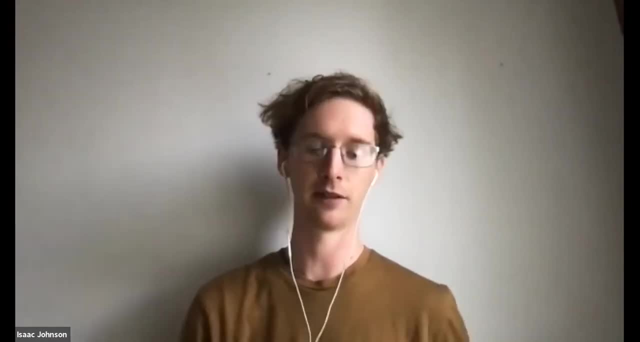 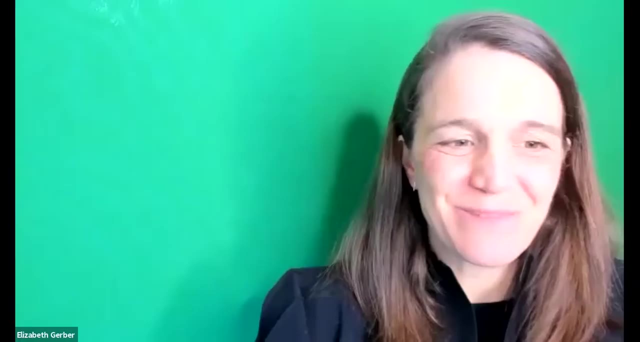 can I bring to this when I'm designing these systems. So I'll say thank you. Happy to talk, Obviously, much more about this, But I'll pass on to Emily now. Thanks so much, Isaac. It was great to give a little frame also of your organization. 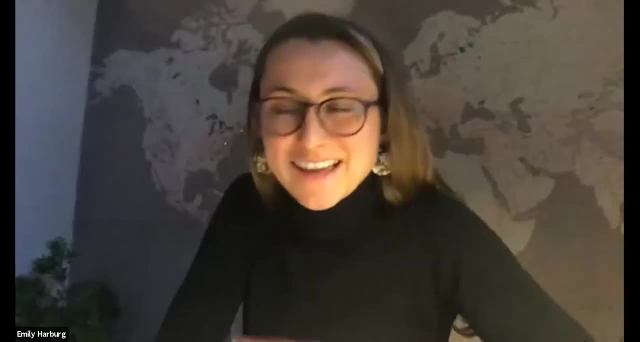 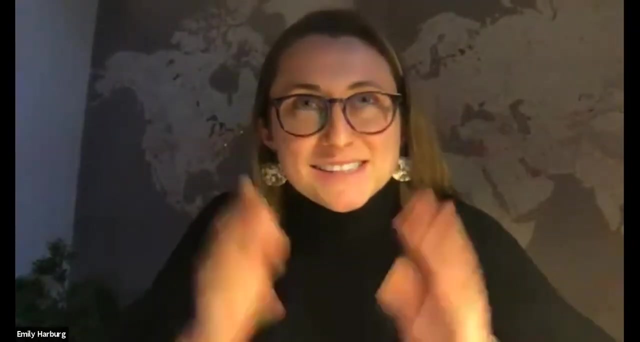 Thank you, Emily. Yeah, so I'm going to take us. I love both of those And I hope we can dig in a lot into both of those themes over the next hour. But I wanted to kind of take us into thinking a little bit. 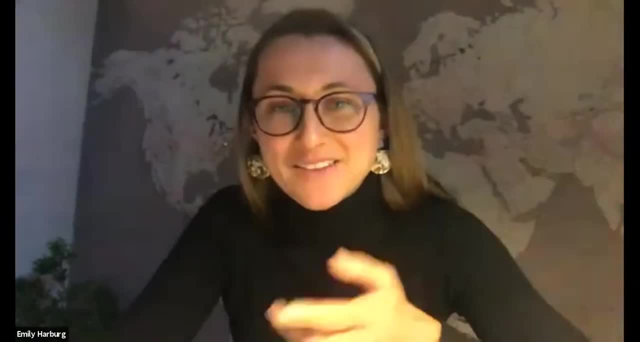 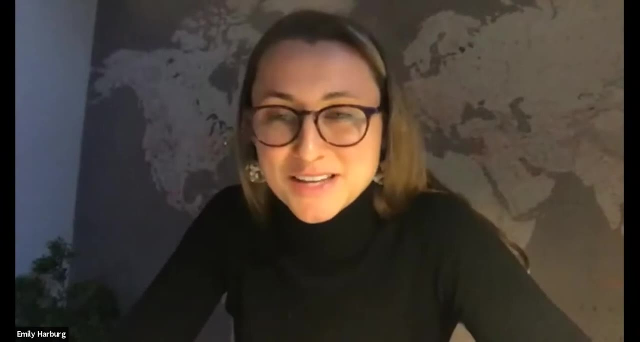 about tech in the world right now, And so I've been working at EF Education First for about three years now, And my background was also in working in tech and theme parks at Disney World. So I've done a lot of work, Kind of thinking about tech, interacting with experiences. 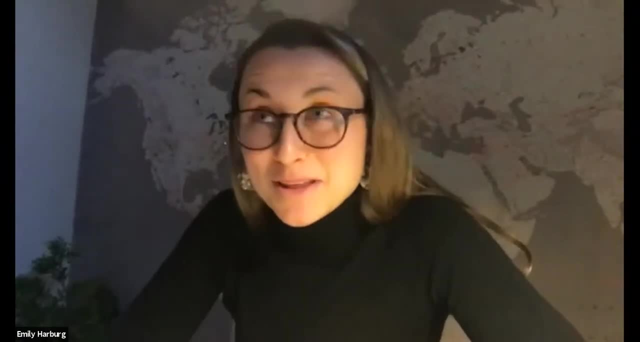 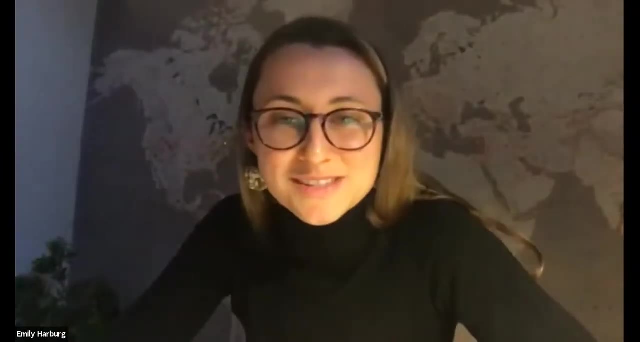 and kind of enhancing and augmenting those experiences. But to me, one of the big challenges that I've been thinking a lot about is how do we help people kind of use tech to look out and not down on their phones, And so I think this like we build for addiction. 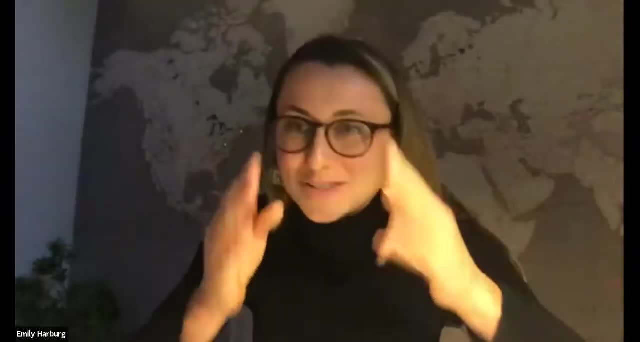 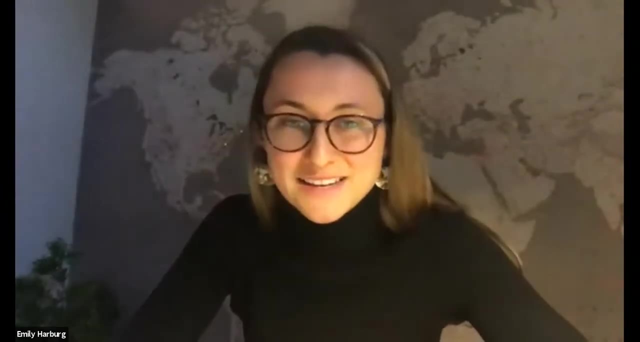 We build to kind of pull you in and keep you hooked and keep you in the tools that we're creating often. But I think the best technologies actually push us to connect and interact and engage and see things and with new eyes, And so I think that's been something as a team. 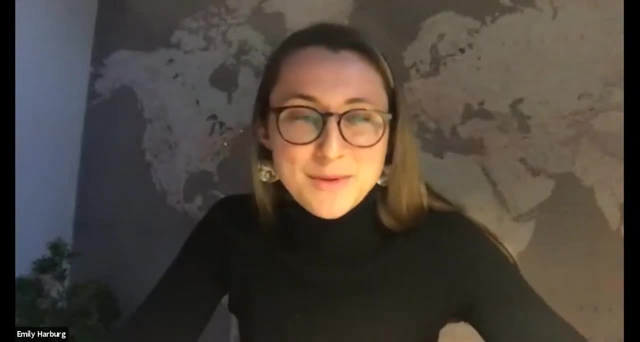 we've thought a lot about And all kinds of new technologies are kind of coming out to do that better, like glasses and different kinds of AR to help you interact and engage more effectively. But I also think where we build these chambers of that kind. 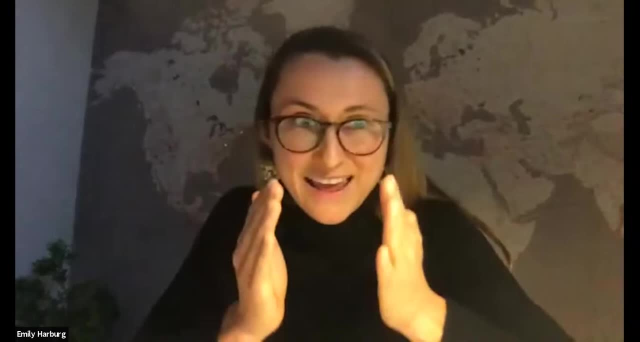 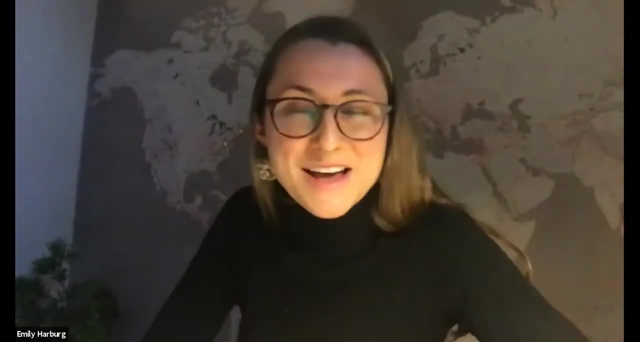 of force, especially youth, who it's kind of all they know to stay hooked on their phones, and older adults alike. So I think I'd love to dig into that a little bit today. And I think you know industry. I think you know industry. 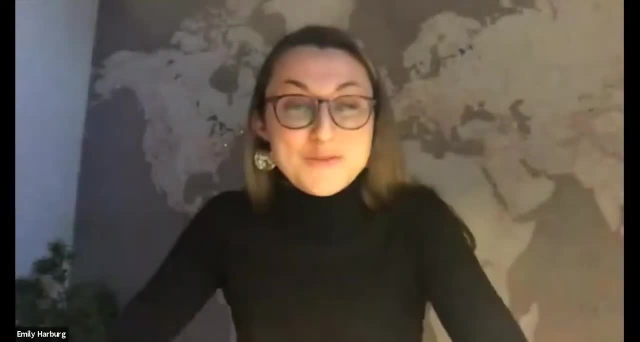 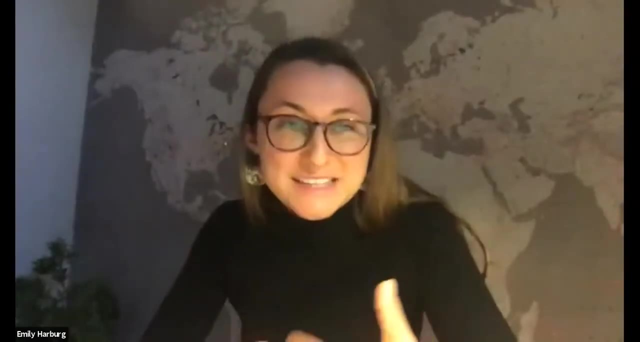 I think we are incentivized to keep you on your phone, And so I think that it's going to take some shifts to see. I think we are seeing people quitting tools because they find that they're too addictive or they find that they're taking them away from experiences. 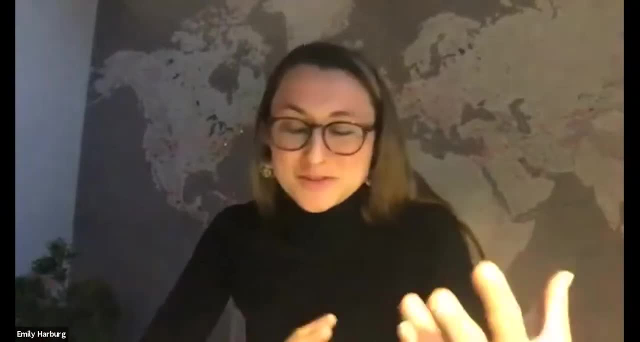 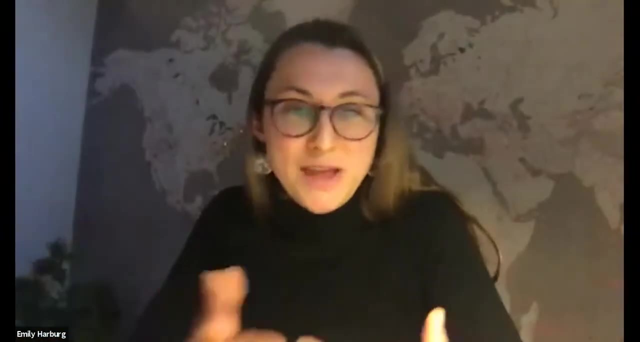 or making them more lonely. So I think we are seeing some customers kind of shake against that and especially parents who are concerned. But I think if industry can adjust and also take into account research around this, I think we'll be a lot better off. 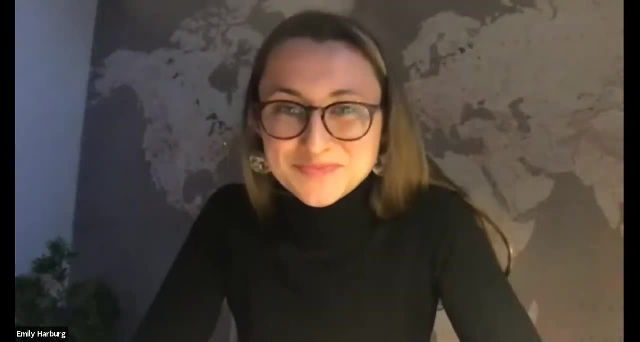 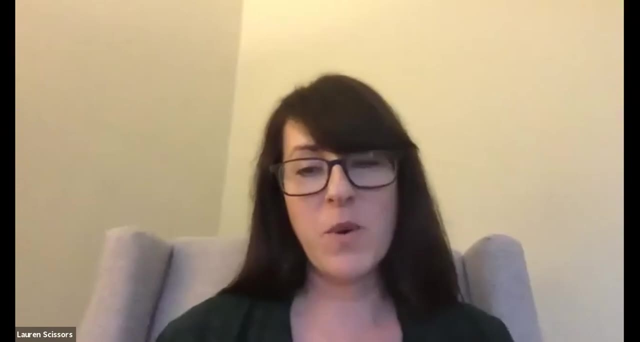 So, yeah, excited to dig into more of that tonight. Thanks so much, Emily. Appreciate that. Lauren, Hi everyone. So one of the things that I've been thinking about for a while is just how challenging it is to build features, products, apps. 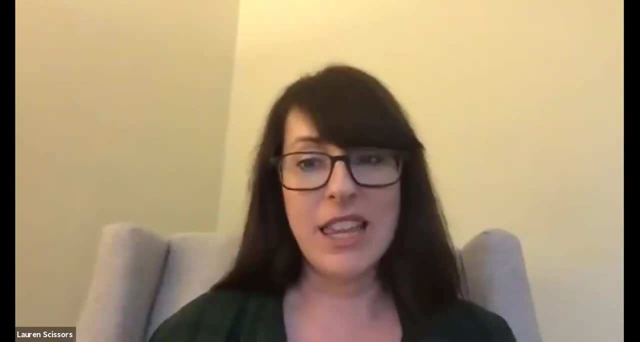 for the diversity of the world. I think that we all kind of know and learn that if you try to build something for everyone right out the gate, you probably won't build something very compelling. It might not serve an actual need But at the same time, when you narrow in, 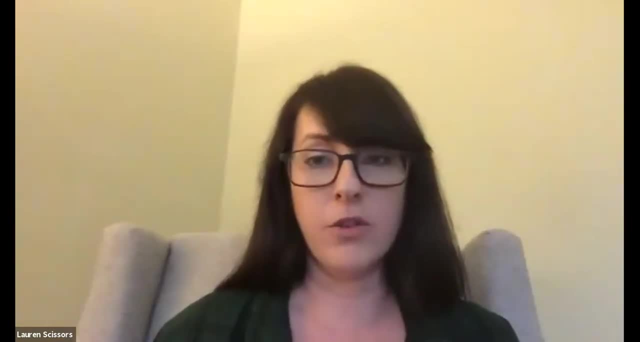 what populations or groups are you excluding? Are you hurting? And even if you don't intend for those groups to be using your feature, your product, your app, maybe in the future they will, because things evolve. And so when that happens or when you find yourself, 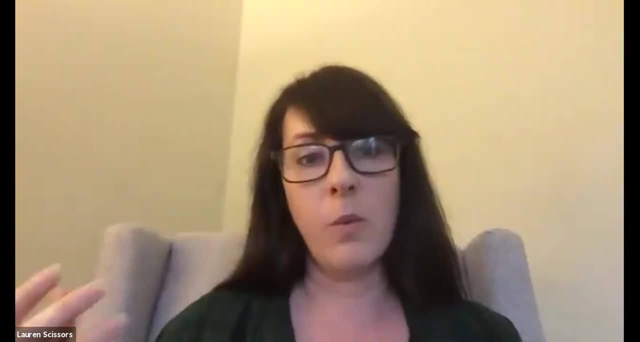 in that situation, how do you then look back and say, OK, what is a scalable way to ensure that all different types of populations or user groups are having positive, meaningful experiences with my feature, with my product, with my app? And I think scalable is really the thing there, because we 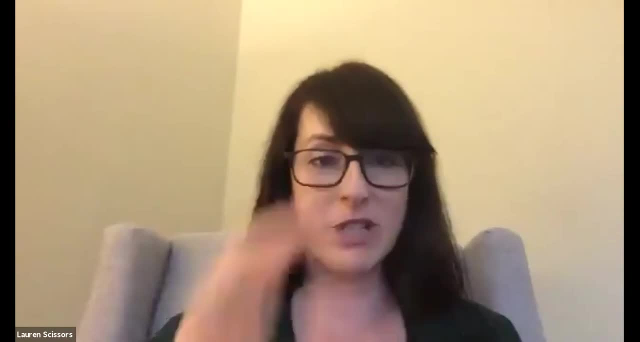 know that it's just impossible to think about every particular group of people and make sure all of their needs are served, But we can't just throw our hands up in the air and say, oh well, we'll just ignore that. So what are some systematic, scalable ways to think? 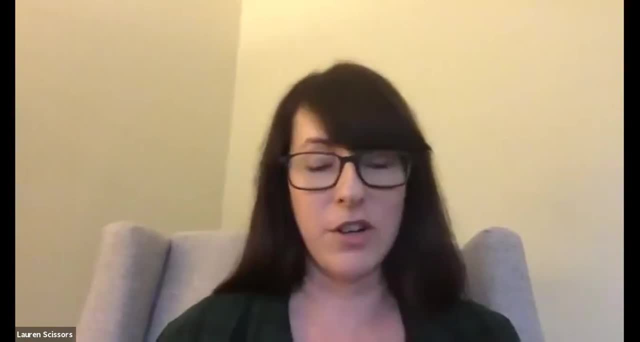 about different populations And how do we do that, And their use of your feature or your app, And so one of the things that's funny to me is I remember when I was in grad school writing CHI papers and writing the section Implications. 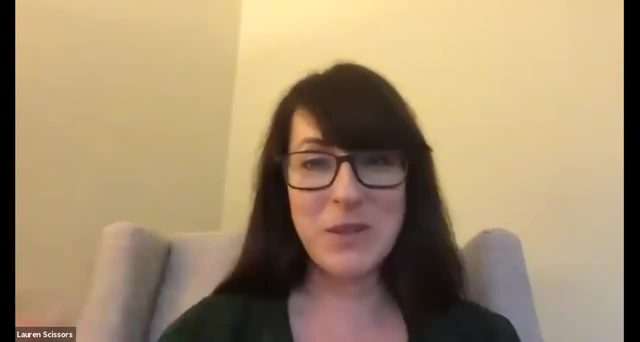 for Design. I'm not sure if it's still called that, but I would always do my best. But of course, I was coming from a place of not really knowing what it's like to be a designer, be a UX researcher in a company. 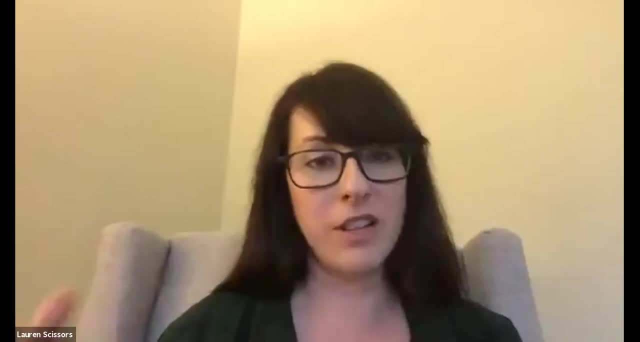 or in a, You know, non-academic environment and actually make those decisions And what are all the constraints that one is facing. And so I think the more that we can make sure that folks in academia understand what it's really like to sort of build products and what constraints folks 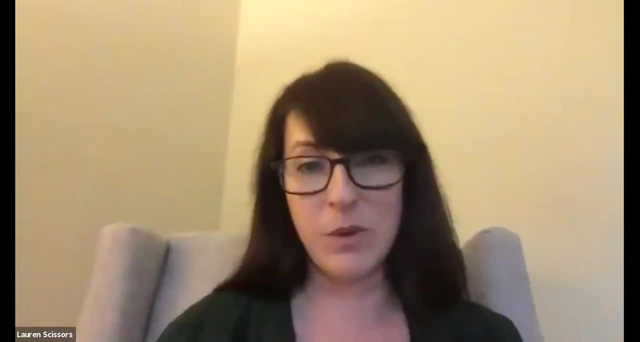 are under, I think the ideas and the recommendations will sort of be a lot stronger. And then, similarly, I think folks in industry can look at some of the information and recommendations coming out of academic research And even if it doesn't fit their mold, 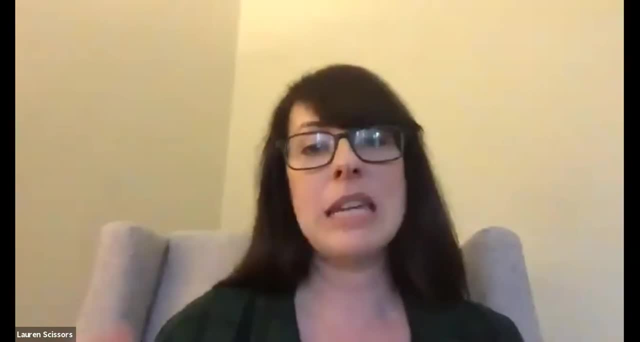 they can look at some of the information and recommendations coming out of academic research And, even if it doesn't fit their mold right away, to say, OK, but there's something here, There's a spark here, There's an idea here. 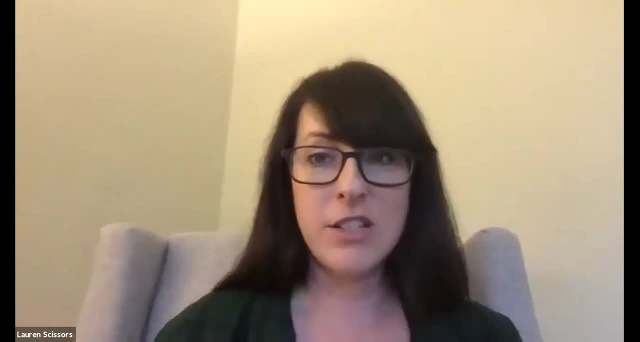 And how can we expand our mind or our processes to do a little bit better or to try things in a new way that will kind of help us better serve a range of populations or user groups. So it's high level, but that's quite on my mind. 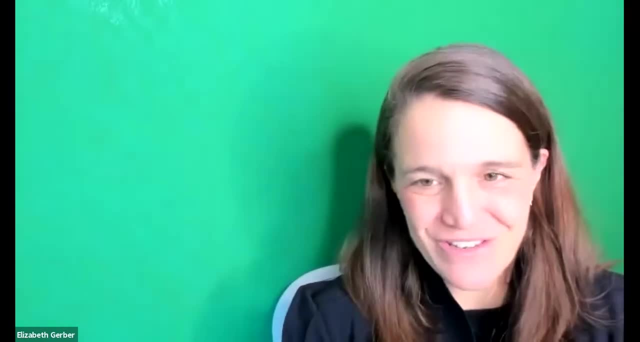 Thanks so much, Lauren. I'm so glad you connected it to design implications and writing papers. So thank you very much. We're going to hear from Prem in just a moment, but I want to remind you that we're going to be talking about some of the things that we're going to be. 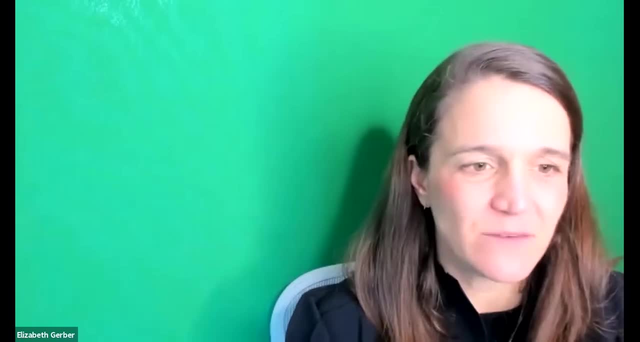 talking about in the next few minutes. So I want to remind everybody that please feel free to put questions in the Q&A box And we have a team that's monitoring them and we'll aim to get through the questions we can. And Prem from you. 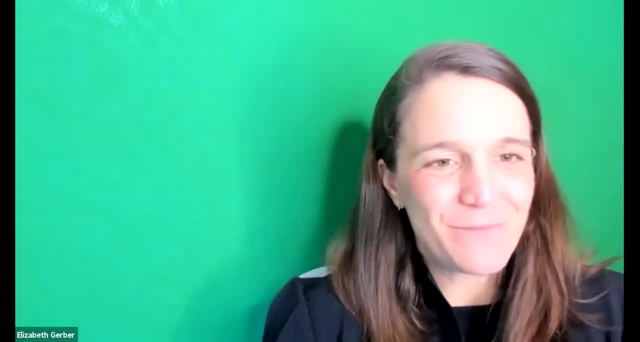 Hi everybody. I mean thanks for having me. My sort of the thing that's always on my mind where I work at Descript, and before this in grad school, was that like content creation is like a very difficult thing for a lot of people, I think. 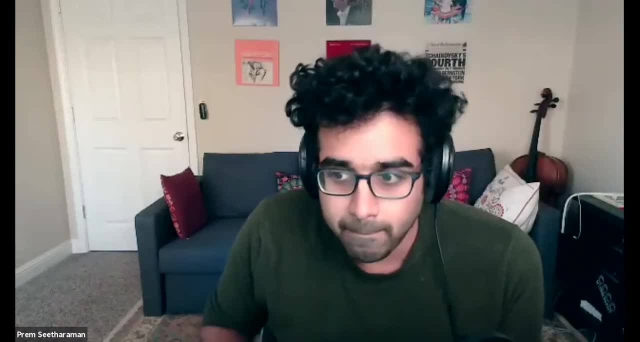 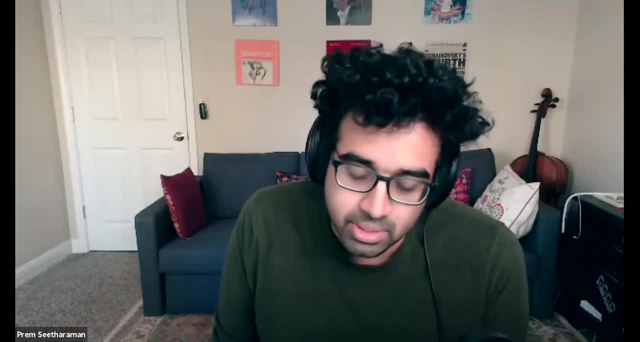 I think that's the right word for it. But if you're local, you're just starting out here, you're just starting out at home, you're starting out at school. I think that should be a big thing, But yeah, I think the thing that's always on my mind. 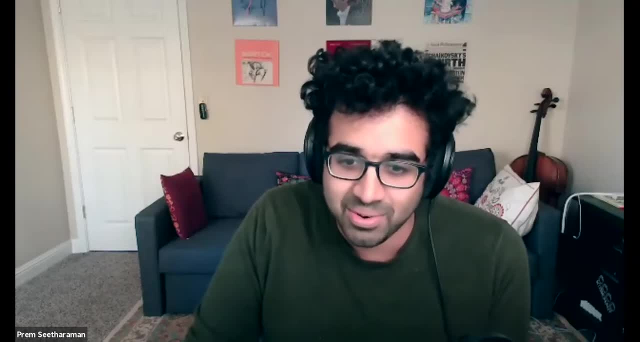 where I work at Descript, and before this in grad school, was that like content creation is like a very difficult thing for a lot of people? I think, Right, Like people have a lot of difficulty creating videos. 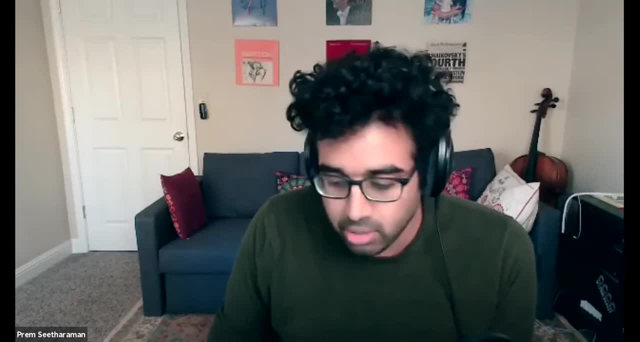 creating music, creating any sort of- you know- audio-based, like a podcast and things like that, Right, And when there are a lot of barriers to this process, what ends up happening is that a lot of creators just fall out of the pipeline entirely. 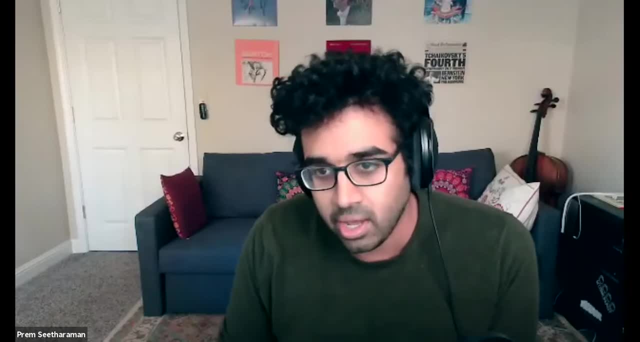 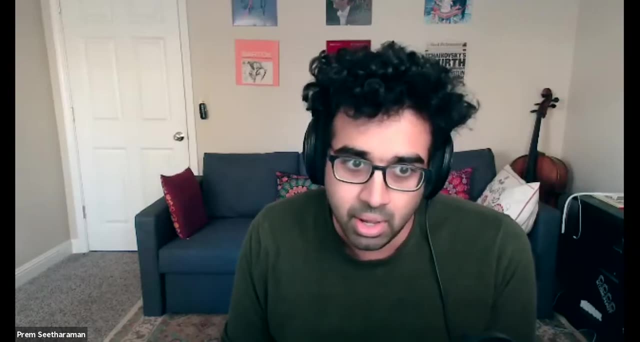 Right, there are a lot of barriers to this process. what ends up happening is that a lot of creators just fall out of the pipeline entirely. right, there are people that whose voices are like not being heard, um, whose voice things are not taking off, like on, you know, on twitter, or tick tock or whatever. 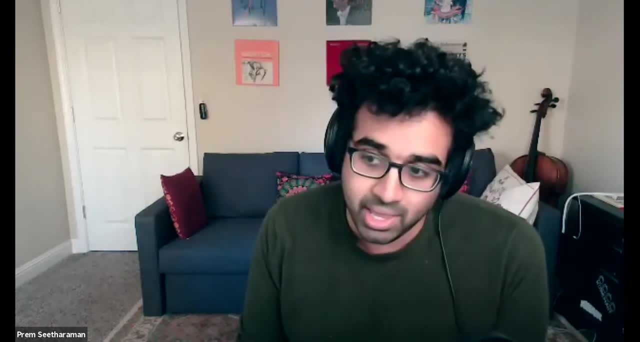 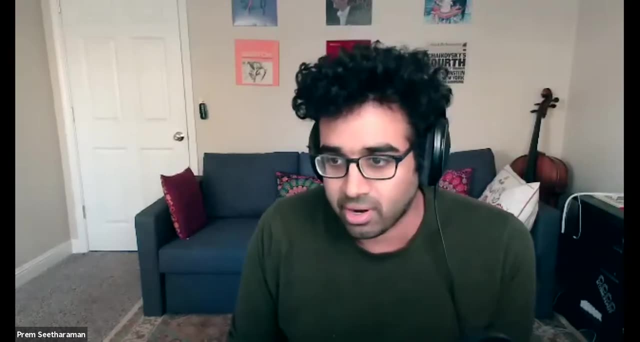 uh, that people are using, like um, because the way that they're making their content isn't great, right, they're running into all these stupid little things that really they stumble over and they end up with this pretty bad end product. right, even if their messages could, you know, they might still. 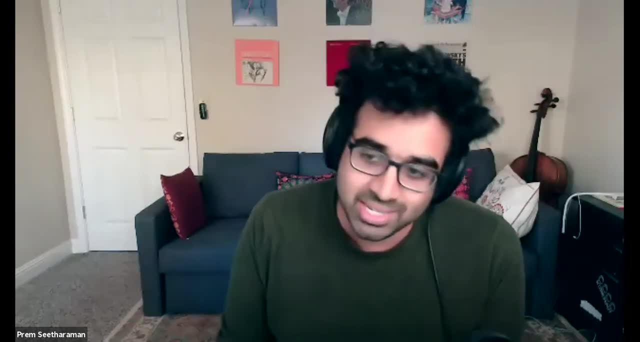 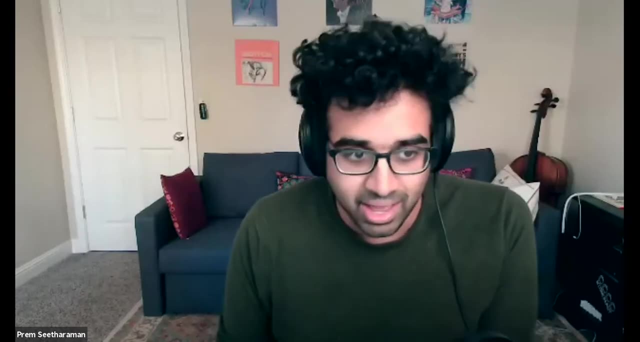 have a lot of room tone in the background or reverb on their voice and people listen to them like, oh, this doesn't sound like professional, right, this probably isn't worth my time. like people you know, subconsciously or consciously think that when they listen to a lot of um content. so 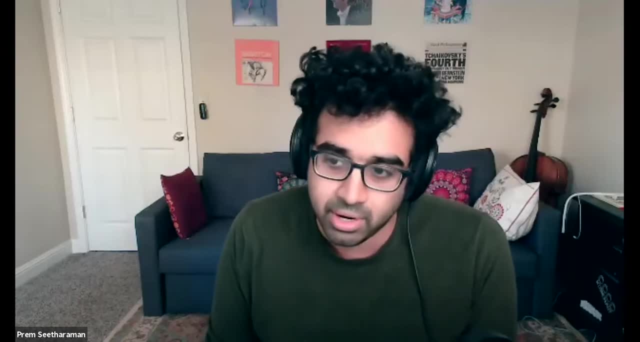 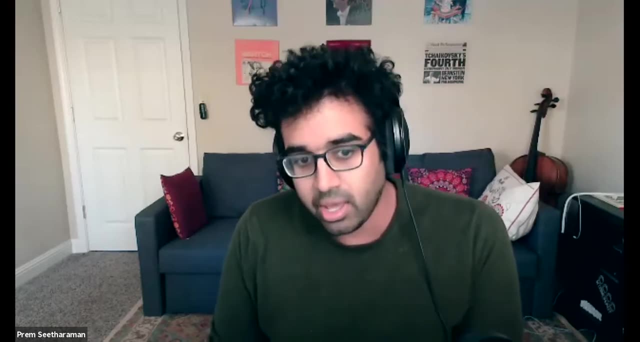 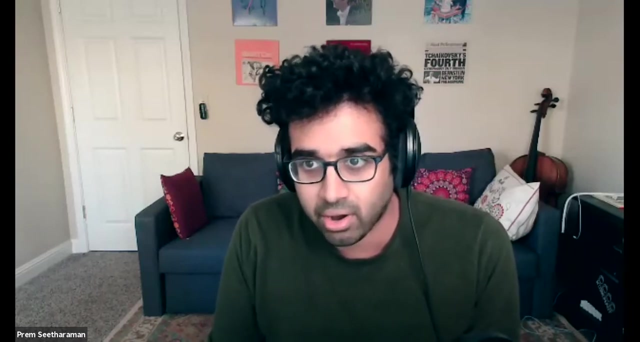 a descript, um, and in my grad school and all my work has been sort of geared towards lowering that barrier to entry and, uh, retaining people in the creation pipeline as much as possible. and the way that you know we've always tackled the problem is by identifying little frictions that can occur. 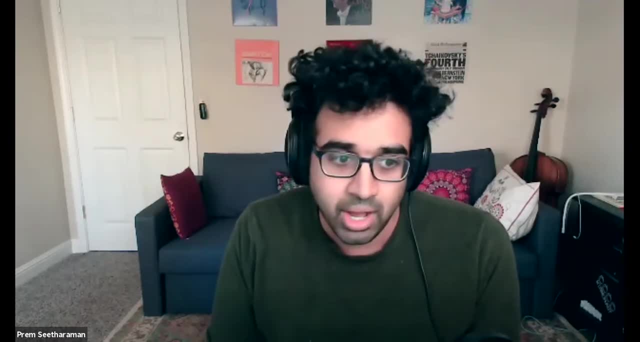 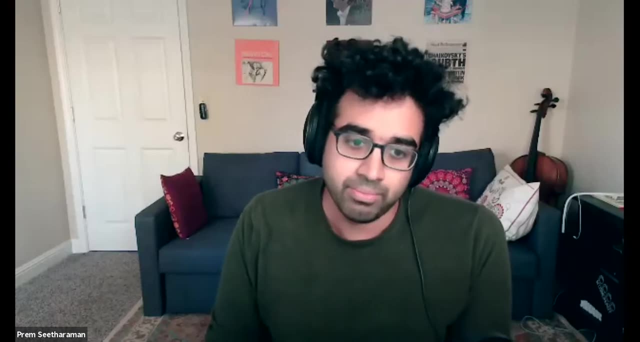 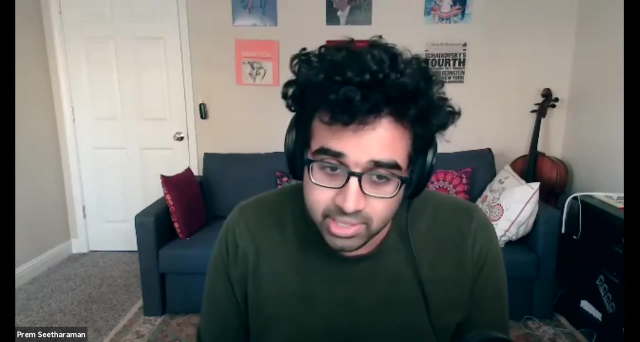 um by you know, observing user flow and stuff like that. like um, making edits, like deleting you know words in someone's audio, like um figuring out like, oh, this is a bad take, this is a good take, all these like little things, right, um, that people need to do, or making good recordings and stuff. 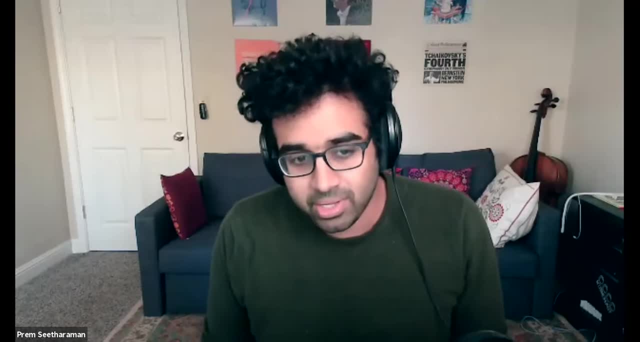 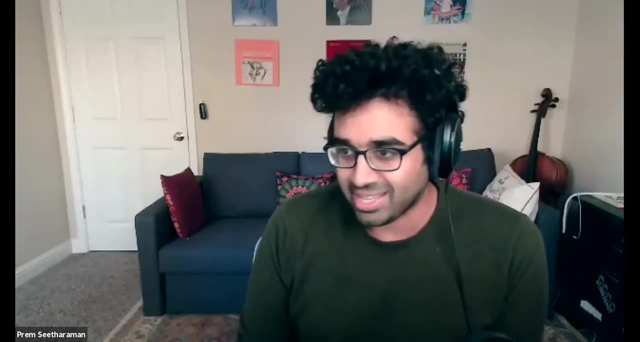 like that right. so we just identify all these frictions and our main goal is to like make it really like um, easy to create content. i'm sure a lot of people in the audience last year have had to make videos for like conference talks in the last year and i'm sure it sucked like i'm sure. 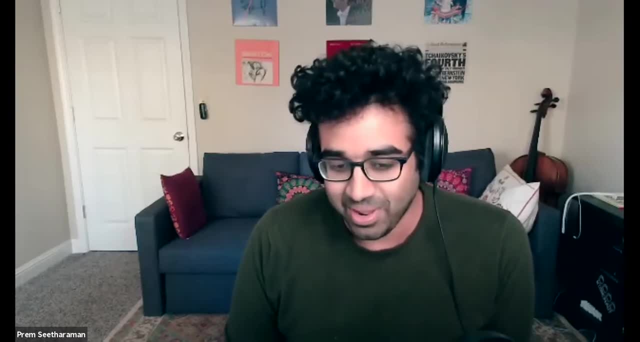 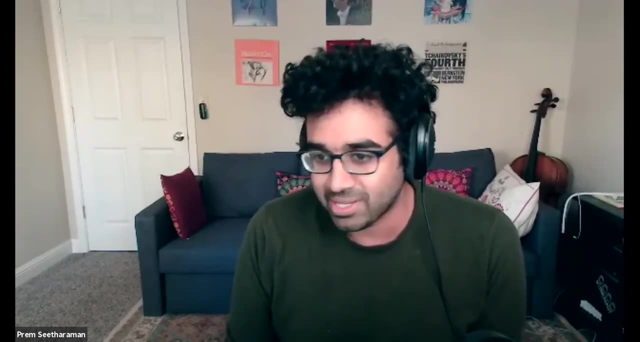 it was just really hard to do, um, and you know even little things like how loud should the music be. when i'm like talking, right, some people mix it at equal volume because it's their first time making anything and you can't understand what anybody's saying. right, it's like these, all these tiny things. add up and really make it a very difficult thing, right? do you know what i'm saying? like i'm like i'm doing it, but i think it doesn't make sense. and i think, like i'm just, i'm just saying like it's like all these tiny things add up, um, and really make it a very difficult thing, and i think it has to be made. 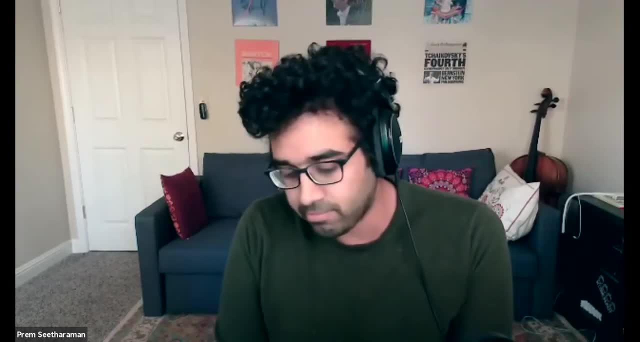 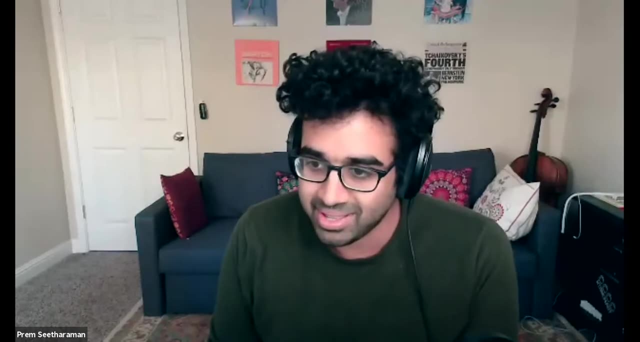 some people are usually really slow to make videos, because the video is a very good way to just like listen to it. a very difficult process, so that's kind of you know, that's been like the, the main like through line of my work for the past like 10 years or whatever at this point and uh, yeah, i'm just hoping. 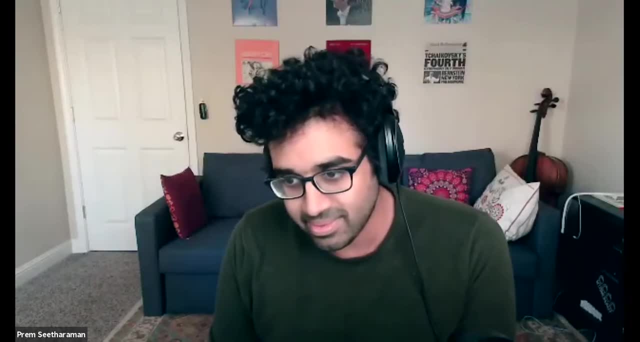 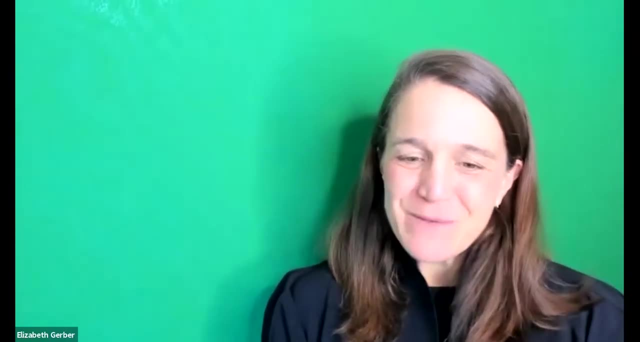 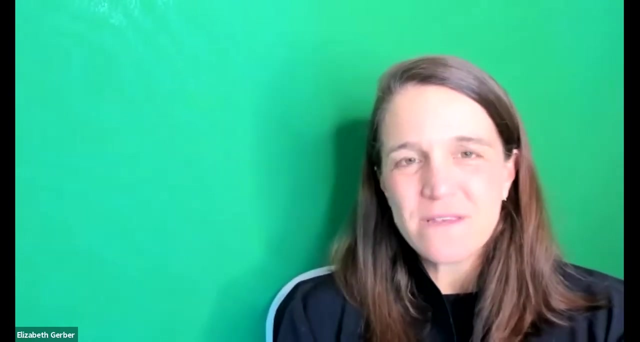 to continue on that. thank you so much. i'm so struck by the, the diversity of industry. uh, representation here is really wonderful. um and makes me want to ask um, given that you're all experts at these particular grand challenges, um, can you reveal for us what some of the biggest or most common 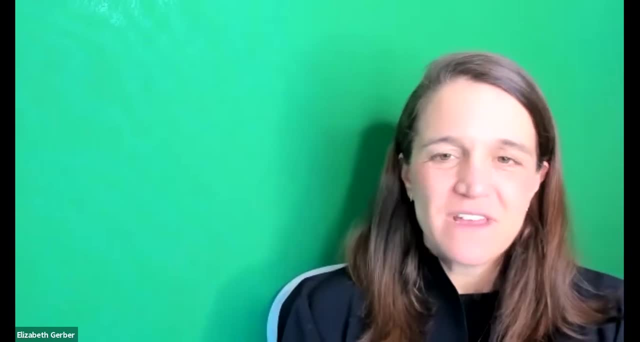 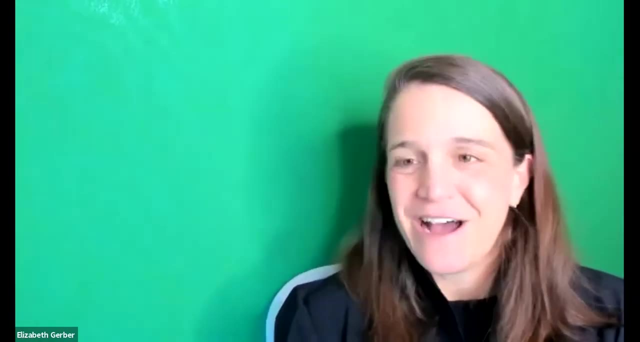 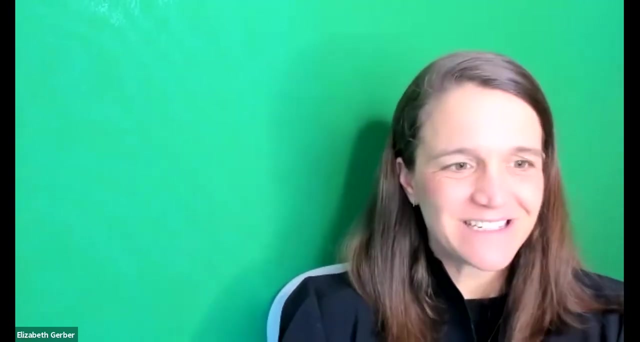 misperceptions about some of these grand challenges are: what are things everybody thinks they know about um broadening participation? what are things people think they know about scaling um that really aren't quite true. based on your position from industry, would anybody like to take that, or do we know everything? 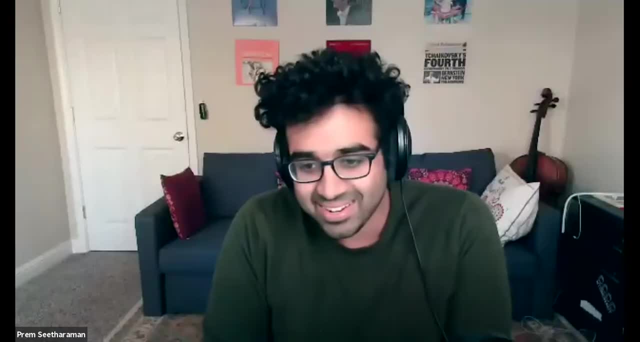 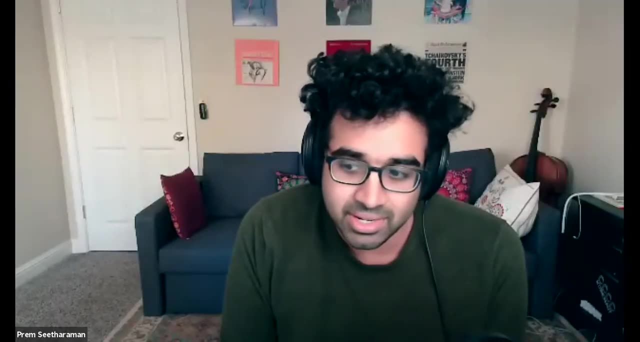 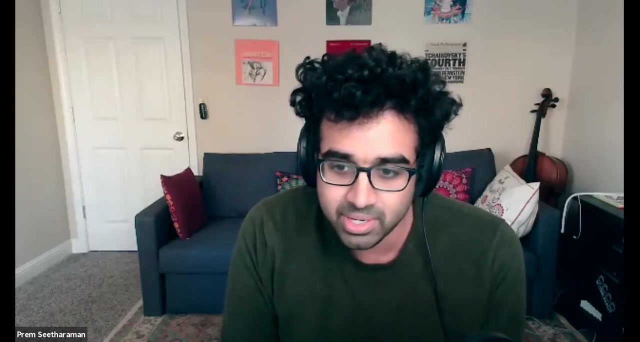 uh, i can, i can really quickly. i mean, i think one thing that um struck me coming from academia into industry is that, uh, i came into industry with a very like blue sky sort of mindset towards research where i really wanted to solve problems that i you know that industry actually simply isn't. 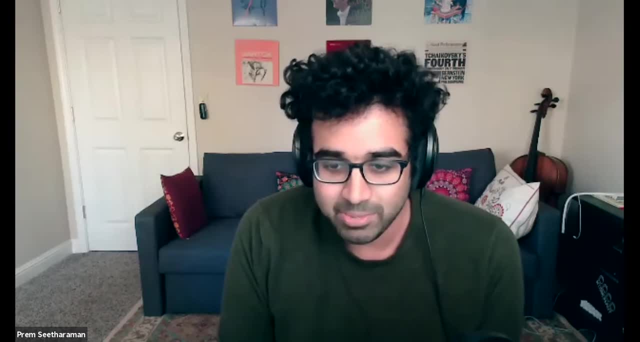 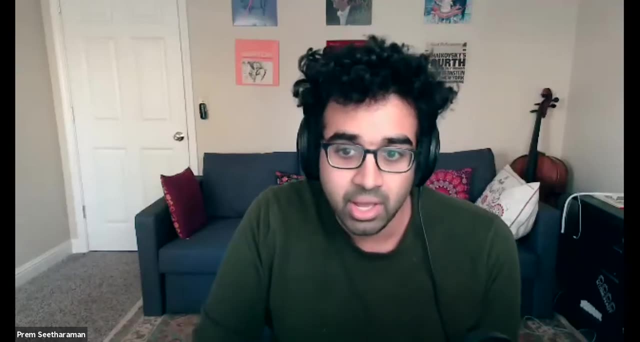 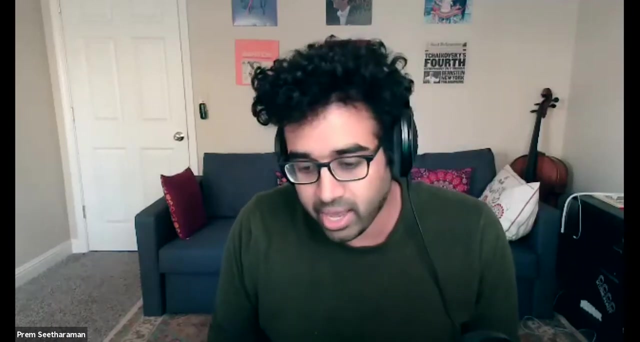 incentivized for like at all right, like especially at a startup, for example, like the pace of research is like much more geared towards like product and like solving, um, like some little problems versus big problems, and i i would say the one thing that really helped a lot in changing my mindset was that like little problems add up to like a big. 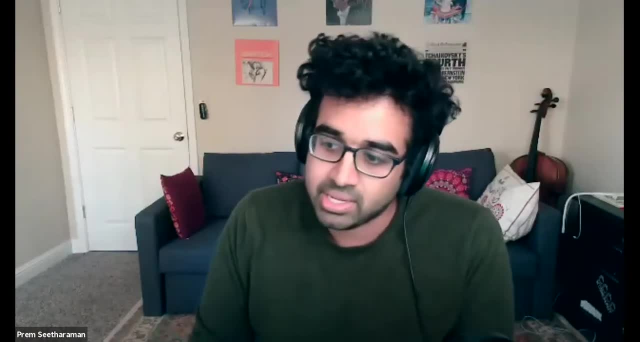 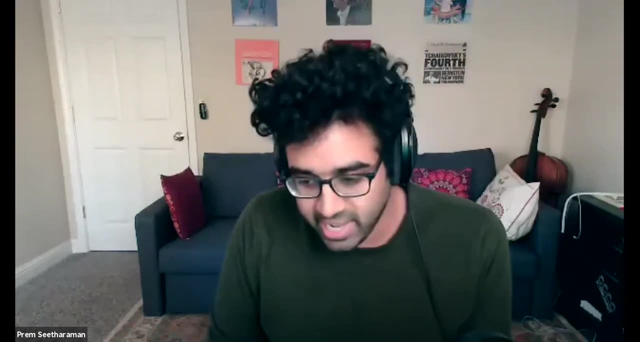 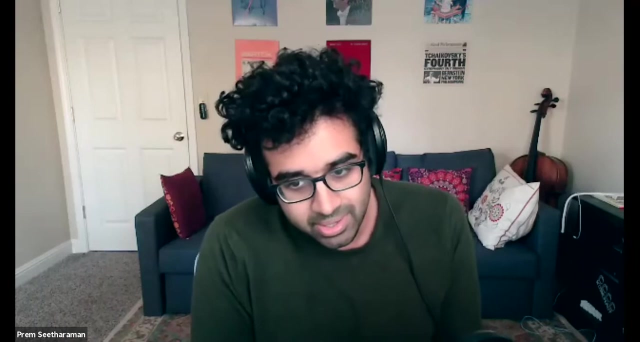 result right, and like breaking it down to that thing is like super, um, important, i guess in a lot of ways like uh, just to be able to tackle things in that way instead. so that's one one misconception that i had coming into industry from academia. uh, a lot of ways. 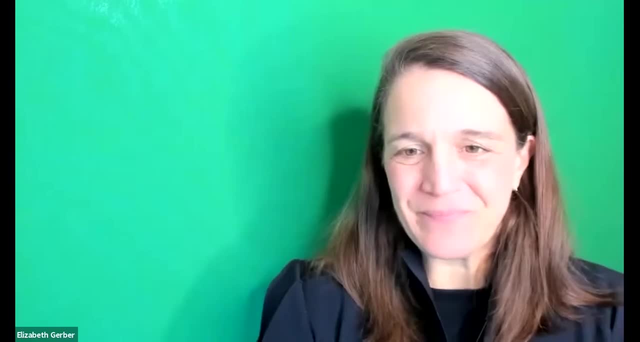 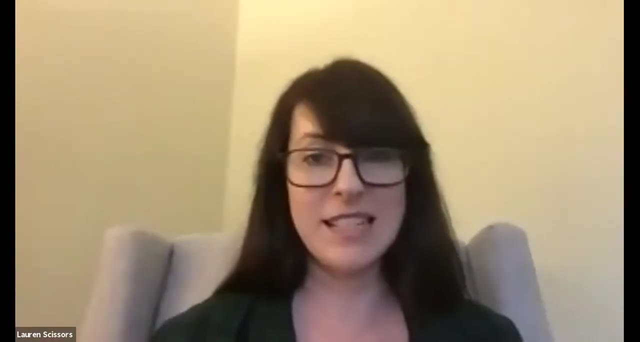 thanks, bram. yeah, i think, um, you know one of the things: it's hard to really know how products get designed, how products get built, until you actually are are in the thick of it. um, so for me, uh, it was really interesting to see all the ins and outs and how decisions get made, what the constraints are. 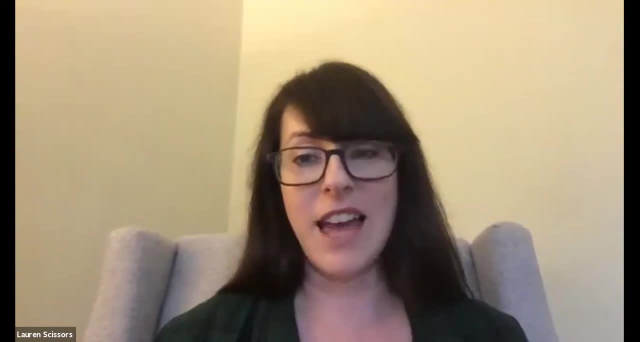 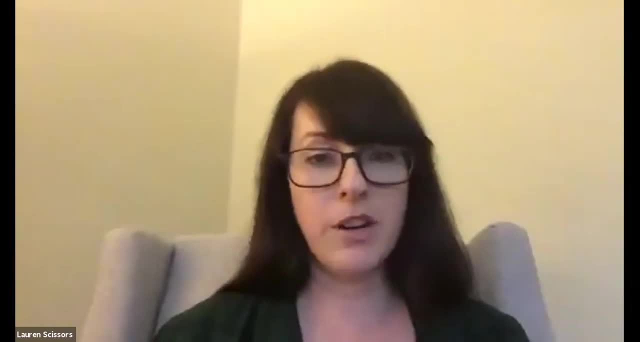 things that we do try to do is, uh, at least in my experiences- we always want to know the, the best knowledge that there is. we're always seeking to, to be informed um, when we make decisions, when we go one direction or another direction. you know, ux research does a lot with that- um, data science. 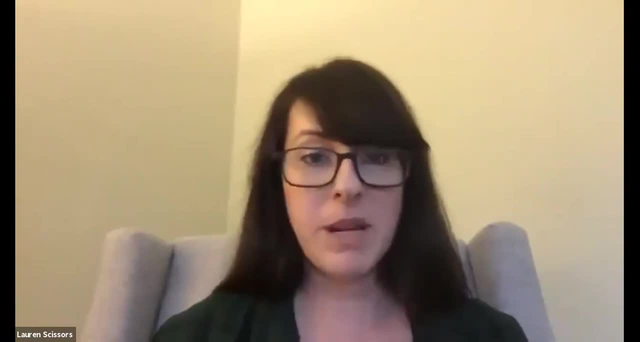 can, can support that quite a bit. um, but sometimes, you know, we we do want to engage with academics who really have spent, you know, decades uh in certain areas and they are uh going to provide more knowledge than than anyone in a particular industry setting might be able to. when 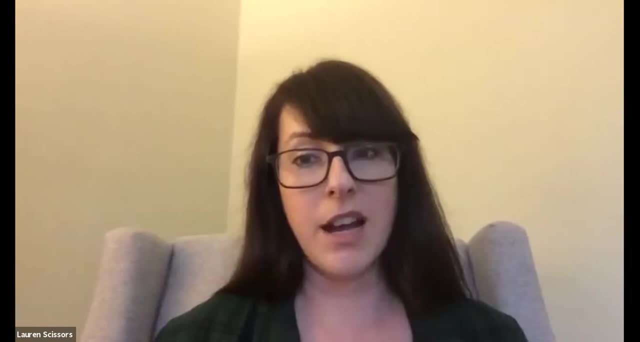 they're coming to a problem, you know, uh, for the first time and so, uh, it's been really exciting for me over my career to have like really, uh, highly esteemed folks from academia come in and actually work with us day to day and, you know, share their 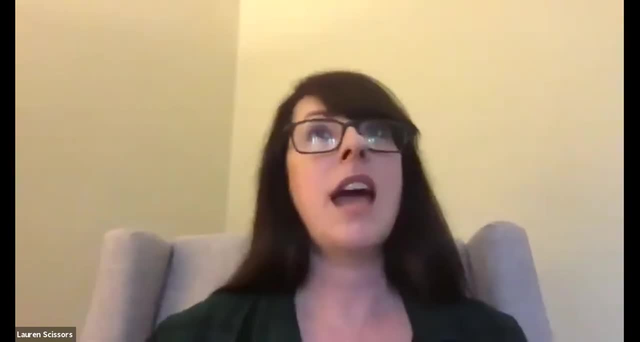 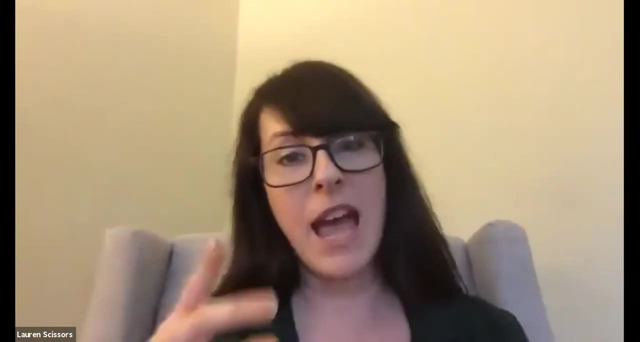 perspective, but also have them see how we do things and then reflect back: oh, this makes sense. oh, i never thought about that. oh, have you thought about doing it this way? and it feels really like a nice exchange, you know, where we kind of have the same goal: we want to build good products for. 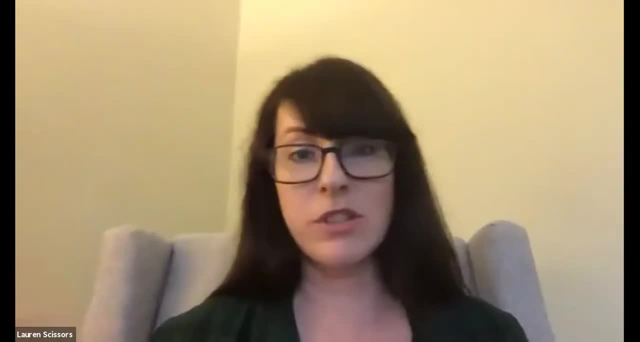 people. um, you know we want to make good choices and we're just learning from each other, you know, about how to do things and and evolving our practices on both sides, so that's been really cool. um, and we've had a few academics come on my team, you know, spend the summer, spend half a year, and and those relationships have been really 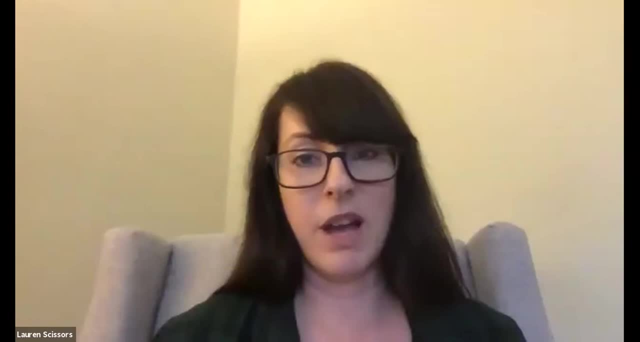 rewarding. um, the other thing we've done in the past is we've held, uh like workshops or summits where we bring in folks from academia to you know, discuss or tackle a big problem that you know we're we're working on or we're caring about, and those have been really rewarding you. 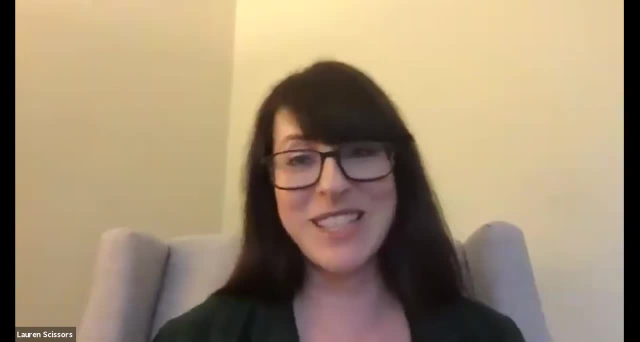 know true, true research forum. we always do little surveys afterwards like: how did you, how did you find this workshop? and you know, it seems like people get a lot out of it, both the folks in industry and the folks in the industry, and the folks in the industry and the folks in the industry. 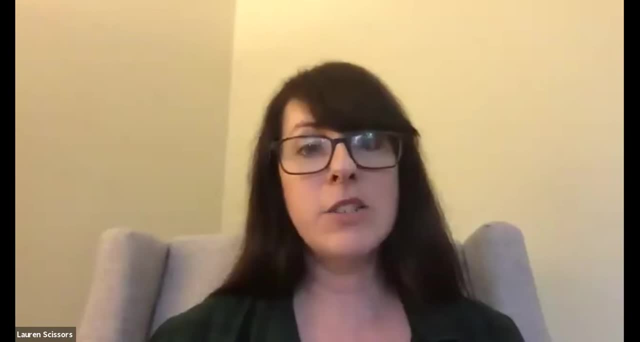 and the folks in academia. again, i think like it's, unless you're really talking to someone who's living it day to day, it's hard to really understand. and if you have that understanding, it's going to make your recommendations, i think, stronger and more likely to be, you know, taken. 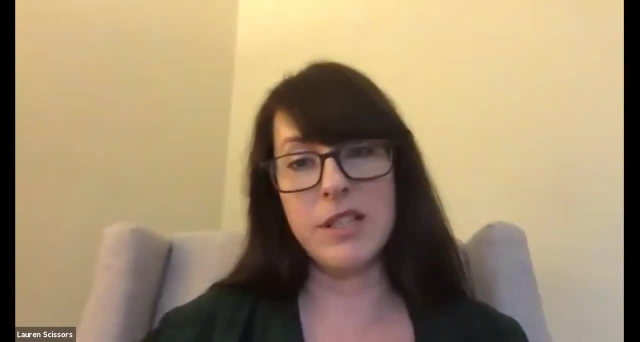 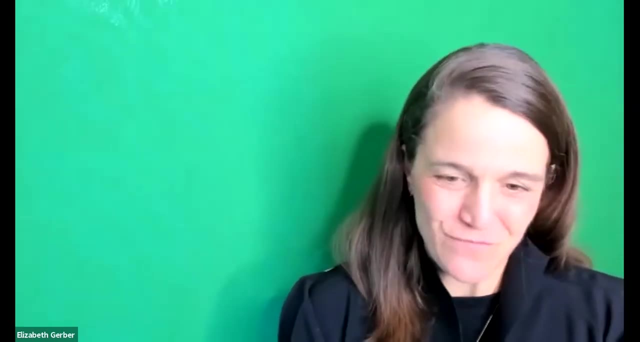 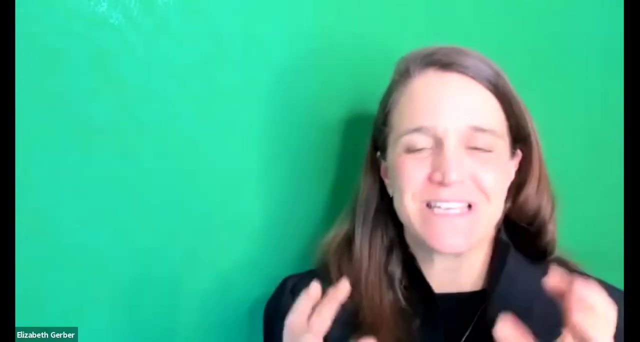 into account and adopted. so that's just a couple of experiences i've had that i feel have been really good. that's great. i appreciate this. uh, specifics you've offered there. um, so, bill, building on, building on some of these conversations and maybe getting a little more into some specific case studies or examples, to the extent to which you can share them, um, i'd. 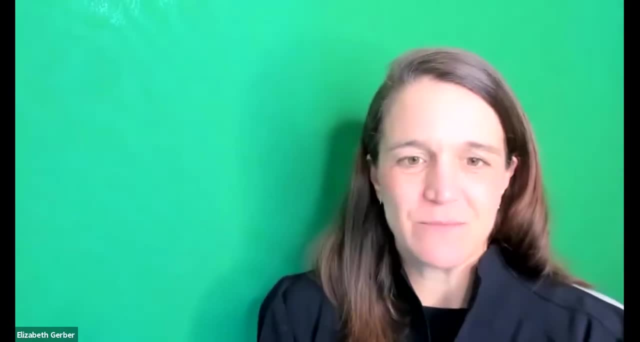 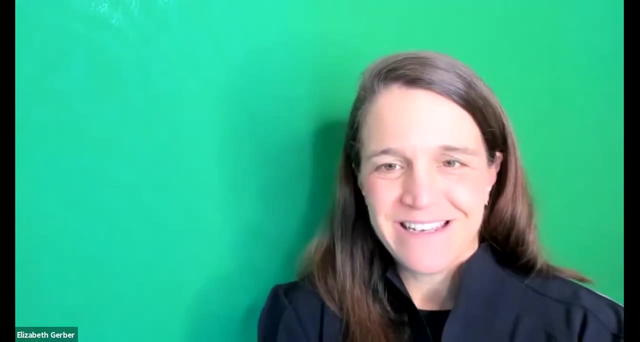 love to hear some success cases of what are things that you've been able to do, that have really been able to tackle concretely, um some of these grand challenges that you're that you're facing, and with as much detail as you possibly can, so we can really have an understanding of. 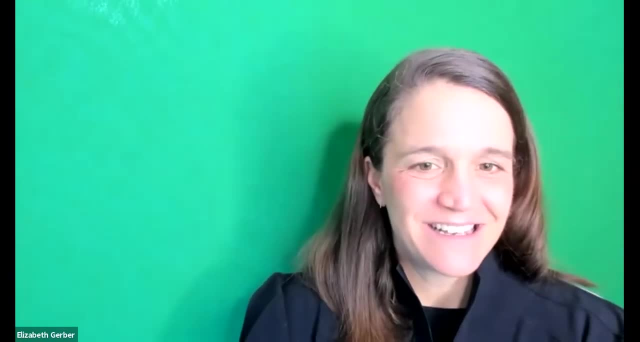 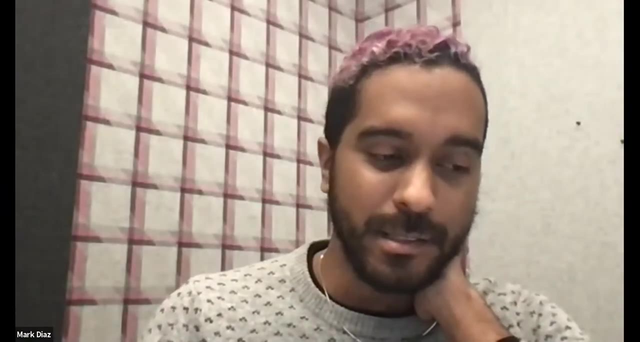 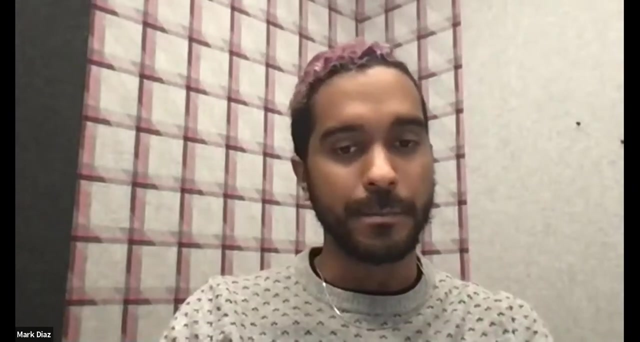 what you're doing day to day to tackle this mark. can i call on you? yeah, i was just thinking about this at different like scales, so um one of the so thinking about, i guess, the problem i mentioned earlier around participation, um one of the things i've been 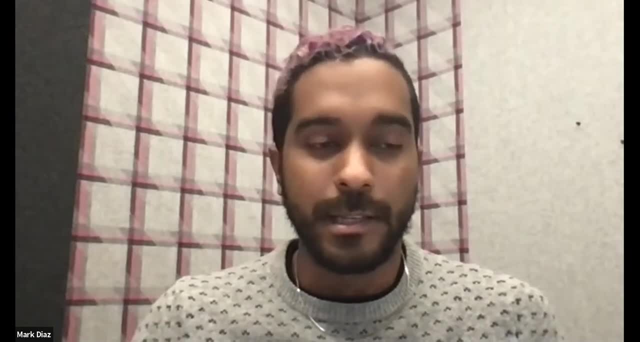 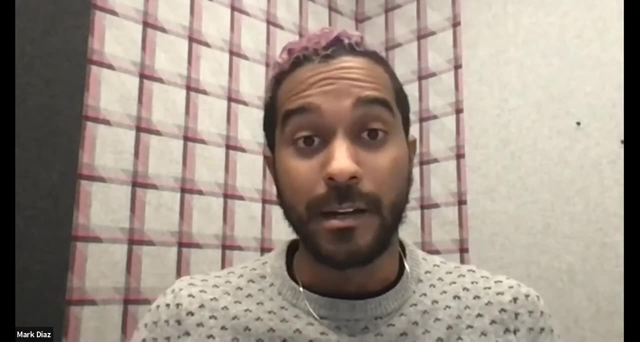 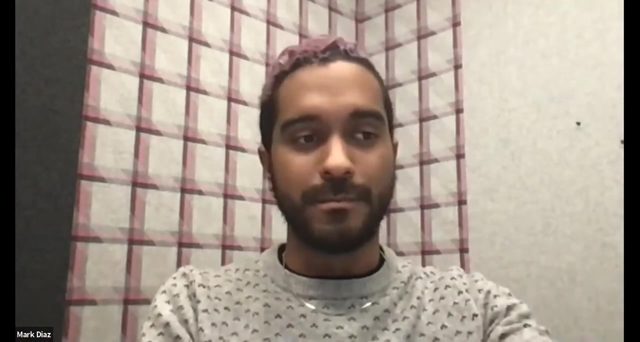 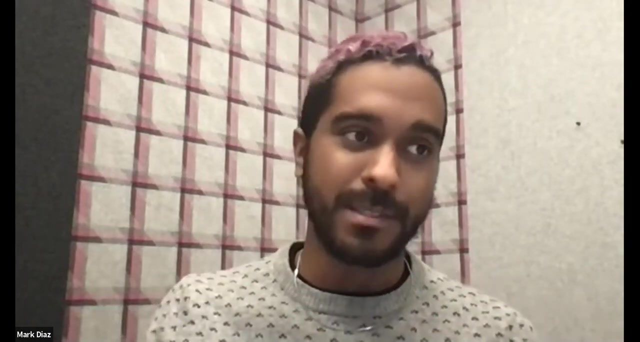 really uh, excited about is um, an intern project we just had this past summer that involved community-based work in chicago. um, and the structure of the the project might be familiar to some researchers in academia, where we are running community-based workshops with community-based partners, um, who are themselves community leaders, and 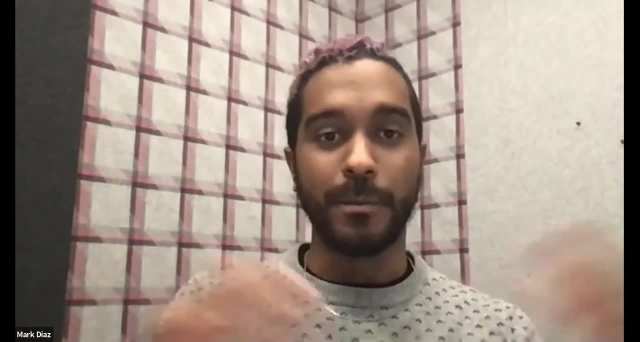 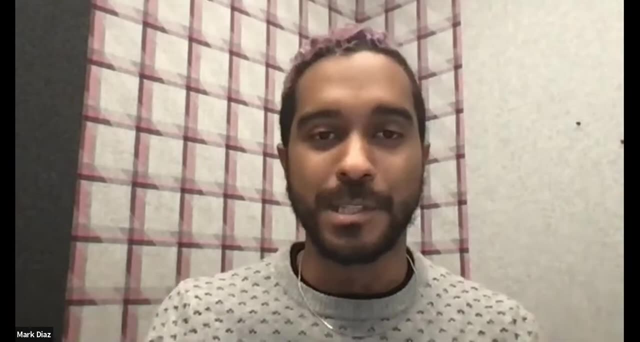 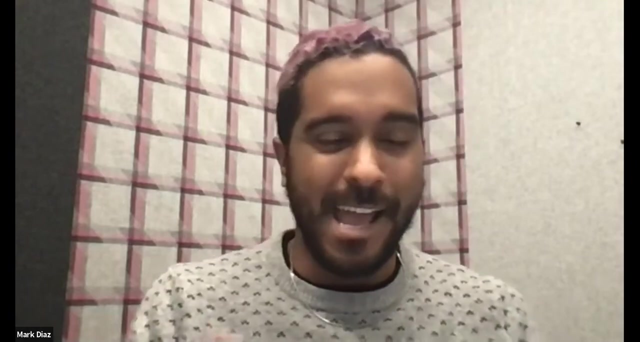 we are co-authoring with community members, um, who are participating in the workshops, and that's just something that doesn't happen in industry. i'm also in a weird position where, like i, my day-to-day is basically that of an academic and i have the privilege to like sit at a company and sort of have insight into how. 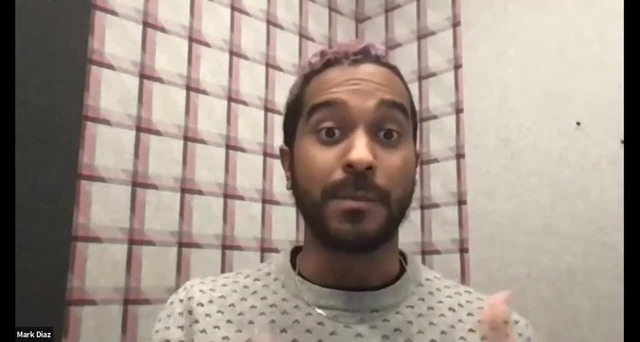 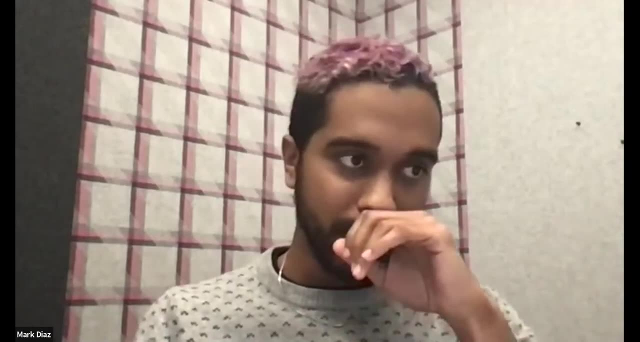 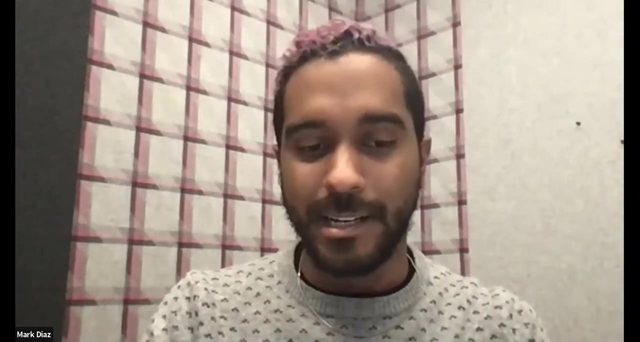 all the internal processes are happening, um, so i'm not working on a specific product, but, um, i was really excited to see this work which is also being done with uh researchers, actually sheena arete, so depaul, and, um, uh, christina harrington as well, who a lot of you may know. 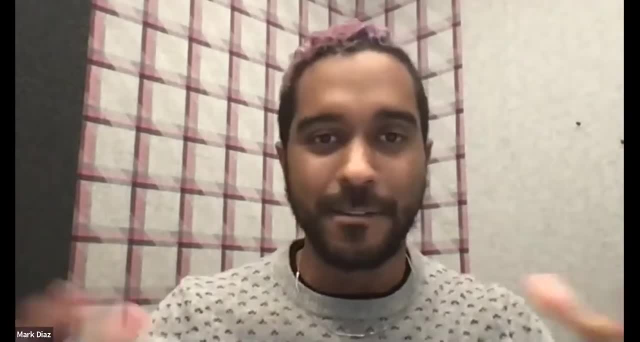 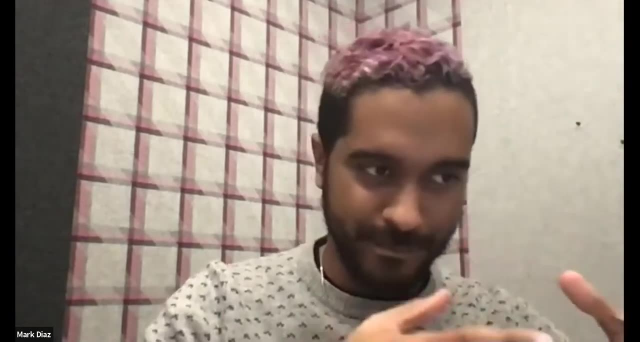 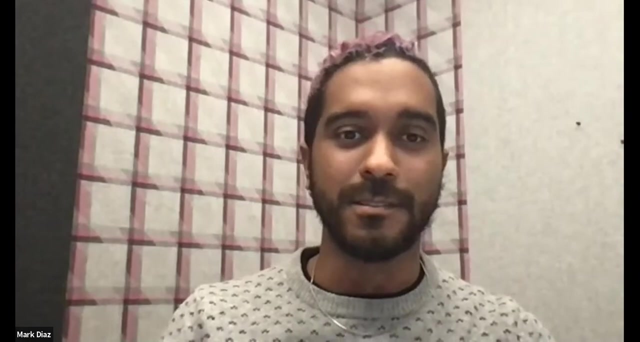 um at georgia tech, and so it's this, like great confluence of minds and people, that i think will stand as a good example of how to do this again moving forward, and so i'm excited for for that, as as a successful um, it's still ongoing, but it has so far been successful and i hope for sustained. 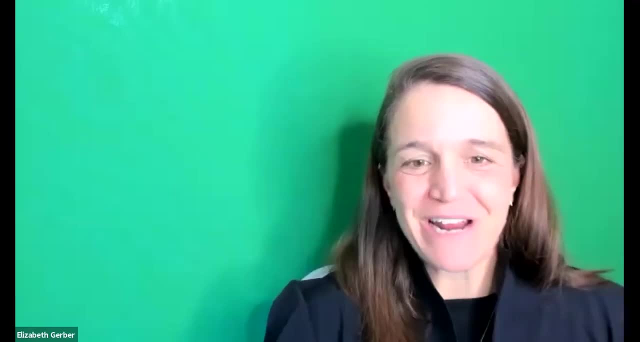 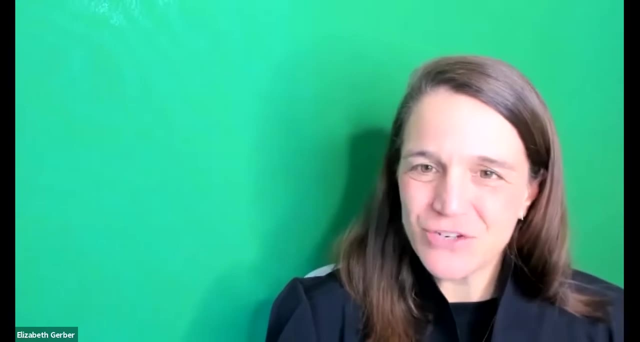 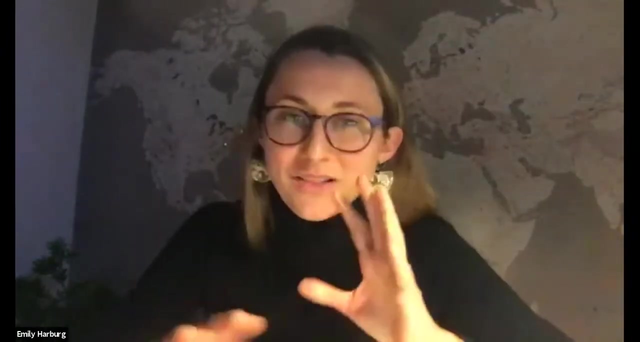 success. thanks so much, mark, and i really appreciate you calling out um those wonderful researchers by name. they are um doing fabulous work. thank you very much, emily. did you have uh? did you want to jump on here? sure, yeah, i think uh one case study for us that i think was interesting. we've been doing a lot. 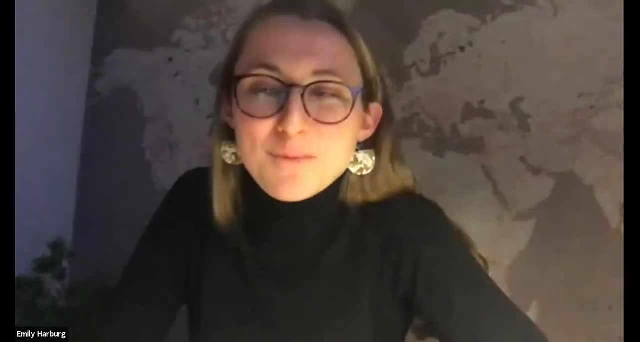 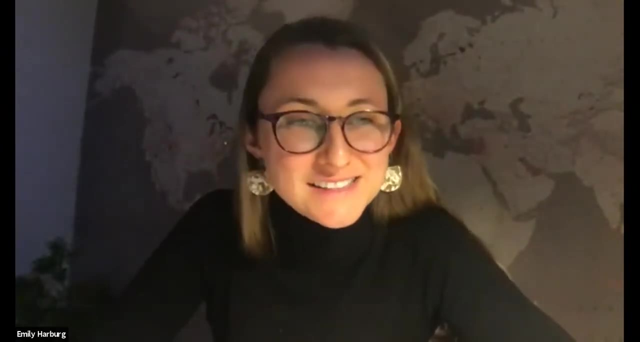 around. obviously, kids can't be exploring cities as much right now, but we've been been looking at even from home, and when kids can't travel the world, how could they still kind of explore cities where they're living, and so we ended up doing some scavenger hunts that kids could collaboratively do. 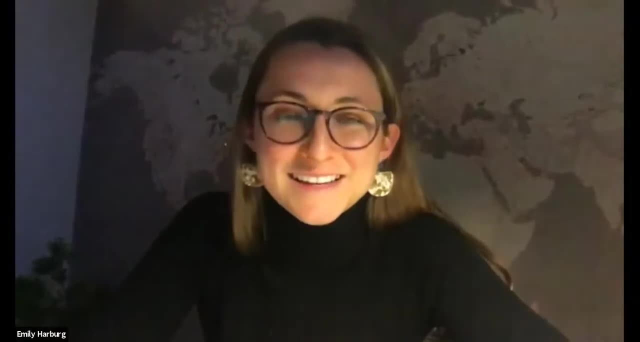 and kind of connecting with others and then actually go and explore and to me it was one of the first times i really was seeing like kids, you know, not just looking at their phones but using it to motivate behavior and to talk to people who had opinions that they didn't necessarily agree with, and to learn and 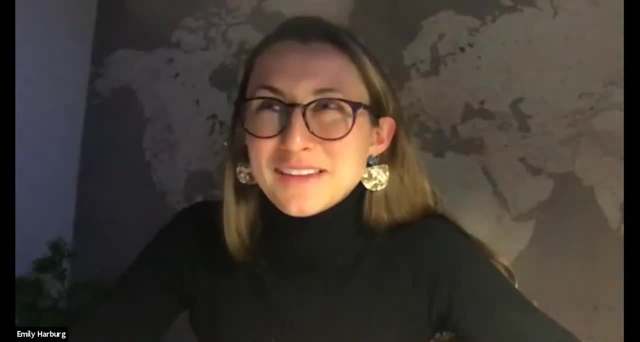 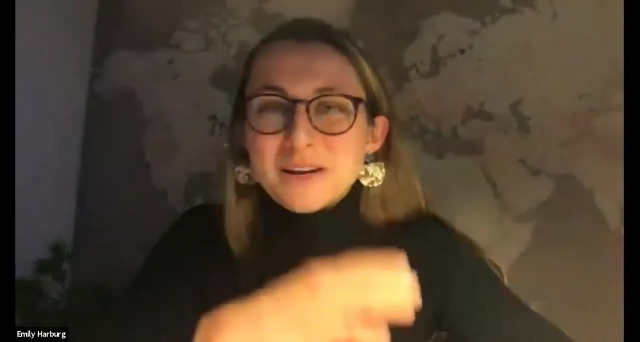 engage with others. so i think, um, for me that was one that really exemplified where tech can kind of help spur that interaction and engagement and understanding. um, i think one other one that was that was pretty interesting was we did um some ar experiences where you could actually scan, like 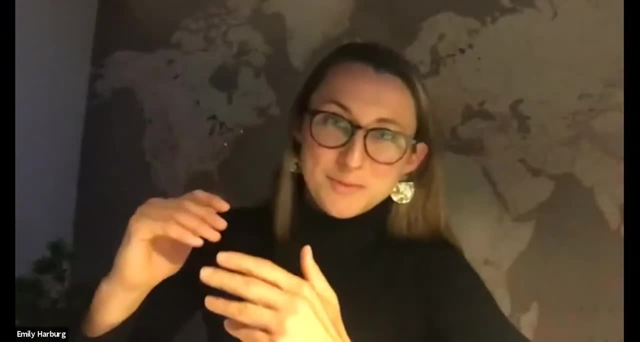 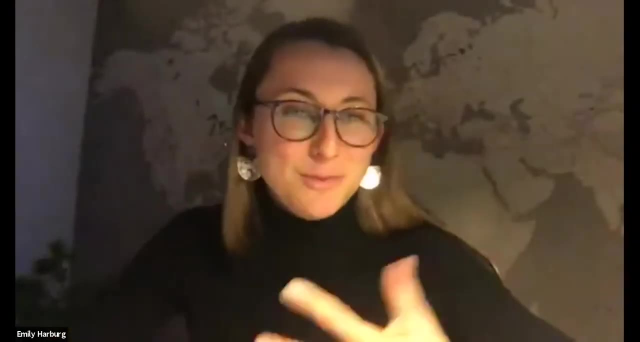 we had that um during d-day. you could stand at the beaches of normandy and scan the air and see what it was like with the planes coming in, or scan a photo of a veteran and he would pop out and talk to you about what was. it was like on d-day, so to me those were also some really cool. you know the. 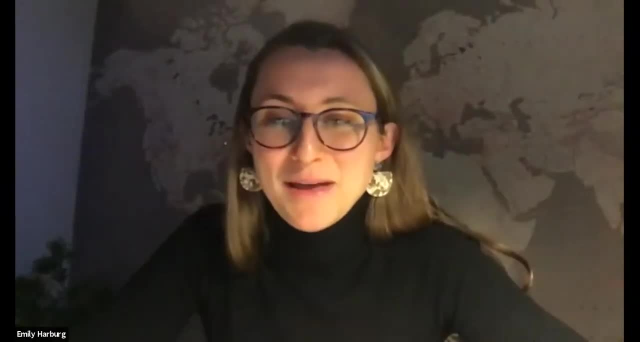 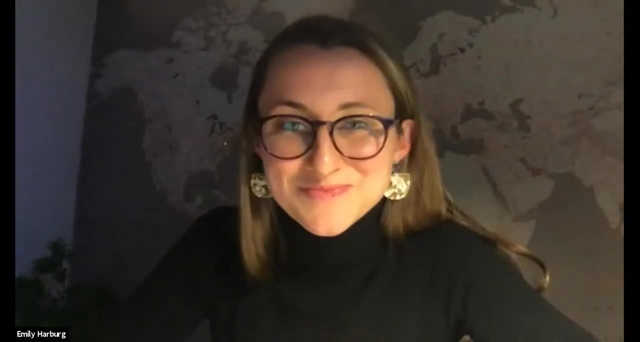 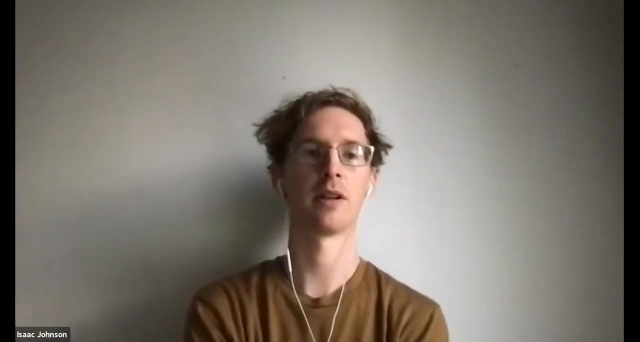 use of tech to kind of engage and interact and learn um and and ask questions kind of in new ways. so i think i think those were two that i was particularly excited about. thanks so much, emily. yeah, and i'll jump into and uh build a little bit on on mark's point about 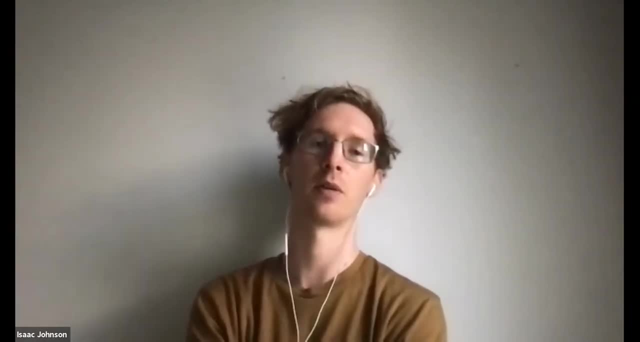 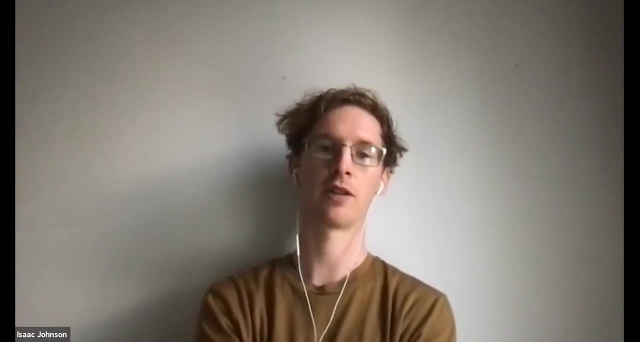 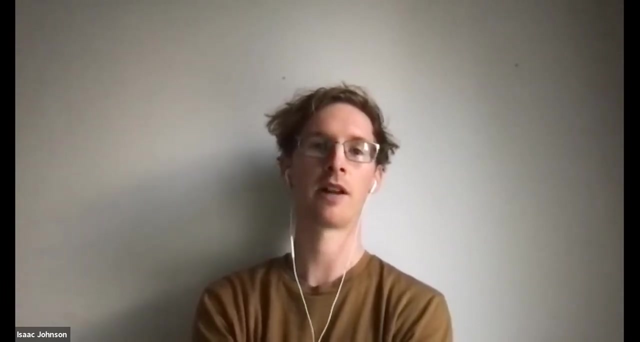 the kind of like broadening participation, one of the kind of fun things for us. so with english wikipedia- obviously quite big- there's a huge resource they're trying to protect, so they're a little bit slow to be interested in experimentation and things like that, a little more conservative in their kind of approach to change, which makes a lot of sense, whereas a lot 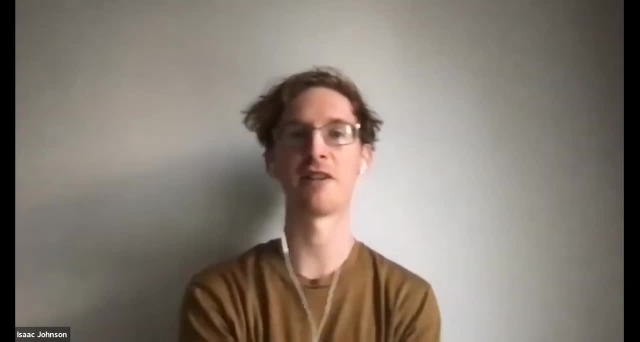 of the smaller language communities are really trying to like experiment with things and like try out new things because they're trying to grow um, and so in many cases it's like i mean just absolutely fabulous these communities, because they're willing to put aside a lot of time to kind of talk with us. 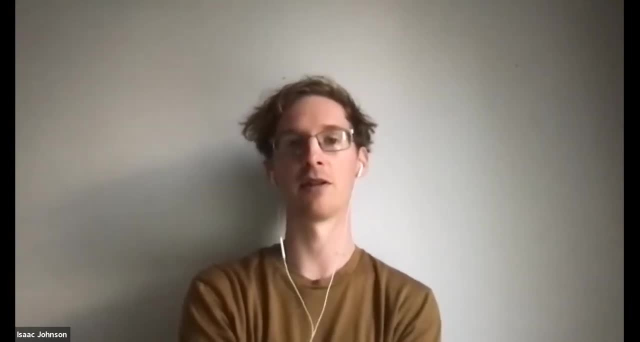 through the issues they're facing and think about and just try out new, you know new- whether it's new onboarding experiences for editors or kind of new tools for you know, like recommending edits they might make and things like that, And so that's been really a lot of fun just having those. 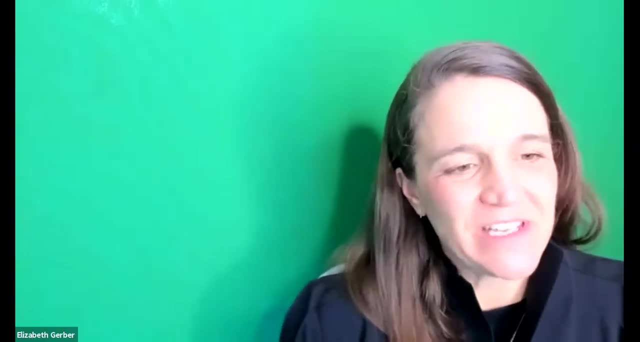 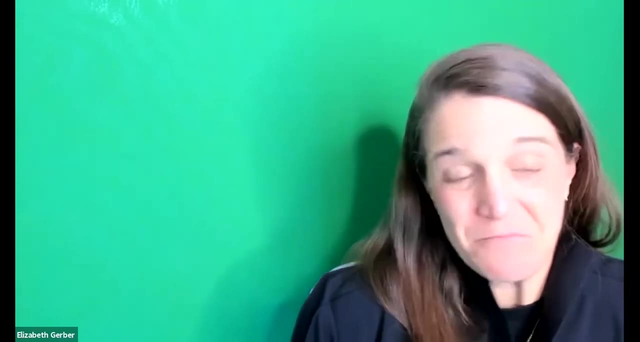 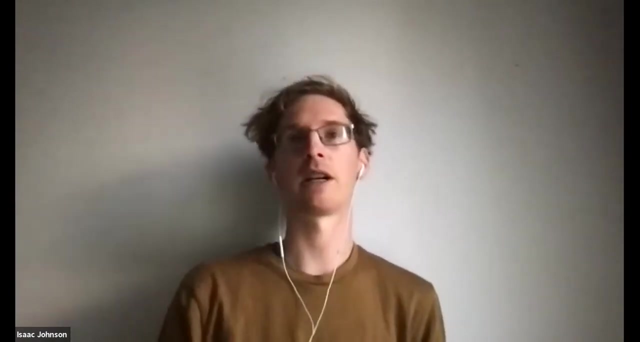 collaborations. Isaac, did you have a specific community that you've worked with recently that was exciting to work with? when you say I'm curious, when you think about broadening participation, what groups are most exciting to work with? Yeah, so we tend to kind of break our 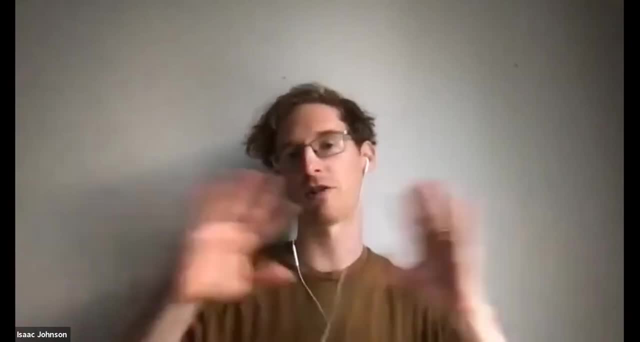 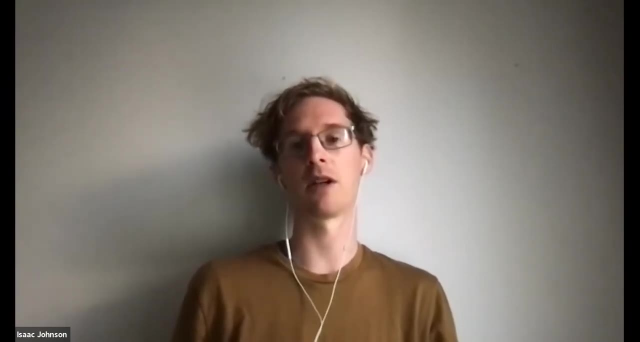 communities down to like large, medium and small, where large would be like English or Spanish, some of these really huge languages that span a lot of areas. The medium-sized language communities: these are things like Czech, Korean, those, you know, languages that have like a 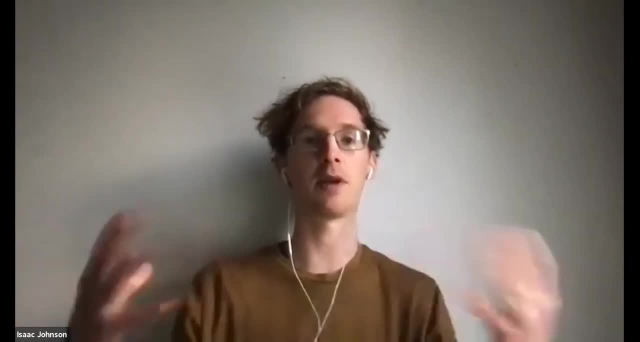 an on Wikipedia have kind of a community that's like built a fair bit of content but it's still relatively small, often because it's, you know, focused in a smaller geographic area or something like that, And so working with it is, yeah, it's a huge, you know huge diversity. 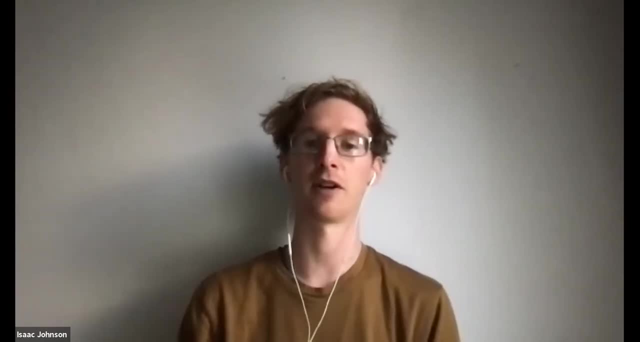 a lot of very different languages and you see really different kind of responses And just like like one good example there, it wasn't my work in particular, but some colleagues at the foundation were trying to understand. so on Wikipedia you don't need. 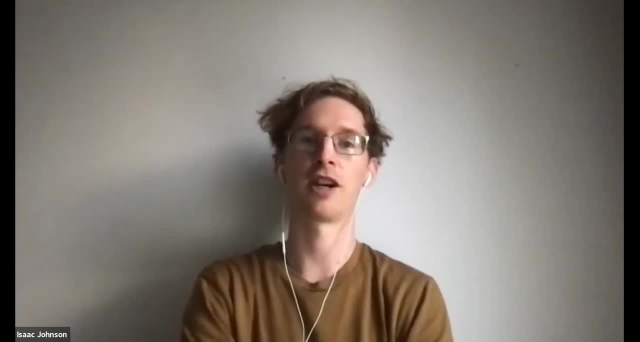 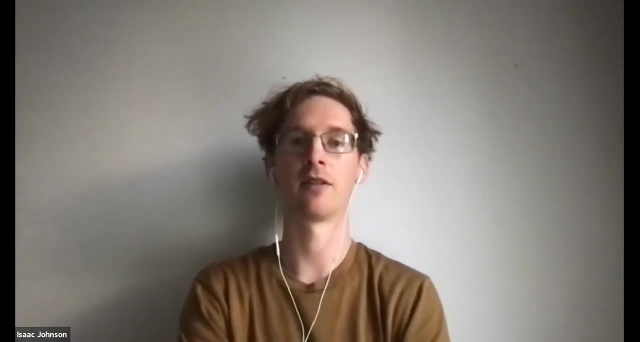 you know an account like to edit or do anything like that. So we're trying to understand, kind of like, why do people create accounts? Because really the only real reason is to edit, And we're finding a lot of these language communities that have come online later than say a lot of. 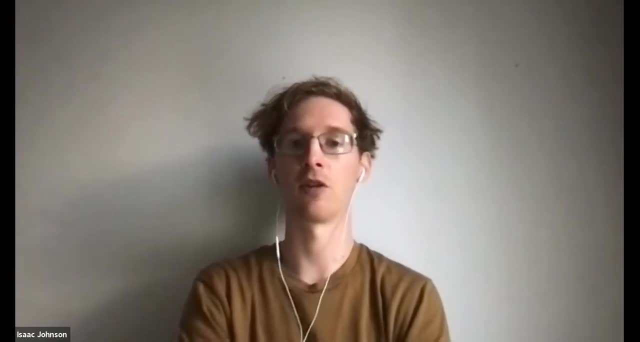 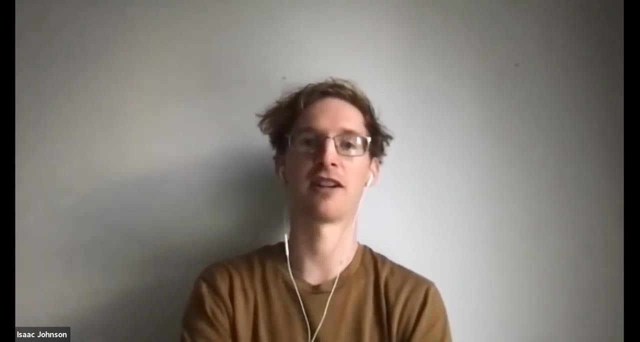 the English communities that you know, people were just assumed they needed an account to to edit or to like, read and access Wikipedia, And it was just really interesting to kind of learn some of these. you know you call them misconceptions because, but like 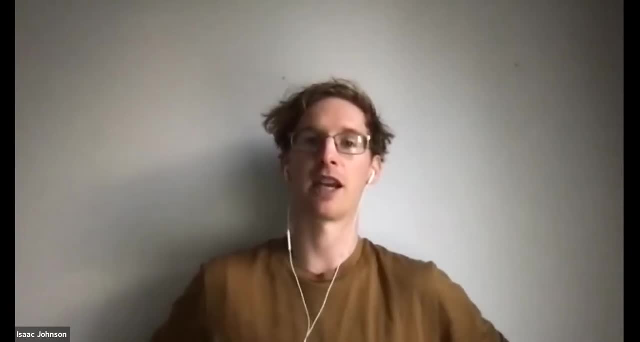 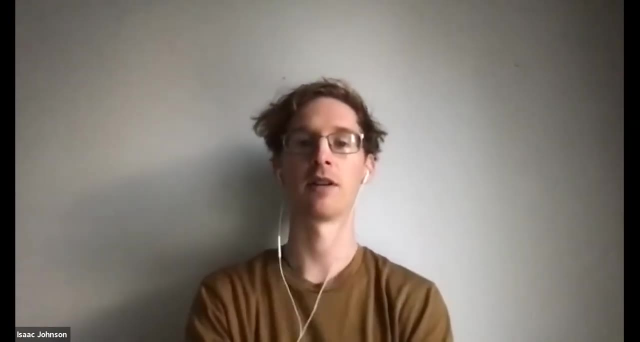 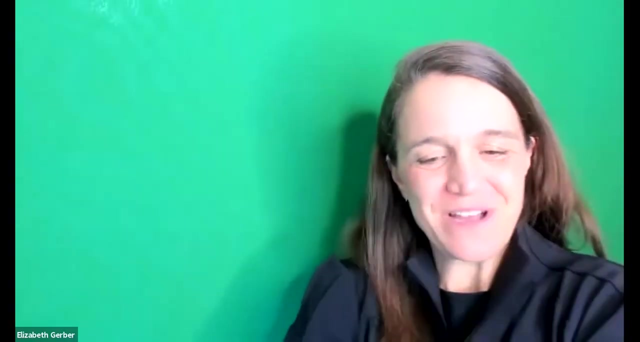 just the reasons, the motivations behind why people were taking some of these actions. that really kind of helped us understand some of these workflows and, oh where, maybe do we redirect people or does you know? that sort of thing. That's great. Thank you, Isaac. I'm going to move on to another question, which 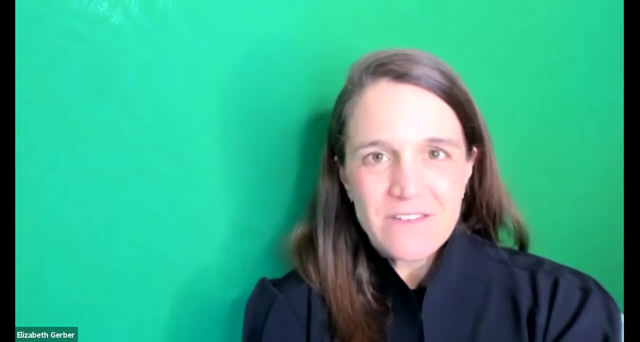 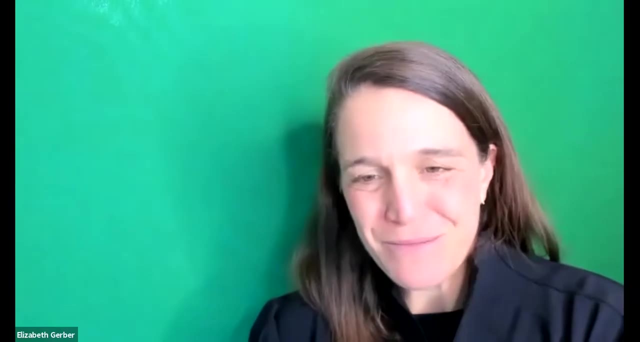 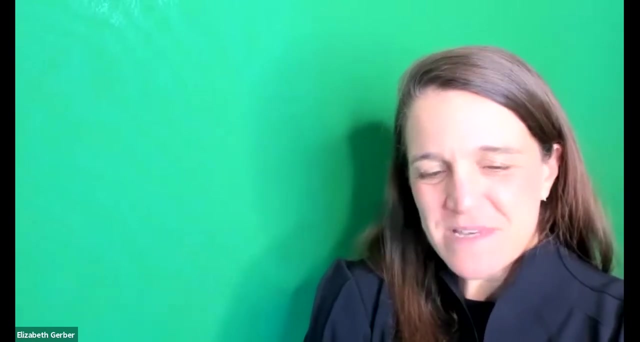 is really about the business case for overcoming these grand challenges. I think a lot of you've already suggested a lot of you in grad school- that you weren't necessarily thinking about the business challenges. So I'm curious, now that you're steeped in industry, what are the business cases for? 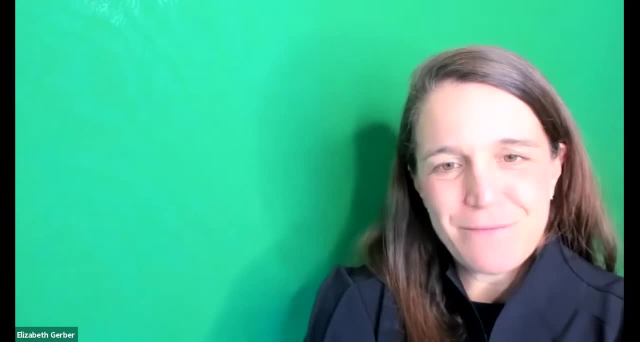 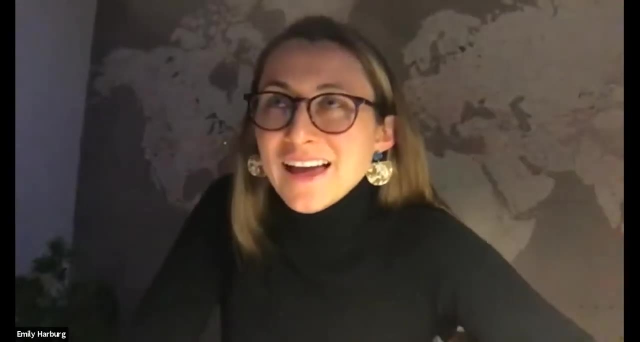 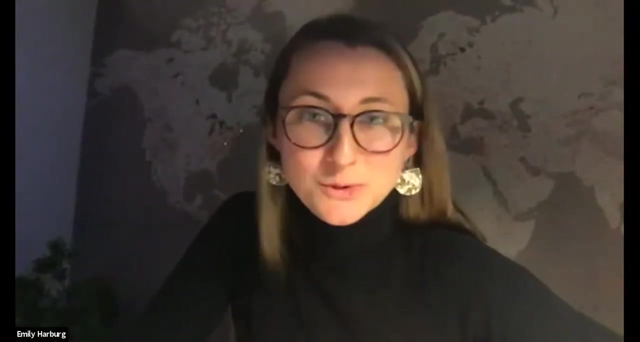 overcoming these specific grand challenges that you each have shared. And maybe, Emily, I'm going to start with you, if you don't mind. Sure, Yeah, I mean, I think. well, I'm thinking now, from everything Isaac and Mark have been talking about, I do. we've been talking a lot about accessibility online for our tools. 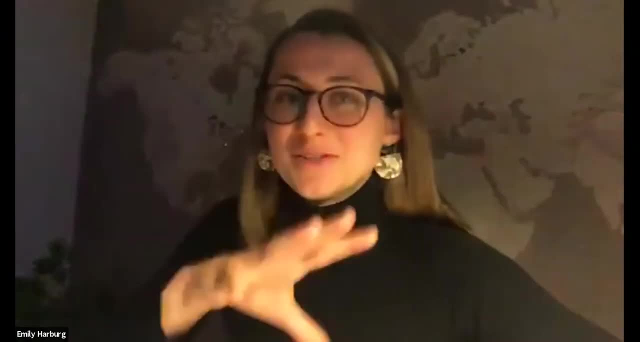 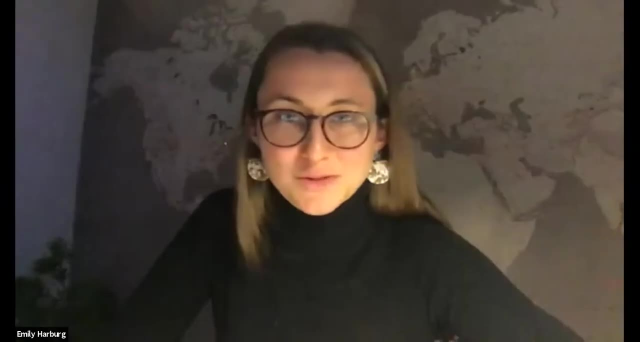 as well, And I think with our we have an older adults travel group that we focus in on as well, and but not even just for older adults. but I think we've been thinking a lot about, you know, for those who are hearing impaired or vision impaired or you know, kind of going onto the site, how are they? 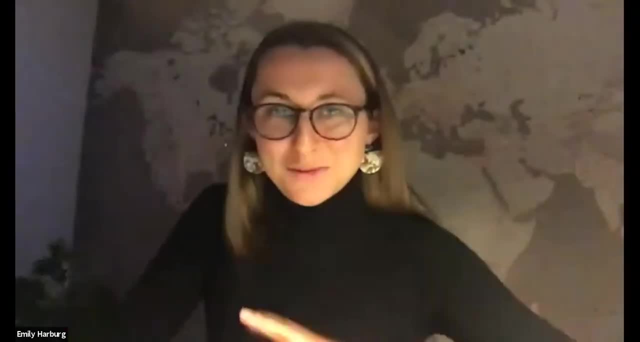 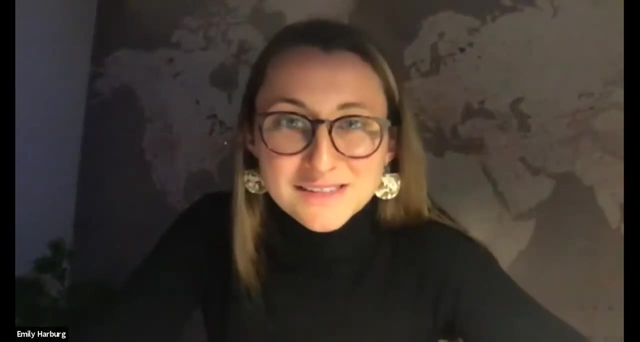 experiencing the product and- and at first you know, it seemed like an interesting research problem or a challenge, but of course it's. it's hugely important for the company to be able to serve those audiences as well and be able to have them as customers, and so I think, if you know, those are. 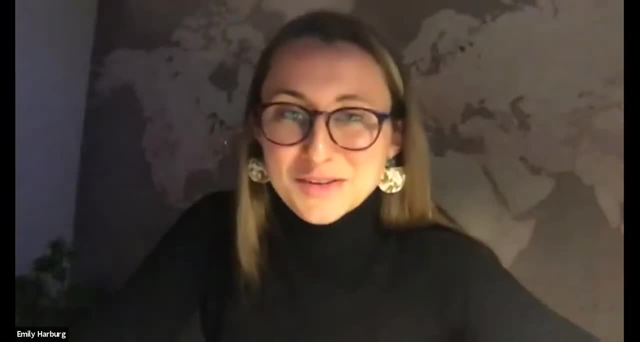 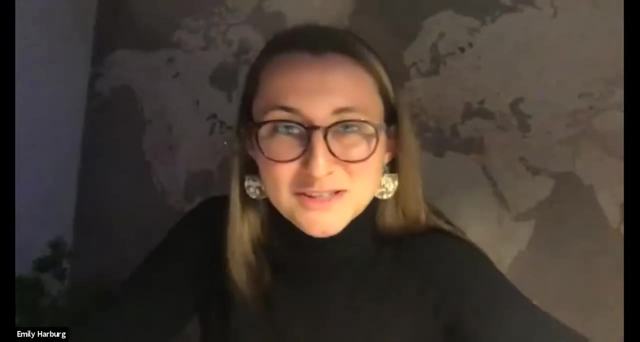 the best scenarios that when it's actually good for society and also, you know, is is positive for business as well. you know that's an ideal combination, but but I think by focusing in on populations who are not fully represented, we're able to serve and and support so many more people. 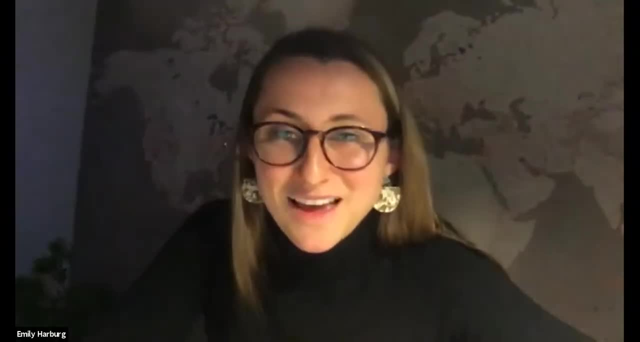 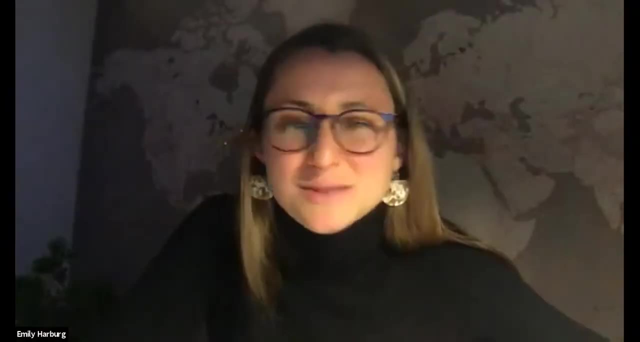 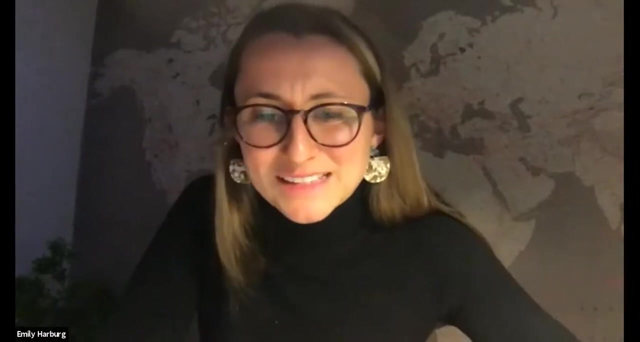 so that was one kind of quick thought that came to mind, kind of in that vein and, I think, also on the like brave sides. as Liz mentioned, I for the past five years been helping support a non-profit that we started focused around helping women learn how to code, and it's been amazing because 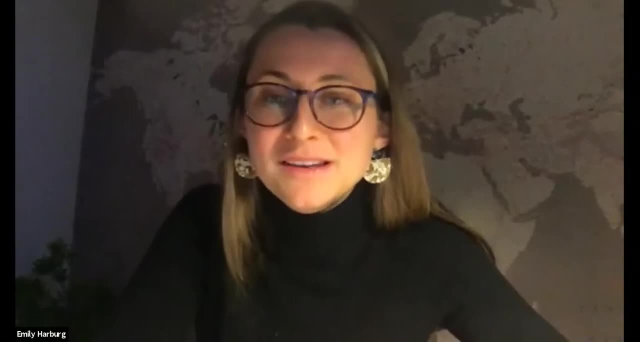 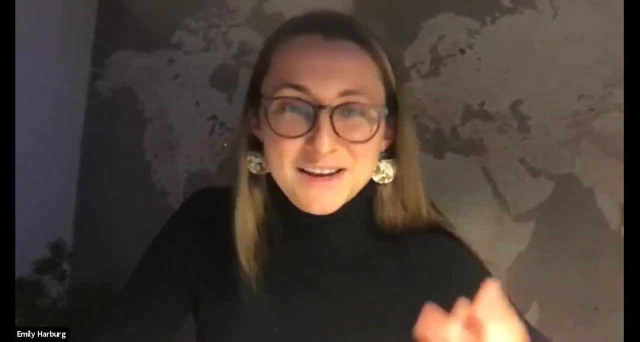 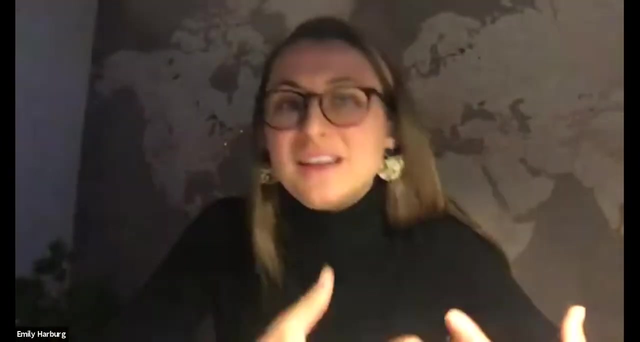 we've kind of moved now into the prison space and helping teach women who are pre-released from prisons how to code and kind of building websites for social impact, and it's to me it's it's again an example of voices that are so powerful and have such so much to give and and society and businesses will benefit if they. 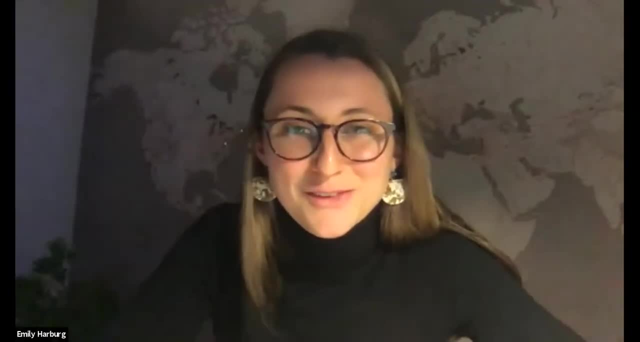 can open their doors for those populations as well, and so I think for me, even in the way we build, it's advantageous to be including different voices and perspectives, and we build better systems when we do that. so, thank you, I think that I'll just on the brave side. I'm also passionate about that. 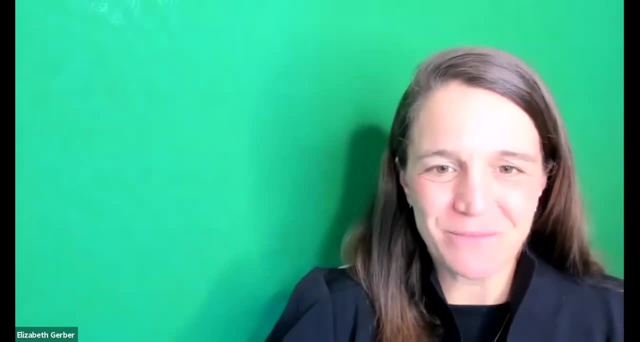 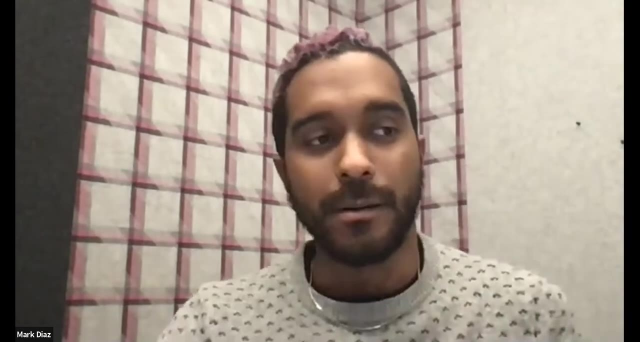 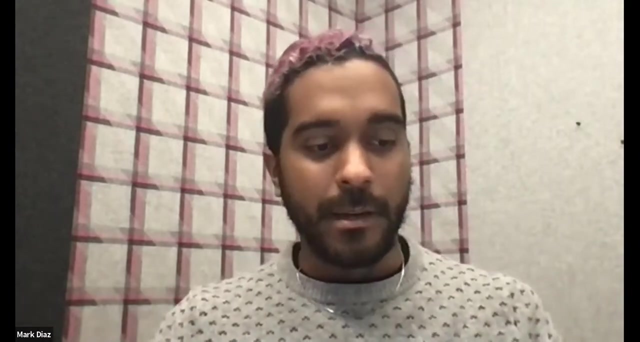 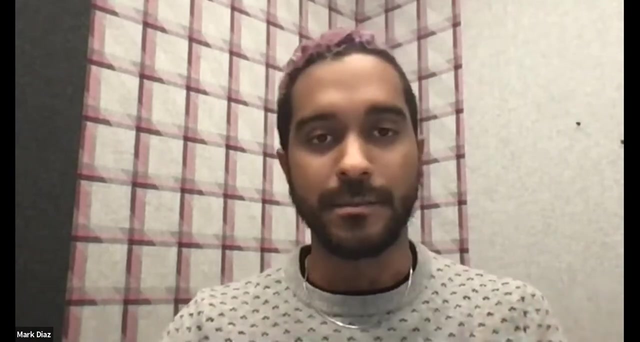 thanks for bringing in that work too. Mark, did you want to jump in? yeah, I can definitely echo a lot of what Emily is saying about there's this kind of broad sort of view or argument to be made. I think about, you know, being more inclusive. I mean supporting more people and, from a product perspective, more users, more positive experiences. 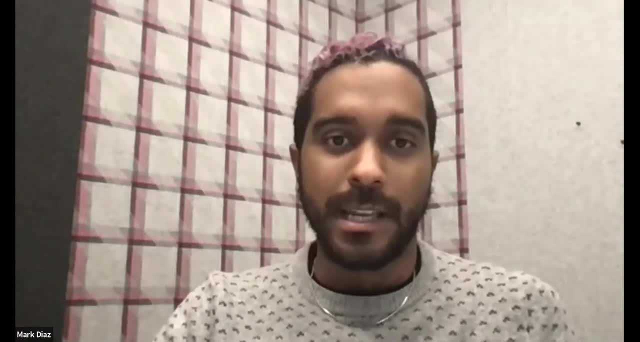 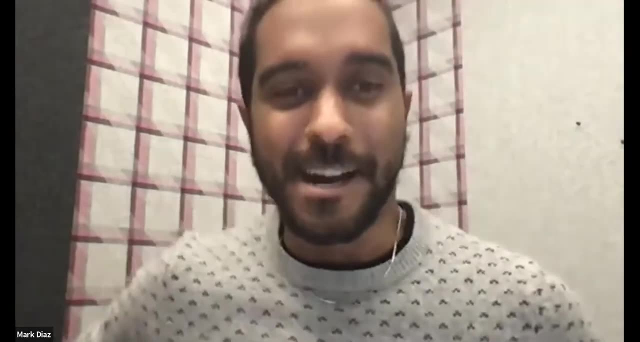 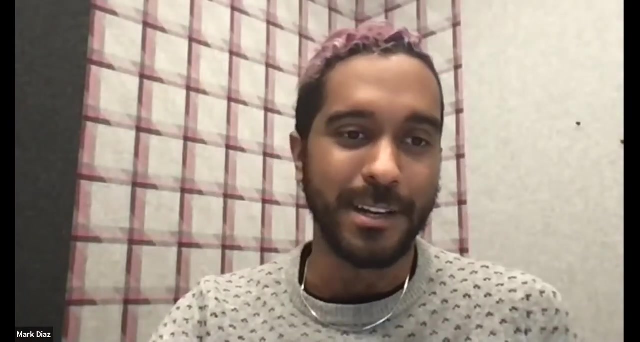 but I also struggle sometimes actually to make a, a case or to, I guess, like articulate in a business sense. it's definitely not my first. my mind doesn't start with those questions. I find myself kind of reverse engineering. oh, these are certain research questions I have, or or certain issues that I think needs to. 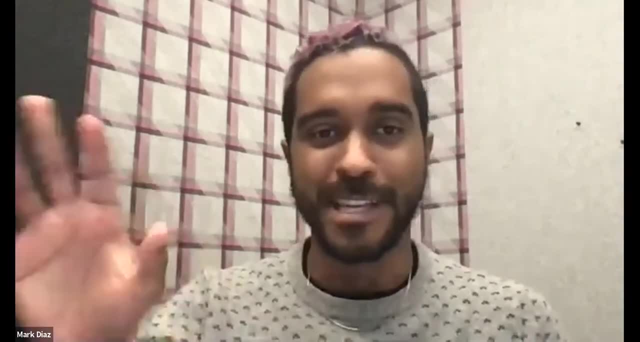 be audited in a certain way, and then I, I can sort of say, let's avoid a PR scandal, right like so. I think a lot of these questions are sort of me asking myself this or this question, or this or this question or this question… right like so, I think we've kind of sort of- you know, I'm working on this at a certain point, but this is we're. we're kind of sort of. 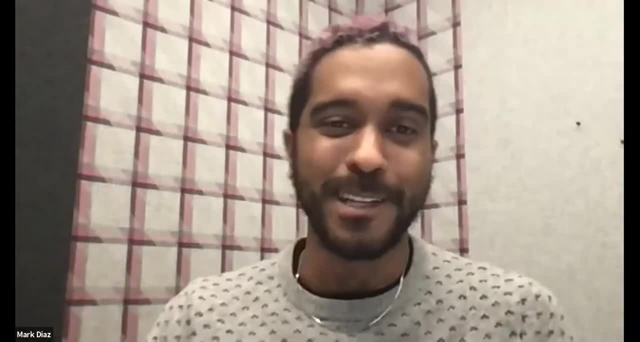 like that. but I think we're kind of sort of at a certain point- but I think we're kind of sort of focusing on that- because we've just I think we've kind of sort of right like scare a business like that's one way. you don't want to lose money either, um, but it is. 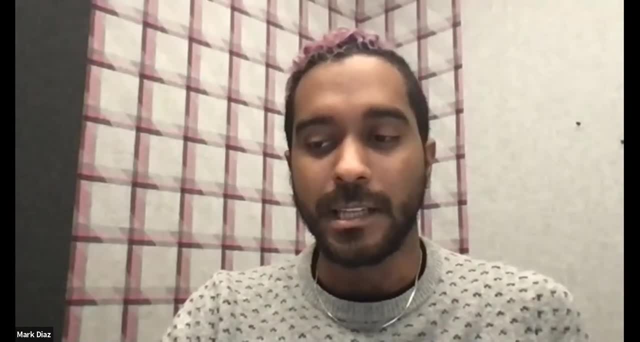 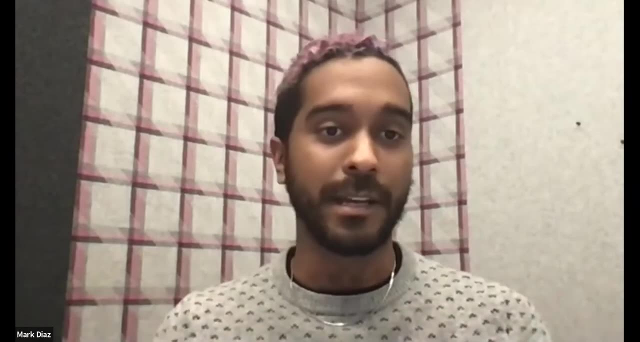 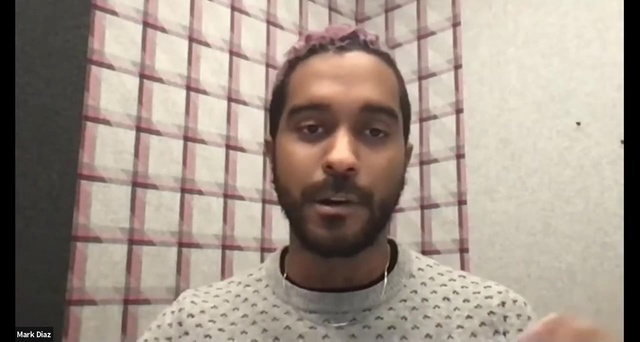 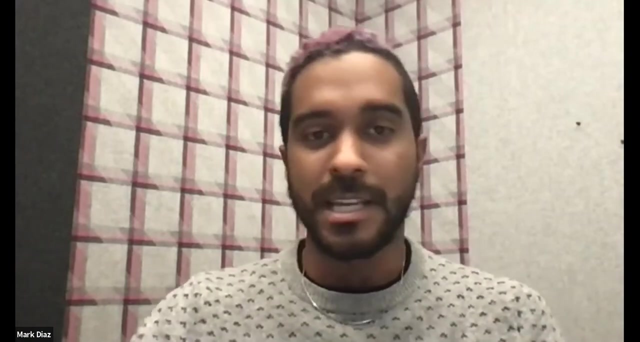 something that i do find to be pretty tricky, um, and less so at the level of, say, getting buy-in from leadership about identifying that an issue is important, but really, um, peers and people who are maybe just slightly above where i am because, um, sometimes and oftentimes, um, there's extra steps. 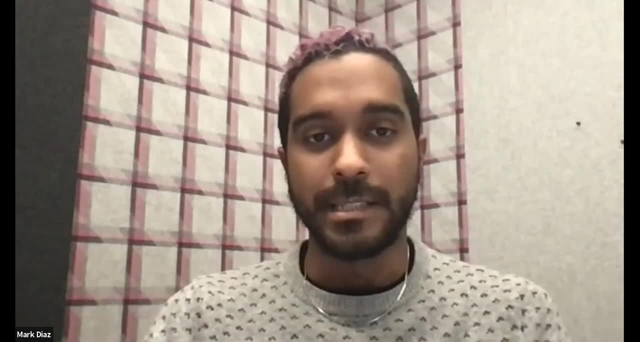 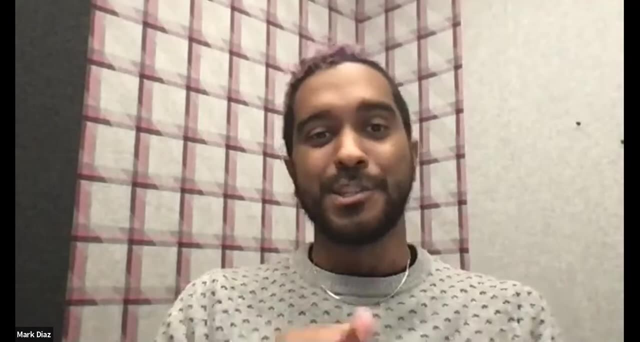 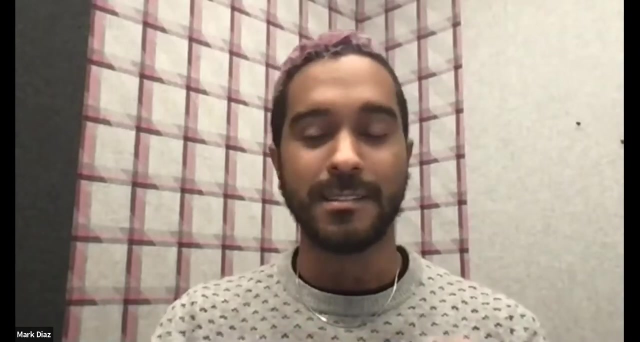 that you're adding to somebody's workflow, um, and especially when it's not the norm to have a very inclusive process, it means starting out changing people's work practices and just because, like, changing your routine is easier said than done, um, and it can be really frustrating for somebody. 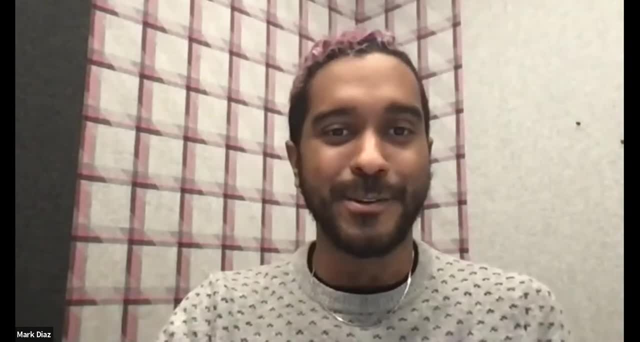 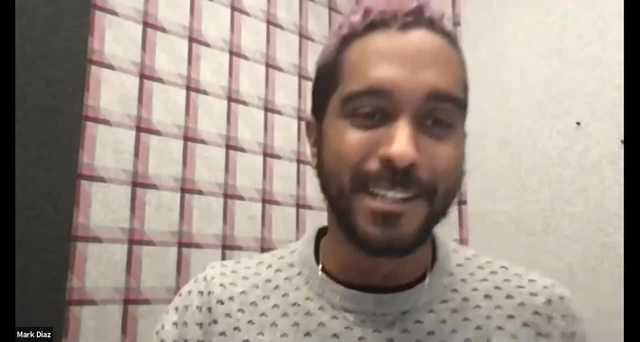 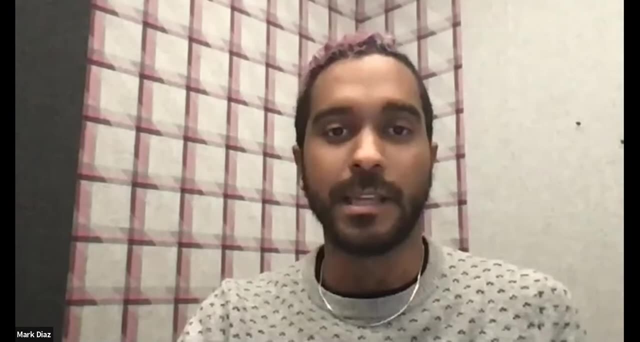 do your job better, like that's never gonna. that's not gonna convince many minds, um, and so i think that's where the biggest challenge for me lies, and so learning that language of how to um bring people in in really compelling ways, um, because i think at the high level, a lot of folks are 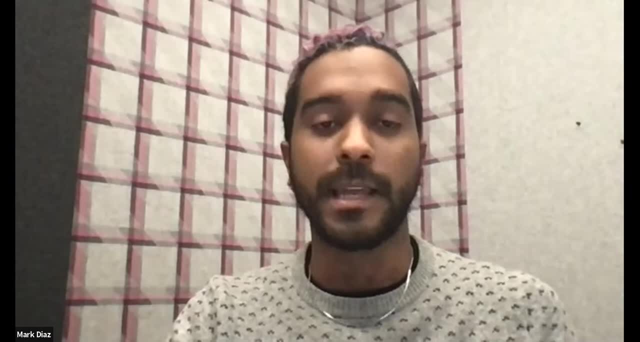 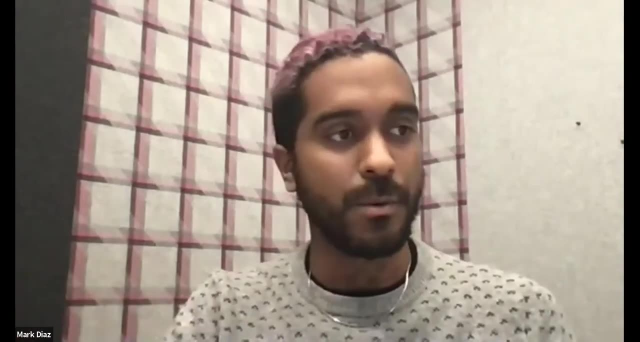 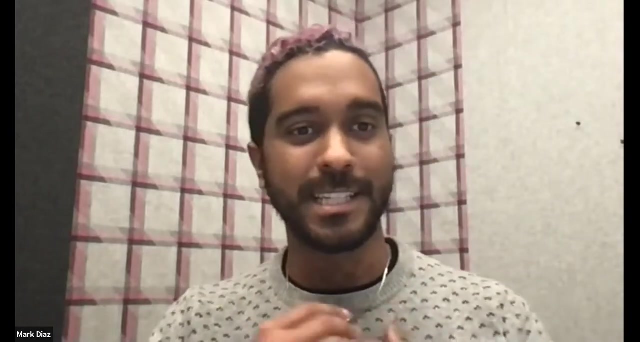 really interested, um, but they're spelling out in a very detailed way. hey, um, this is how we stand to push away users or create systems that aren't working as efficiency, even if i myself am less interested in, say, specific um benchmark accuracy compared to some other way of measuring. 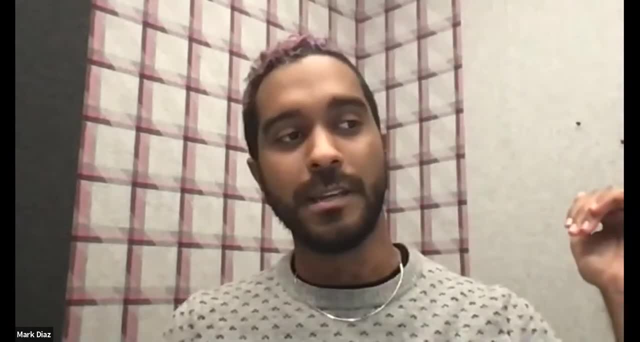 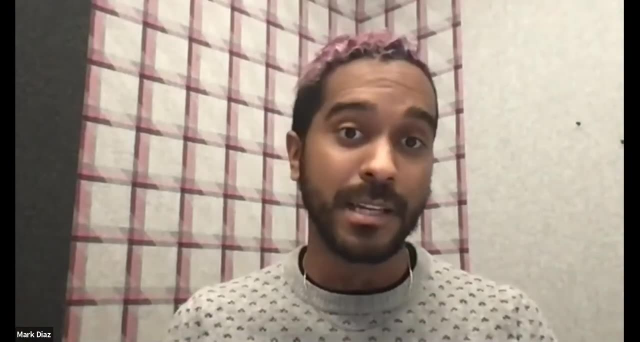 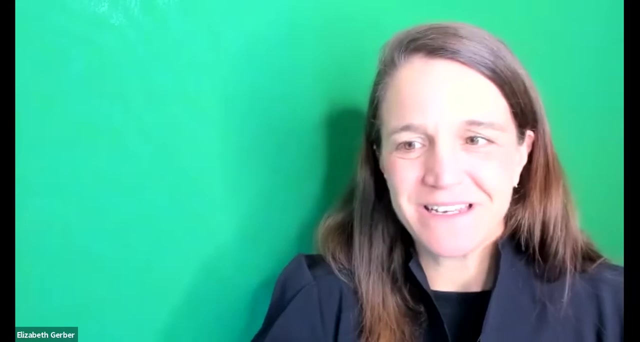 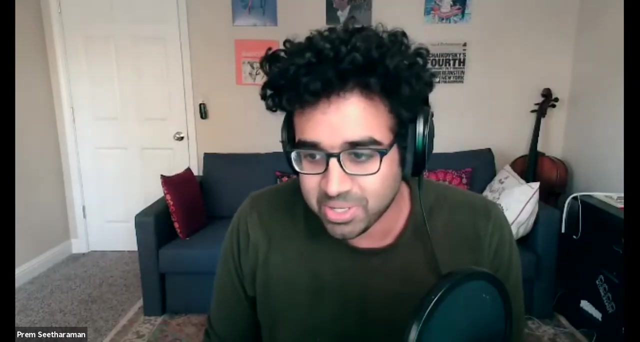 performance. i still need to make a case around the metrics, benchmarks and, honestly, um sort of references that other folks have been using and still care about. thanks, thanks, so much prime. did you want to add something? uh, yeah, sure. so i mean the business like looking at things in terms of like a product lens versus a research lens. it's like a very kind of new. 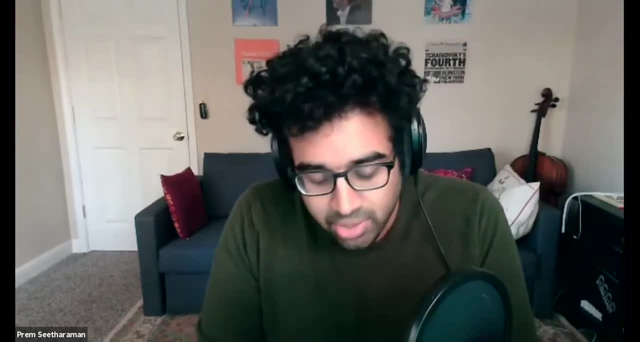 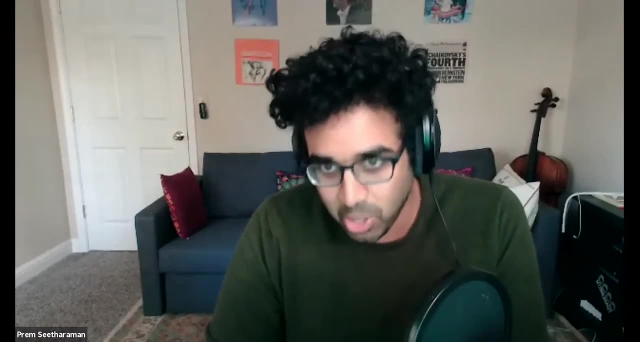 experience when you enter industry and like one thing is that, like all the things that you care about in terms of research are just not going to ship, like they're not going to make it into the product, like for the, for like so many things we're just not going to make, like solving, like certain. 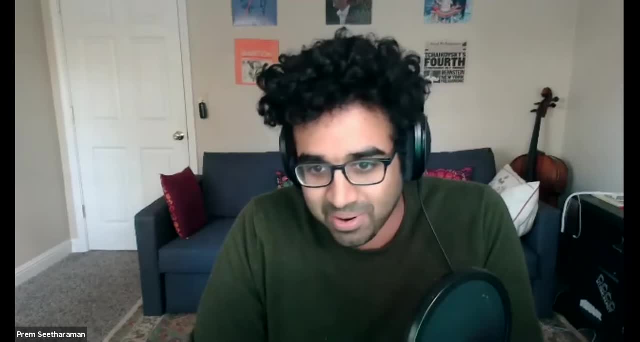 problems in computer audition, those don't have any near-term application for our product, for example right, even though they're things that we're not going to make it into the product. so like i mean i would say there's a lot of things that i really cared about in grad school, so like 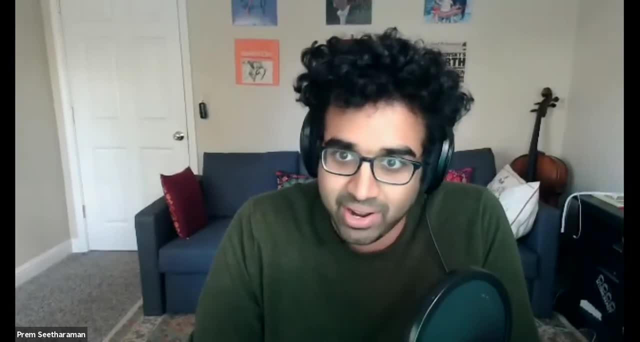 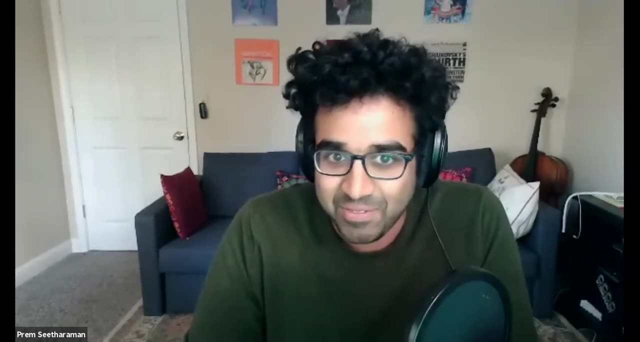 in grad school i worked like a lot on like unsupervised learning and like self-supervised learning, but it turns out in industry supervised learning just works better, right, because like if you just get the data set and then make it work and stuff like that like a lot, of, a lot of the times. 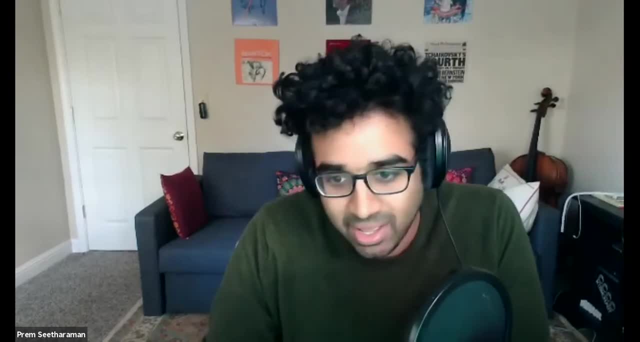 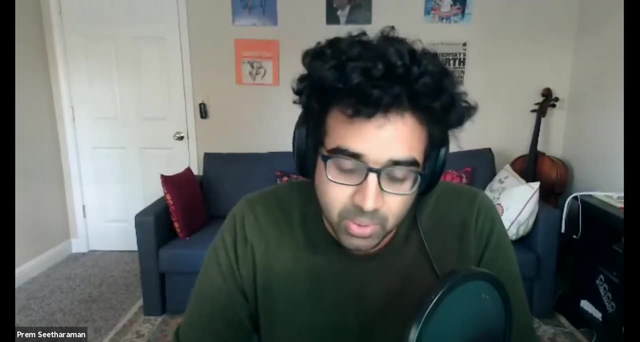 that's going to be the way to go right. so, like you end up shifting gears quite a bit um towards a different set of problems um than might, then you might have wanted to work on um, but it does open up kind of new challenges. so i'm not sure how you guys would address that in the chat. uh, what's your? 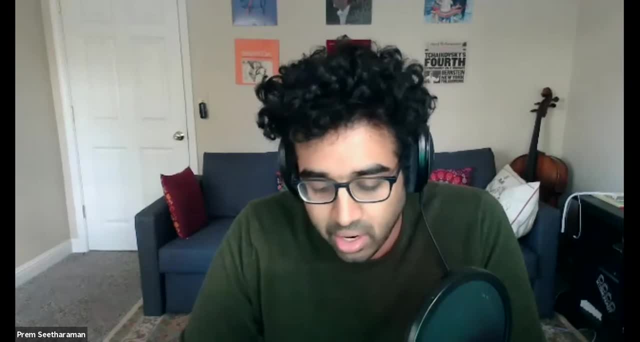 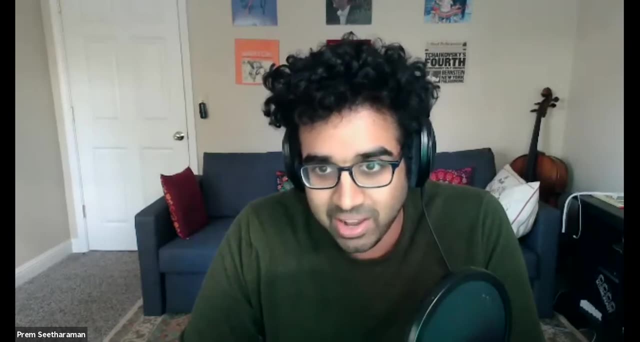 and things like that. and the other thing is you end up focusing a lot on tinier, like like i said before, like tinier things. like getting things to actually ship uh requires like a lot of meticulous sort of research, highly extensive qa, for example. like we ship models that um, like re-synthesize. 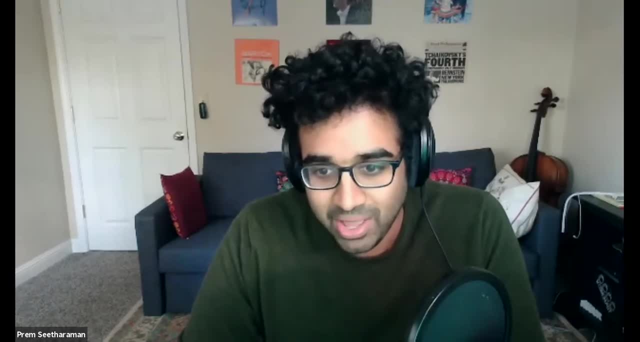 your voice in like good recording conditions, right. so the qa that we do for that is like way more intense than anything i did in grad school, right, because if we ship it wrong, then people start yelling at us on twitter and that's bad, right, so i mean like there's a lot of. 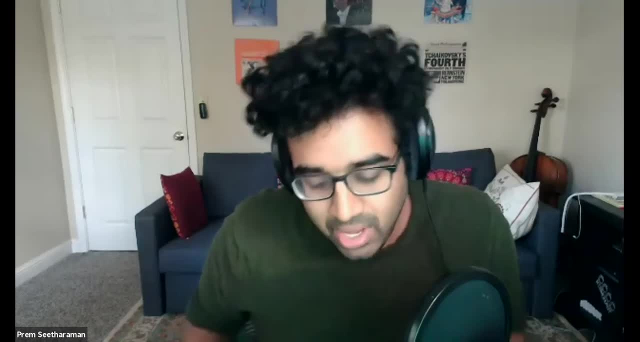 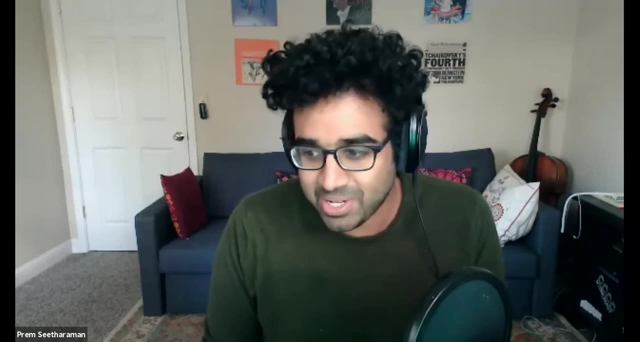 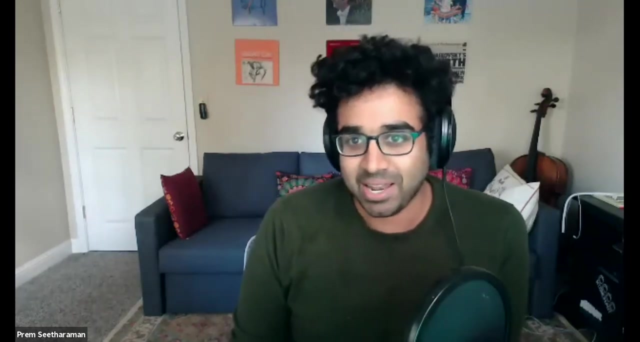 things like that that end up happening. um, so like where you are like the fun part of research. i mean the job as a whole is fun, but the fun part of research is like, uh, shorter than it was in grad school in a lot of cases. so i mean i spend a lot of time really trying to extract as much fun out. 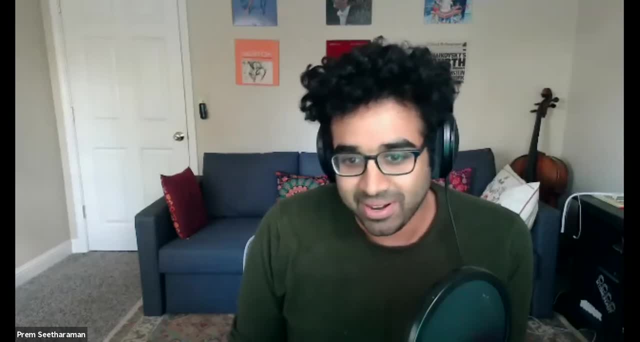 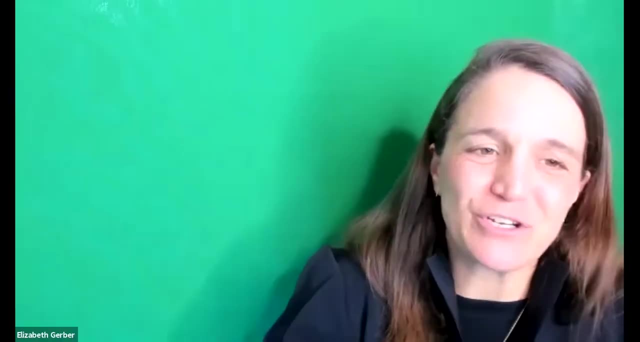 of that period before i have to move on to the painful period of shipping it um. so that i mean, like things like that have shifted a lot for me in industry. okay, then i have to push back frame and then say what's more fun about industry than academia? there's got to. 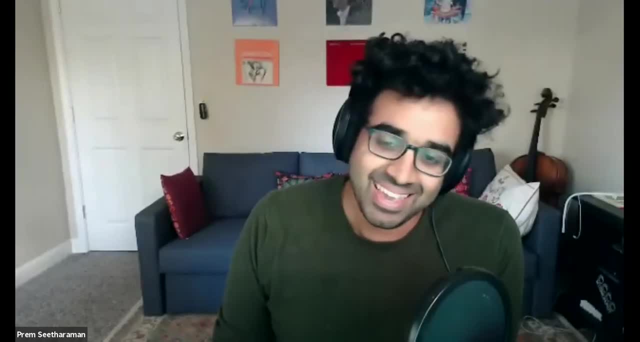 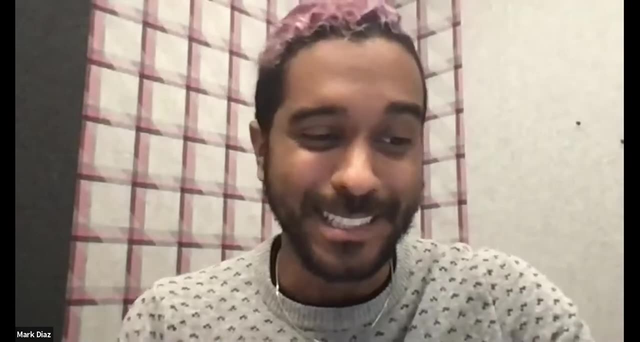 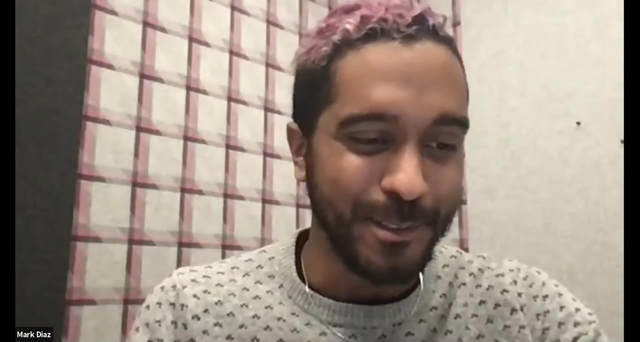 be something that's more fun. i mean, you get it on the other side. yeah, when you ship something, you're shaking your head mark. come on. uh, i was gonna say pto stands for what paid time off. um, having a nine to five is wonderful, although many of my co-workers 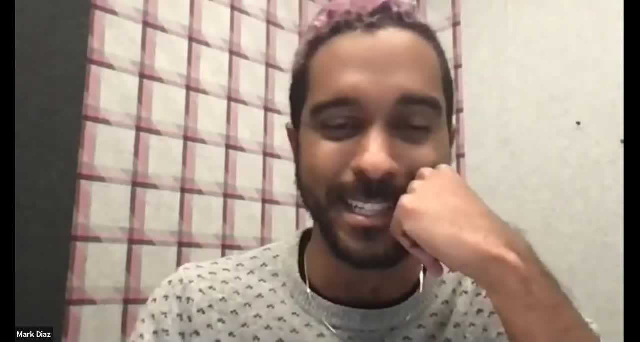 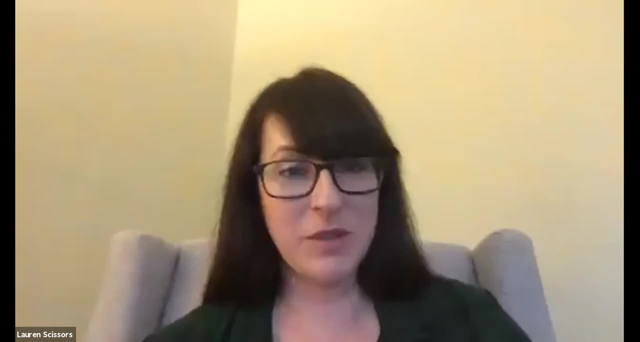 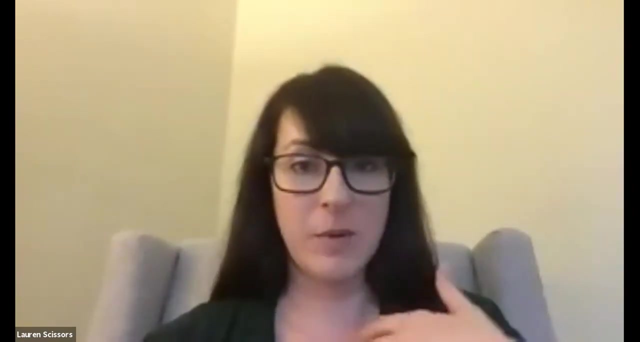 um have carried over their uh grad school working uh habits, which is not good. i will. i will say for me, one of one of the multiple more fun things was you get to work with people with a lot of different skill sets that, you know, i really was not exposed to in grad. 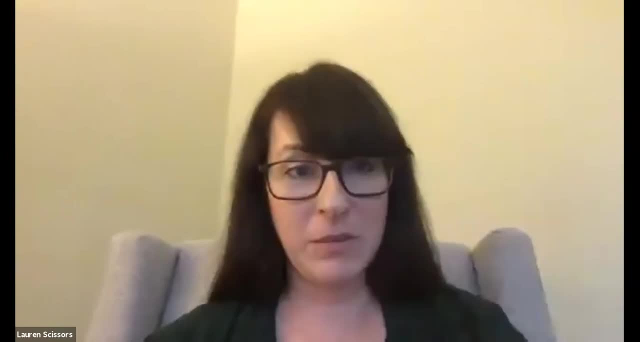 school, and when all those people come together, you can actually make a feature or a product and You can actually put it into the world, and you can do it on a relatively short time frame and you can debate the merits of who you are and you can do the work that you're supposed to. but when you're 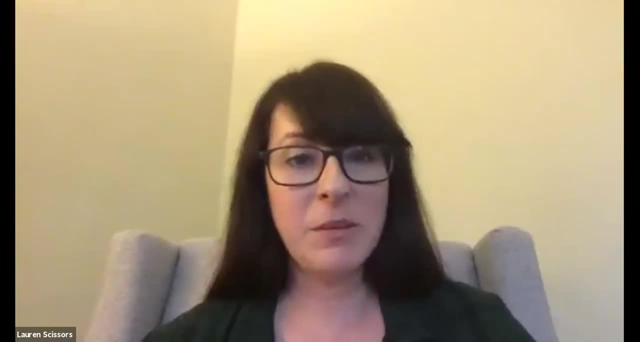 whether it needs to be a longer time frame or not, but actually making things- in my case, software, like making software, designing things and putting them out into the world and having people use them and get value out of them. I think it's very fun. You know, maybe you could. 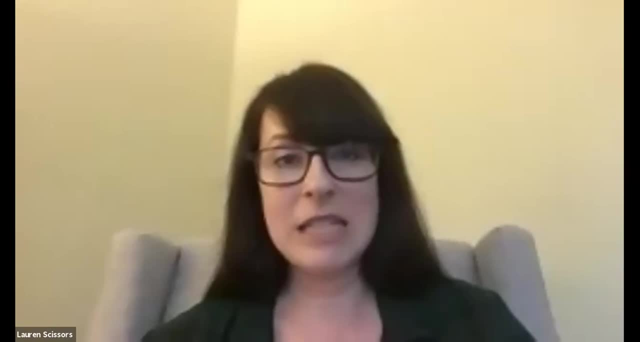 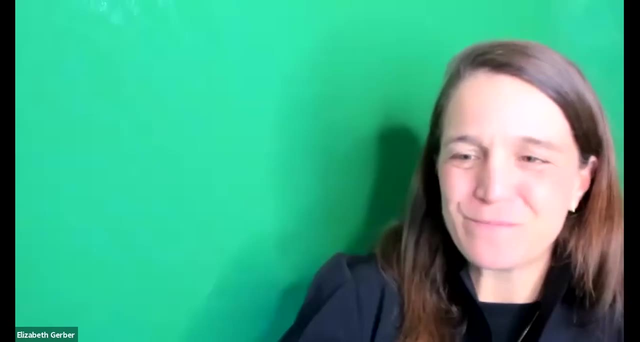 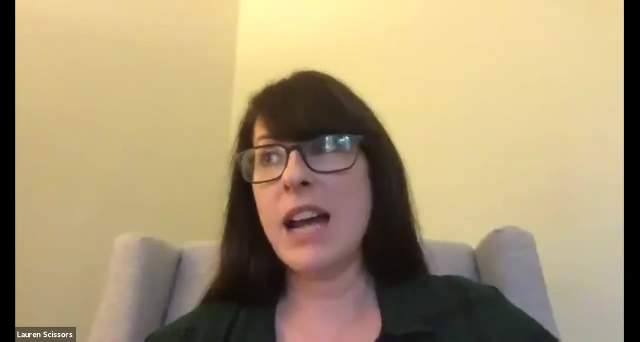 pick another adjective like fulfilling or rewarding, but it's not abstract, right? It's like you made a thing and you put it out there And that is pretty exciting. Lauren, do you have a specific example of something you've worked on that we might know about? Yeah, Back in the day. 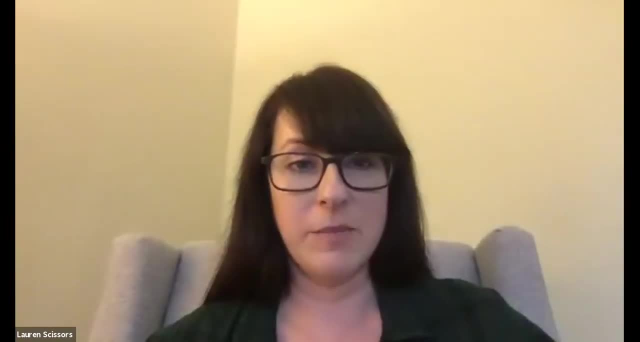 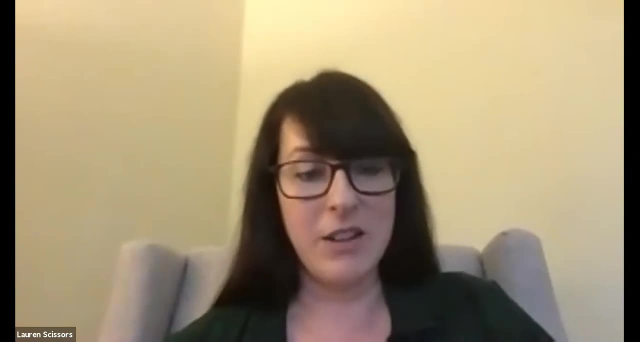 my team and I worked on the original Facebook reactions, So those are the emoji that you can leave on a post. So before that you could just leave a like a thumbs up, and now you can leave a range of pieces of feedback. So we did a lot of research to figure out what should they be. 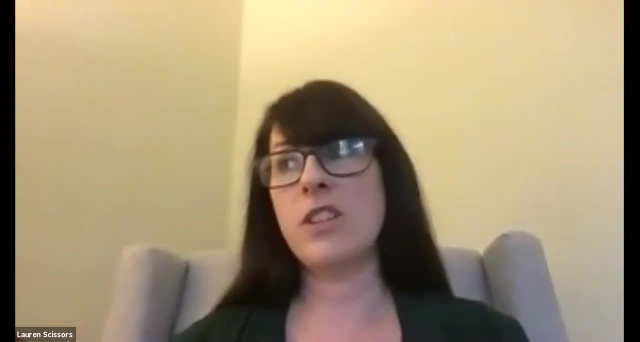 And ught to do research in a number of different ways. So, okay, what should the set be? from this many options down to this many? How is it going to look on different sized phones, right? So at the time, the biggest phone looked like this, So maybe we could fit one more, but what about all the? 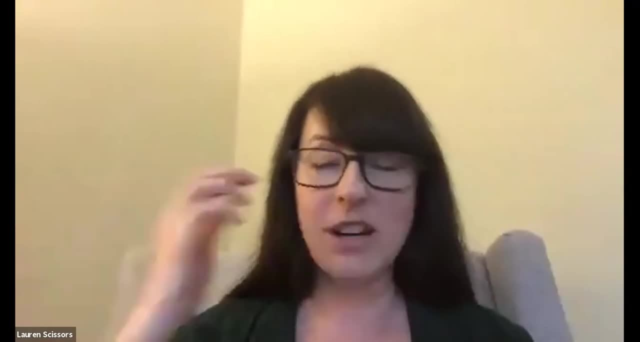 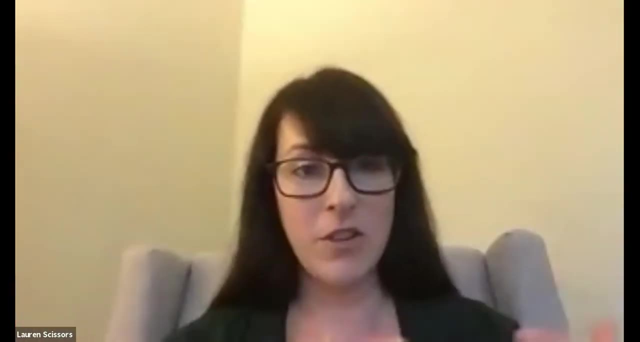 people who have smaller phones. Maybe we shouldn't put that one extra one To. you know everything in between, So very like abstract. you know emotional type research to very specific usability. you know pixel here, pixel there, kind of research, And you know we were doing it because we had a lot of user feedback. 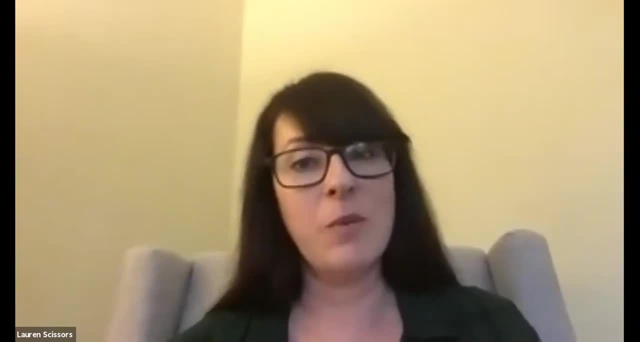 that there were a lot of cases where giving a like just didn't feel right. It wasn't allowing people to express the thing that they wanted to express. So we were solving a real user need. So it felt like a good pursuit, not something that we were doing, you know, for a different. 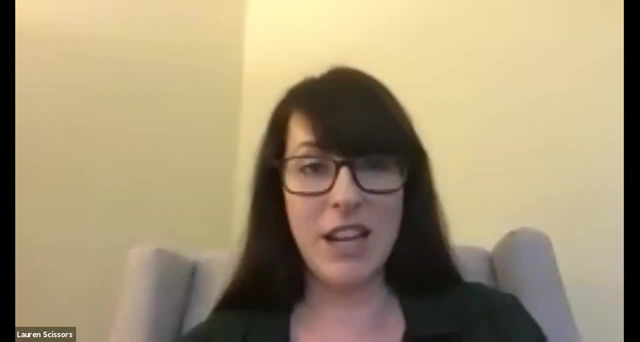 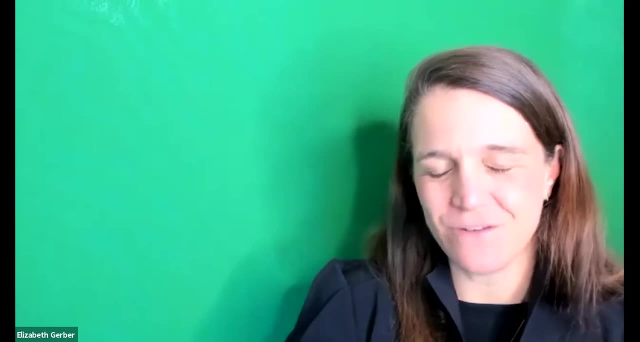 benefit. So you know, that was early on in my time And that was pretty, that was pretty exciting And it sounds like you worked with a diverse group of folks to get you there as well, from psychologists to- I mean, tell us more about the folks you worked. 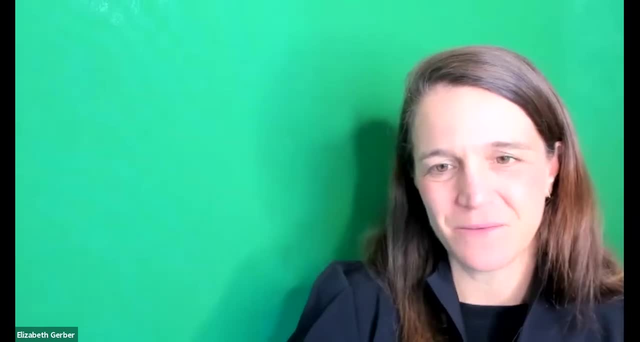 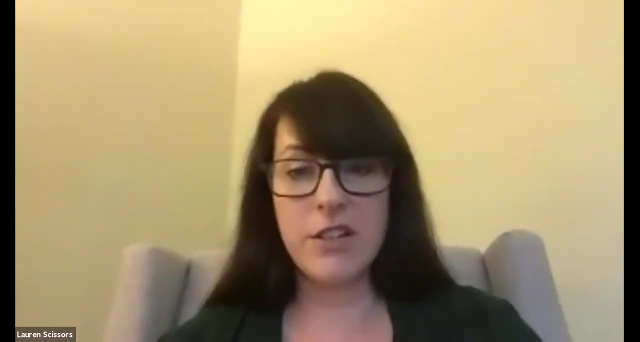 with to realize that feature. Well, I think you know we worked with design, So I'm in the research side. We worked with designers, product managers, engineers, data scientists. We consulted a lot of academic literature. We looked at, you know, the state of the art that was out in. 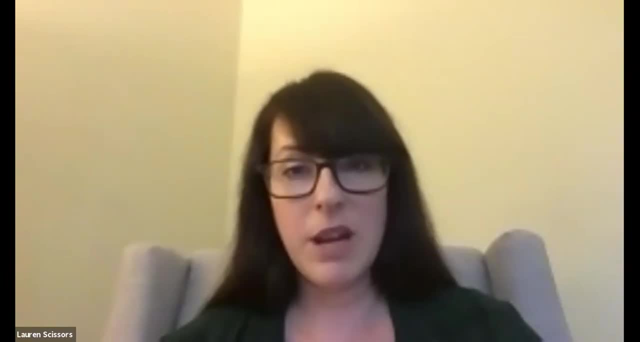 different platforms. at that time, We tested in a lot of different countries. We tested in a lot of countries. We did all sorts of different- you know- research methods, because we knew this was going to be a big change. So we wanted to get it right. And yeah, it was really. it was a good. 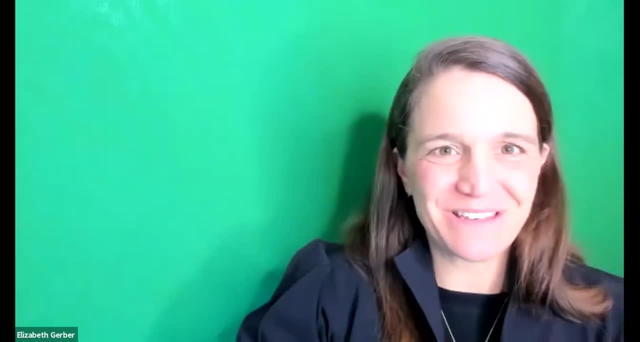 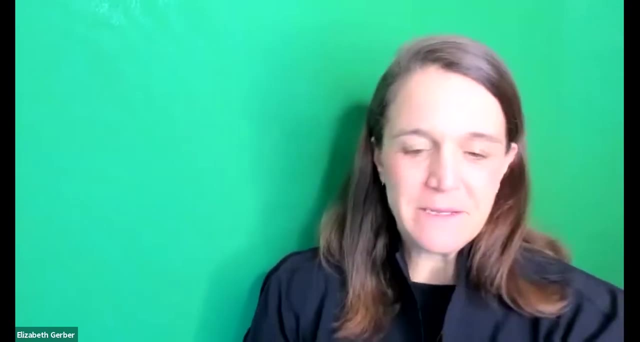 experience. Thanks so much, Lauren. I appreciate the specificity And I think how much those- even that way of communicating- is translated into so many other products we now use as well. I tried to resist giving you a thumbs up when you were talking. Thank you for making that possible. 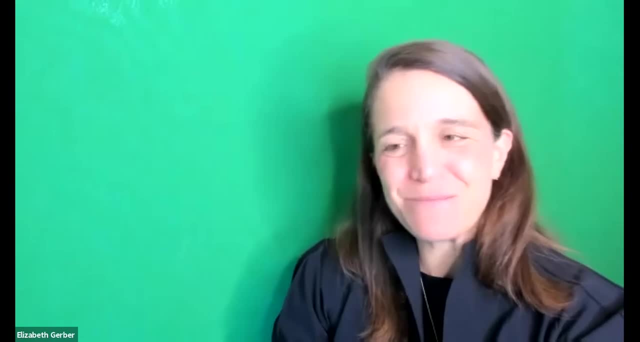 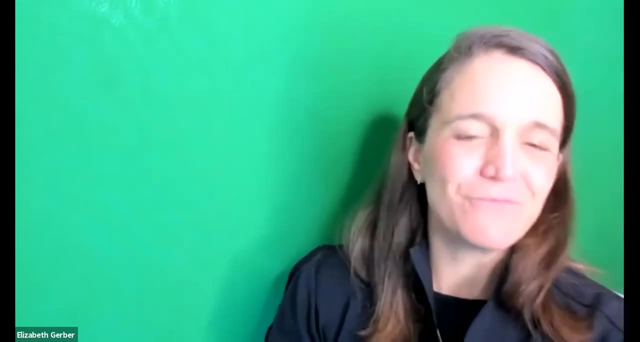 My next question is one of the things- and Mark hit on this a bit earlier, but it's really around the naysayers, So the folks who say, no, that's not really a grand challenge, We don't really need to broaden. 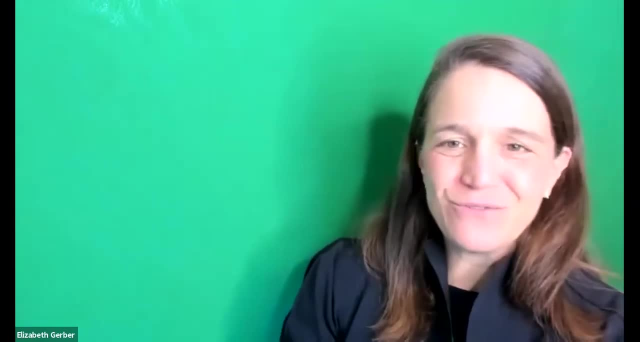 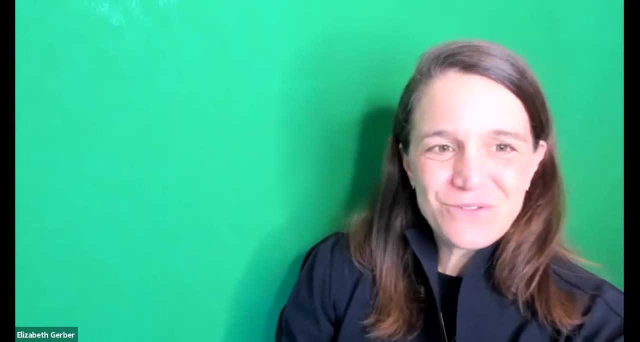 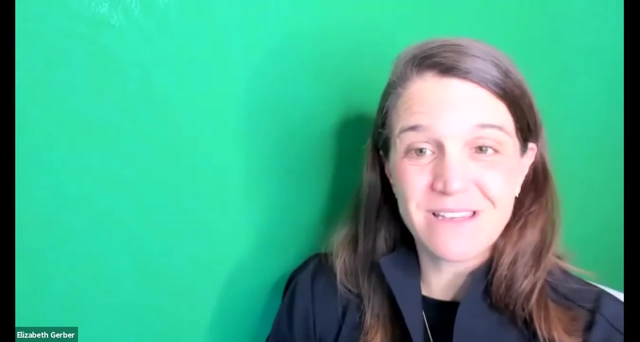 participation. We don't really need to scale. We don't really need to address language equity. We don't really need to get people to look up from their screens. What strategies do you use to overcome those people's perspectives and continue your work, Or do you just ignore them and walk on? 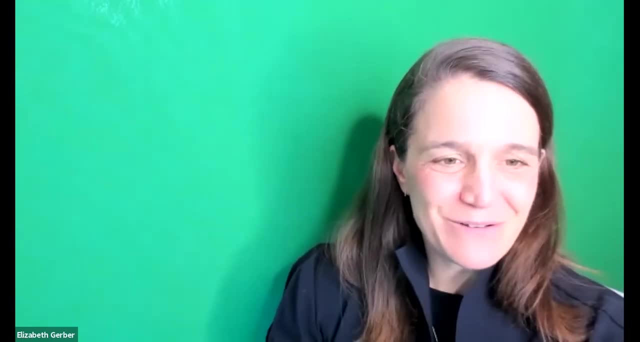 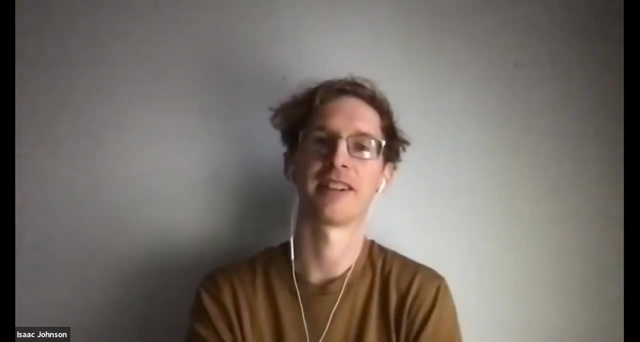 Love to know. Isaac, do you have? you're smiling, so I'm going to assume you have a thought there. I was going to ask whether we're allowed to answer that We can ignore them. I think I mean, honestly, sometimes that's the correct way to go because, yeah, you don't have. 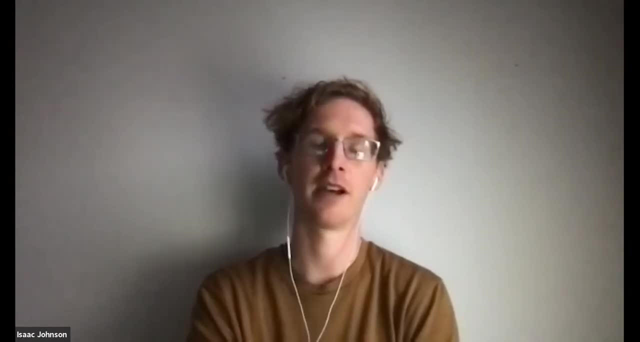 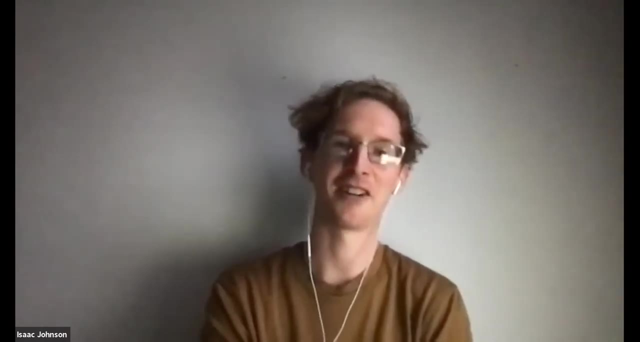 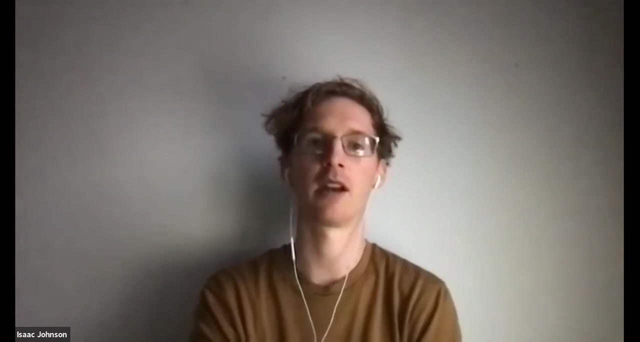 to convince everybody. You just need to convince enough. So I think that's actually a very valid answer. Otherwise, I mean, we're researchers, so try to gather all your data points and make some sort of- you know, make some sort of reasoned argument for it. And you know, I think that's valuable, just to make. 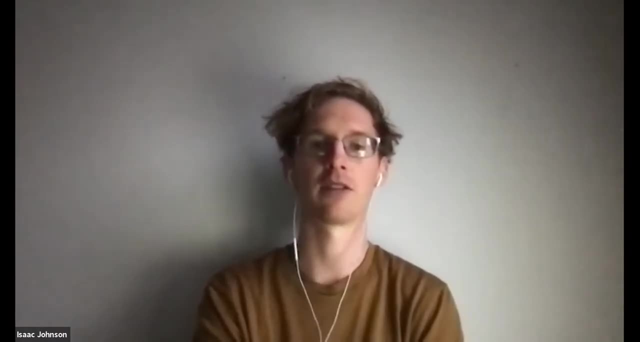 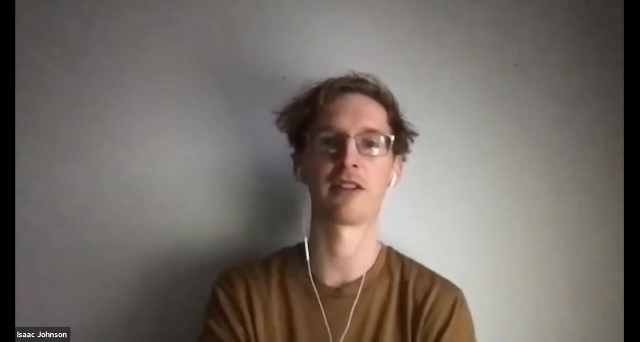 sure you have your own ducks in order and can you know answer to yourself to why you also think it's important? But you know, try not to waste too much time on just trying to convince everybody. And honestly, you know, demonstration goes a long way too, Like you know, if you want something. 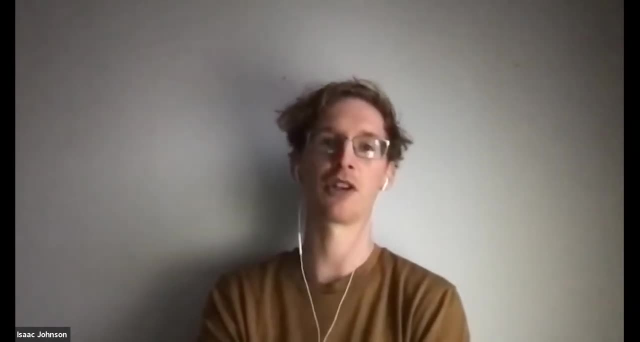 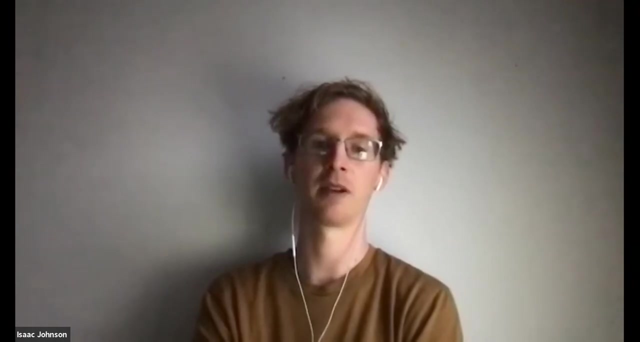 to be done and you think it's important, try to do it. And once you can show people like here's a prototype, or like here's- you know, here's a success story- you'll have a lot easier time convincing folks that it's worth. 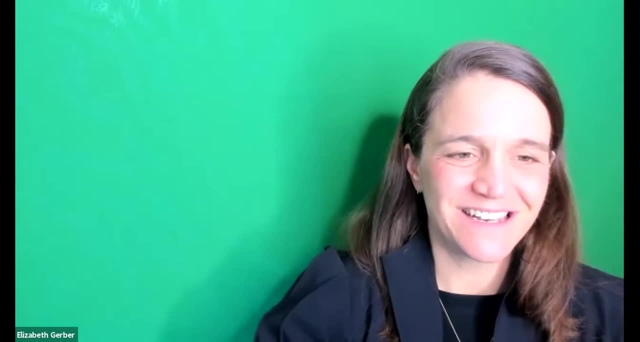 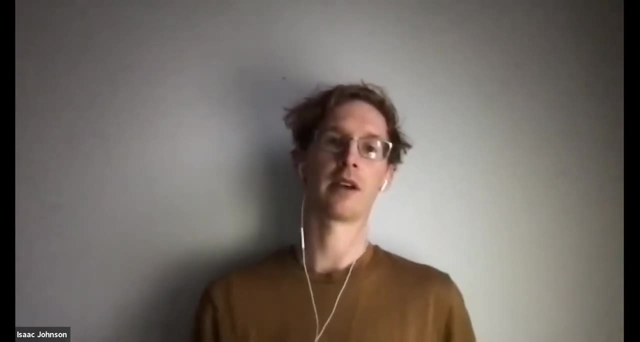 pursuing. Do you have a concrete example to illustrate that? Isaac, Yeah, sure Like especially around language equity. when the foundation was building a lot of kind of our original machine learning model, the state of the field was very much kind of. 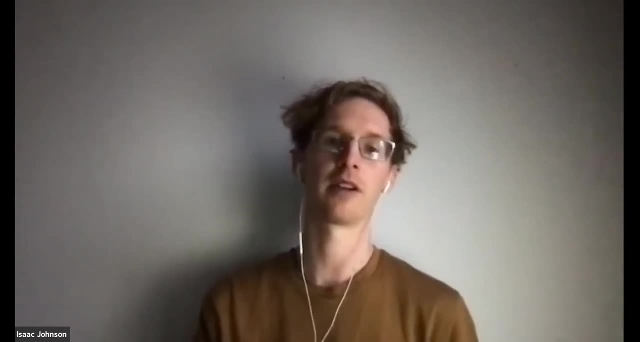 you know, you build a model for English and then you think about building a model for another language And with some of the stuff that we were doing, for instance, we have a model that's just like take a Wikipedia article, like label it with a high 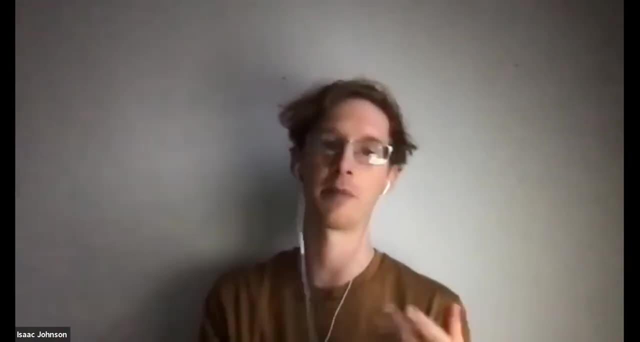 level topic, you know. but Mount Everest it's like, oh, it's about sports, It's about geology, Nepal and, you know, China, And so I was able to go in like and build models that were like. 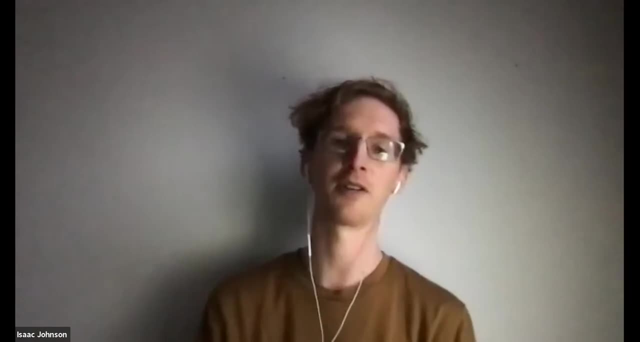 okay, we can do this in lots of different languages, you know, and I'm not going to go into all those details- but like we don't have to do this language by language And by being able to kind of prototype and show people like, hey, this actually works quite well. 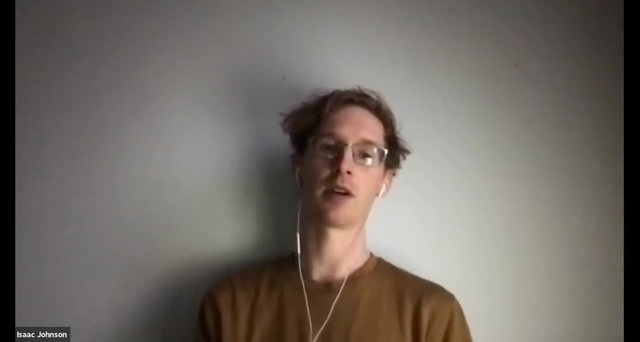 like and we get much higher coverage, was able to build a lot more kind of momentum around. oh, maybe we should take a step back from the way we've been thinking and approaching a lot of these designs of like. let's see if we can do this in English and then think about building for. 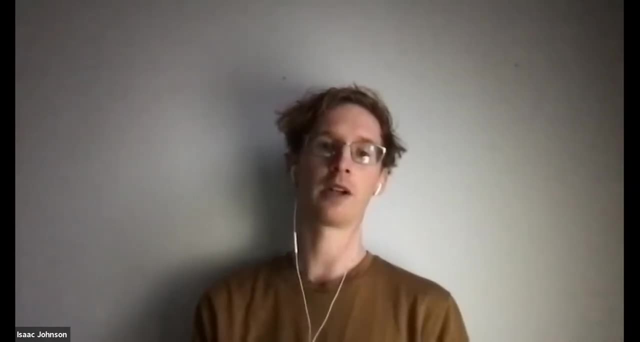 other languages and kind of take that step back and say, okay, what would it look like to build this for all languages? And then maybe think about, you know, narrowing down and kind of fine tuning for other languages. Thank you so much, Isaac, Thanks for. 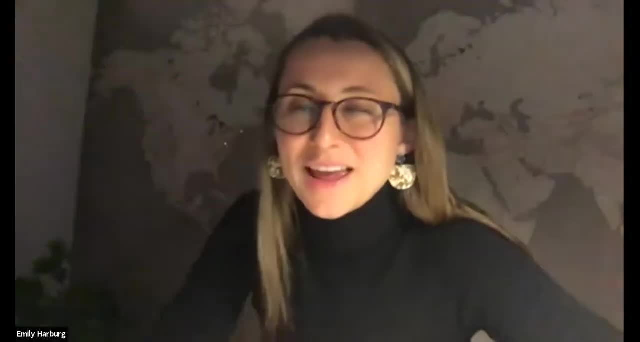 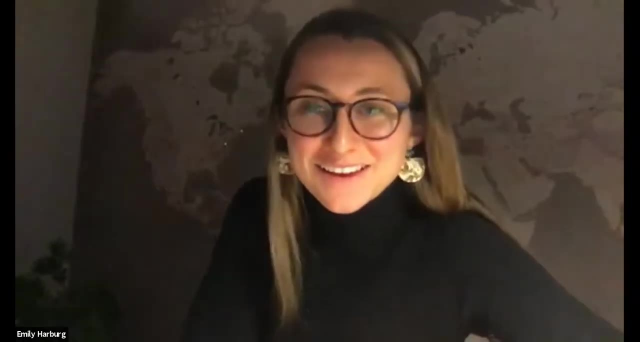 the specifics. Emily, did you want to jump in? Yeah, sure, I would echo all that. I think we have really found that having like stories and even like having a voice of a customer saying you know their thoughts around something has been so helpful. I know the data has been super. 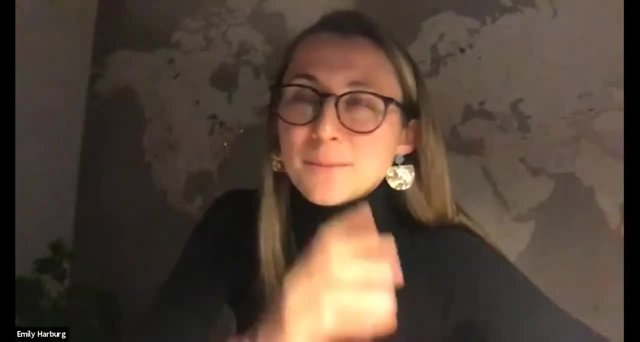 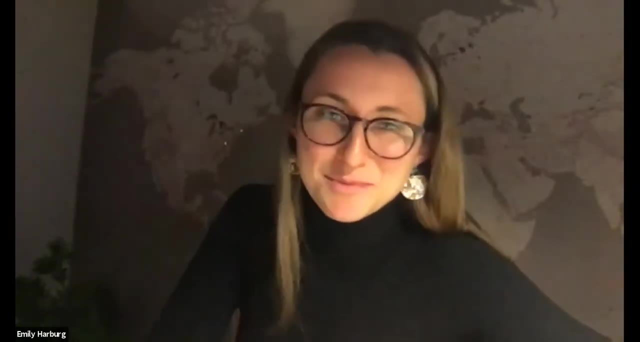 helpful but, like I remember, as a specific example, we had this video of a teacher just talking about how much she hated their students being on their phones all day, kind of sitting at McDonald's when they were in France and couldn't go exploring. but we're all. 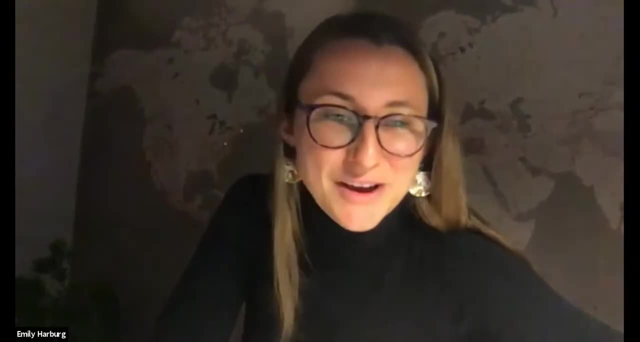 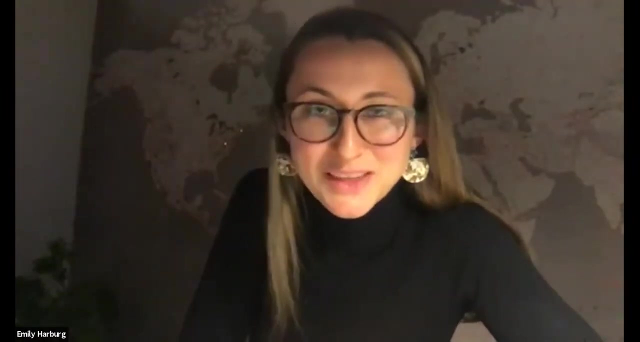 on Wi-Fi sitting in the hotspot there And so and we just always kind of like would think of her and like start a lot of our presentations with her kind of talking, And so I do think having sometimes a voice or a story or a face can make an issue even more personal and real. We've also 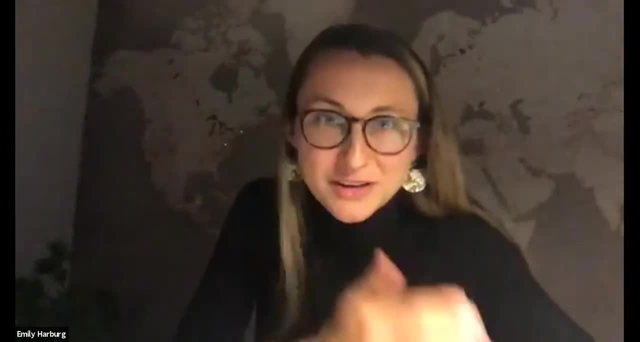 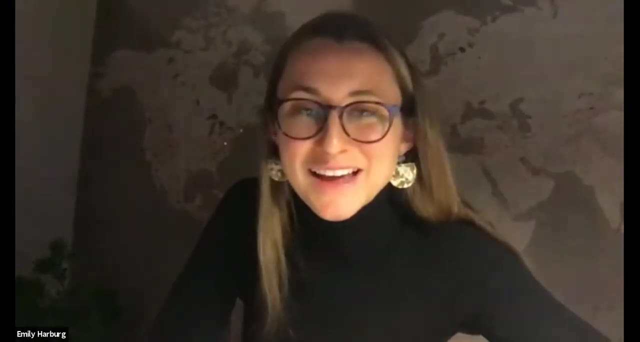 had similar ones around, kind of supporting accessibility on the site and having some voices of some of the customers who've gone on and can't see what we put out there and the options for them and that kind of thing. So I do think like a combination, usually for us, of really 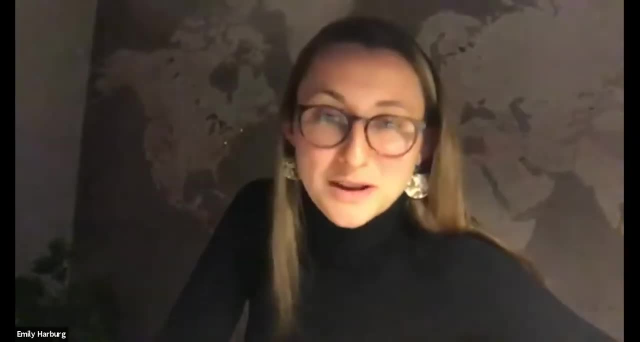 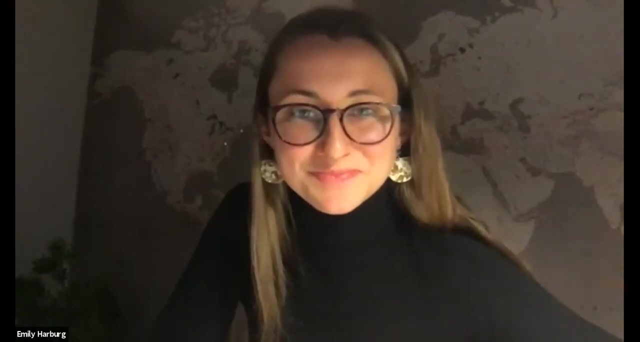 having good data showing it And- and usually that's you know- quantitative data showing the numbers, but also having a face or a voice to make it really like human and personal has helped us. That's great. I love the vision of a teenager looking at their phone in the McDonald's in 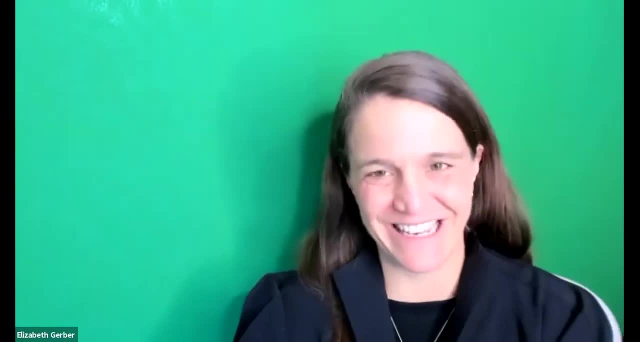 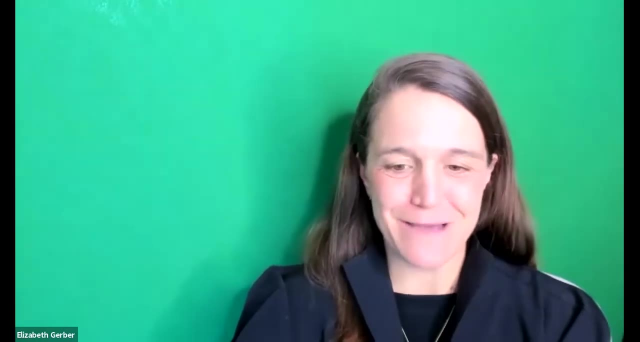 France. I can. I've seen that before. I can relate Absolutely. That's lovely. We're going to switch over to audience questions at this point. We've had a lot of great ones coming in, And so I encourage the audience to go ahead and put your questions in the chat box And, if you have any, 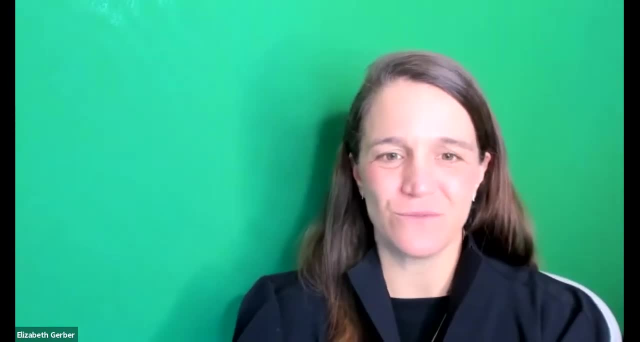 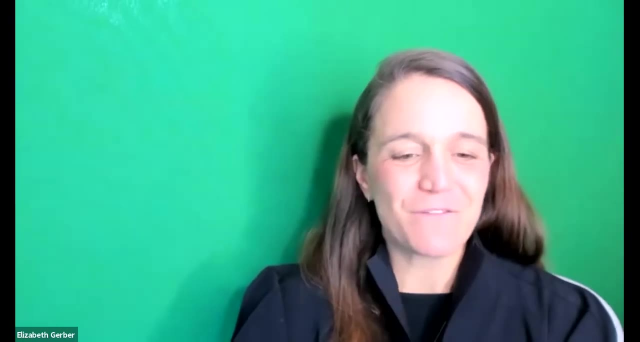 questions for the audience. please put your question in the Q and a if you like, and we'll we'll aim to get get to it, And the questions really range the gamut, So we're just going to going to jump right in. The first one is directed specifically at you, Isaac, which is a question. 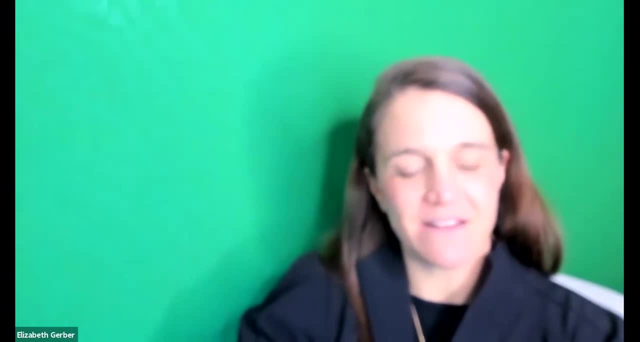 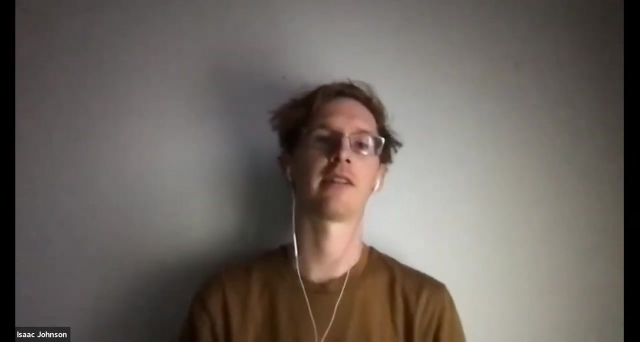 around. have you seen growth in languages as Basque and Catalan, And does it correlate with the desire for independence? So I think this is a question around language and politics, as it plays out in Wikipedia. Sure, So Basque and Catalan, for folks who don't know, are languages spoken in kind of Spain, that area. 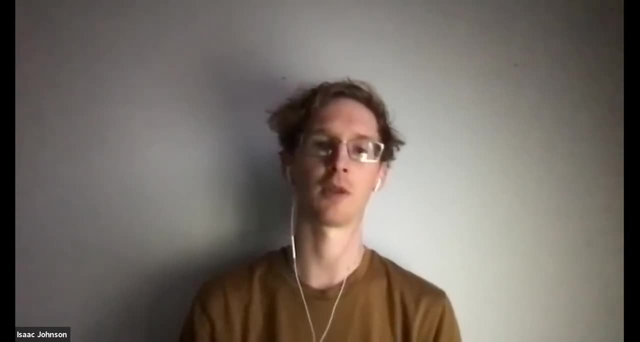 And they do have separate language editions on. so there's a Spanish Wikipedia, there's a Catalan Wikipedia, there's a Basque Wikipedia, And Basque and Catalan have been around for a while- almost this long, you know, since like 2002 or so 2003,. somewhere in there, I think, Catalan Wikipedia was. 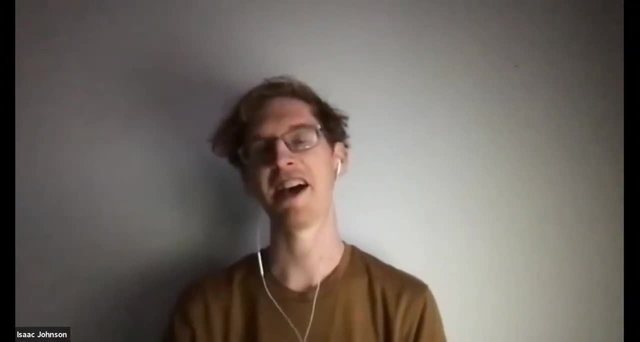 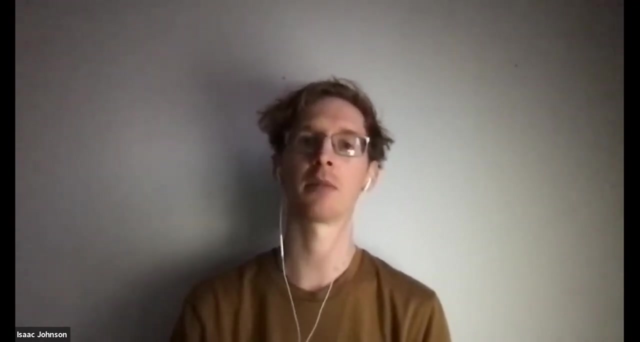 the second language after English, if I'm remembering correctly. And I mean, there's a specifics of whether those- and I don't know the specifics that I answer whether their growth has correlated with politics, but I do think that there's some really interesting. 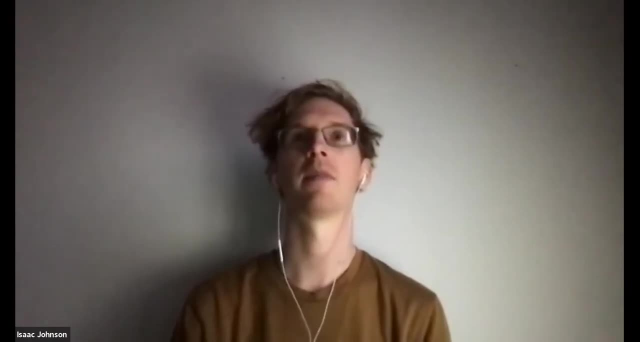 big research questions around what sort of you know offline things that factor into the growth of Wikipedia and like these knowledge communities and participation online. I mean, I'm sure a lot of us have been studying kind of COVID-19 effects on participation and engagement and things like. 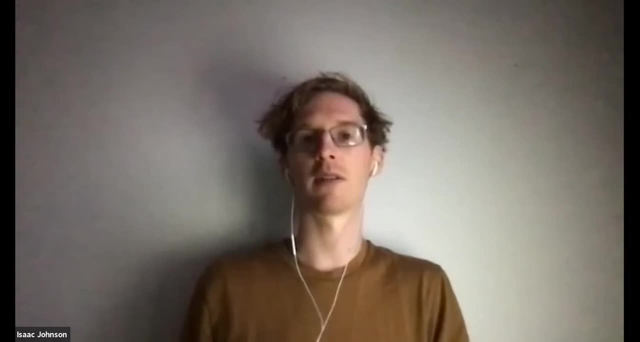 that which isn't, you know the same, But I think there's a lot of interesting questions around same as kind of political movements- It's another kind of huge change and things that then you ask the question: okay, what does this mean for us? And you know, is this a sustained change or is? 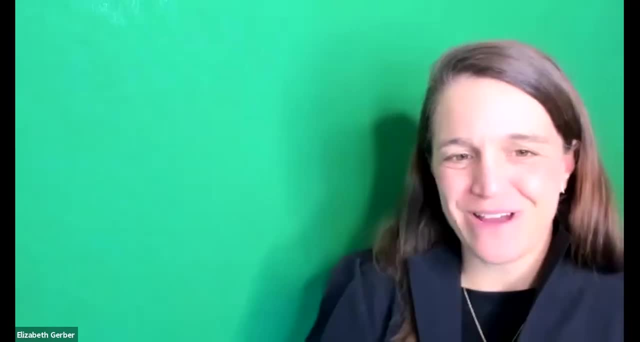 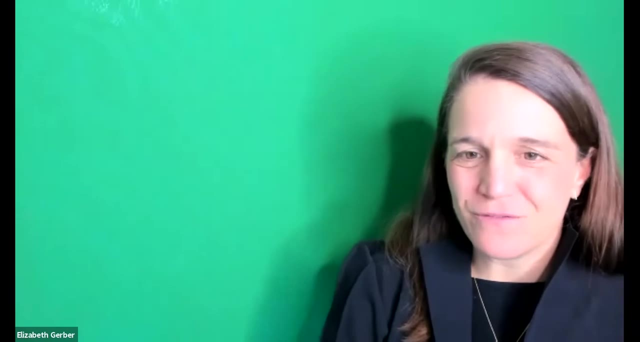 this something smaller. That's great. Thank you, Isaac, very much. This next question I'm going to direct towards Mark and Lauren, which is, if you're trying to build for people who speak different languages- or perhaps nobody on your team speaks that language- how do you handle the? 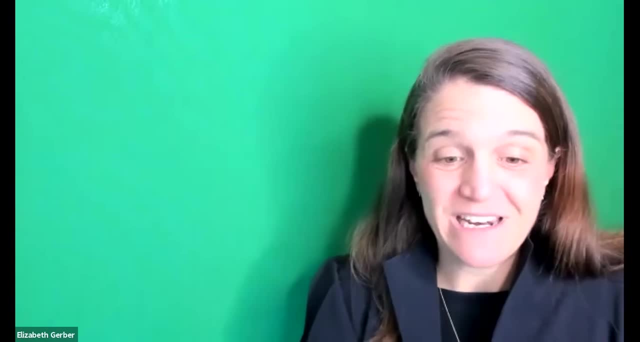 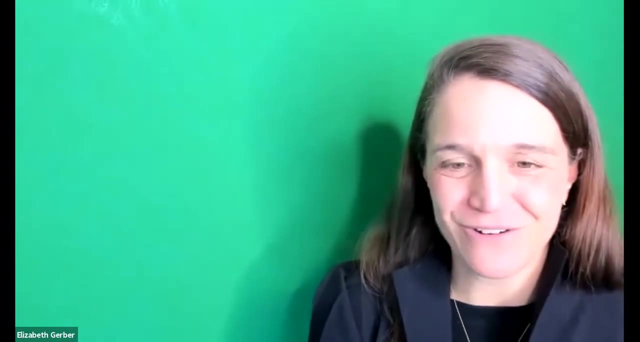 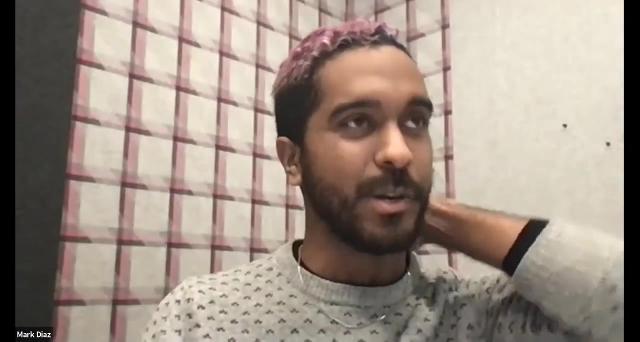 challenge of knowing whether it's working and if people are using it in the way we want them to work. So, as we're trying to broaden participation, this means a lot more language. I'm curious. I'd love to hear Mark and Lauren's thoughts on this. Yeah, happy to quickly say so. one of the 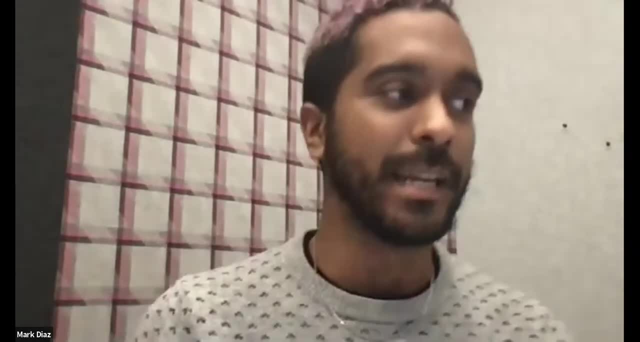 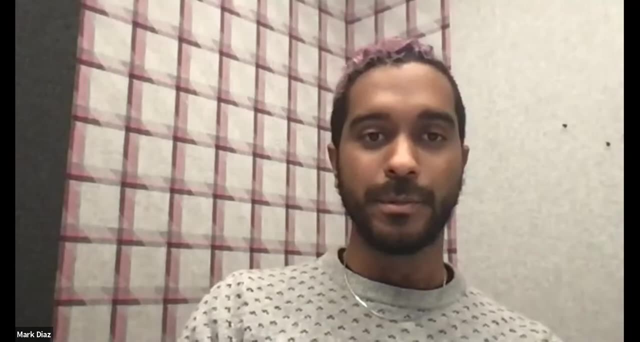 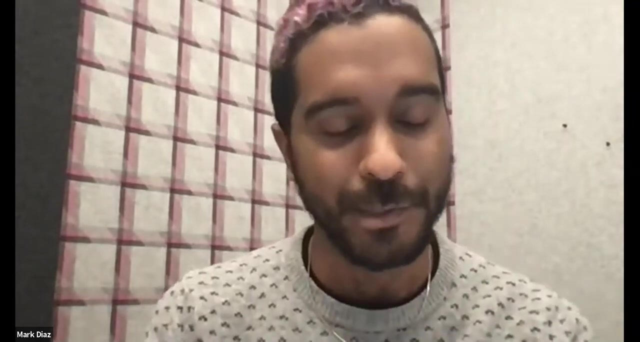 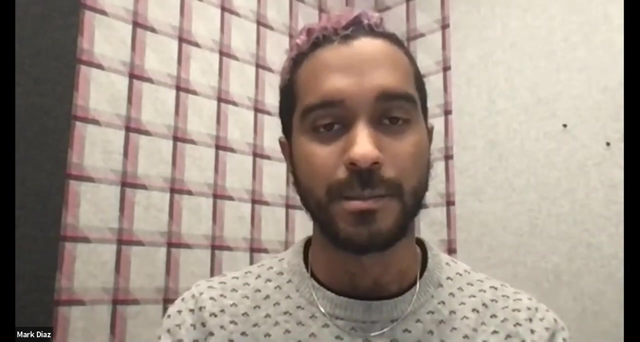 things, I guess, on different time horizons, like in the longer term, one of our approaches is hiring people who speak those languages- At least I can speak for my team and area within the company, which is massive. But there is still the very practical problem of wanting to support and develop systems now And currently the way. 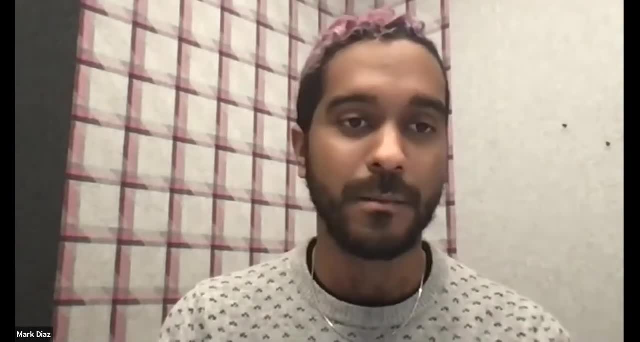 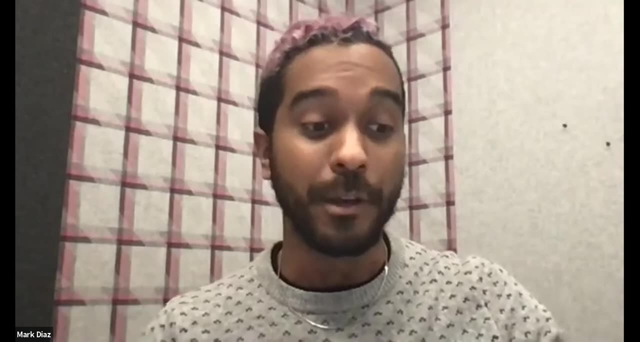 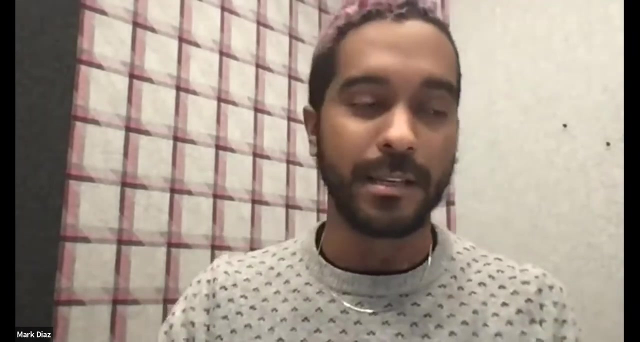 that works is a lot of like contracting with people who, which isn't ideal, I think, primarily because you're looping in people at the evaluation stage of systems and not taking into account their needs from from the outset. That said, I'll say that a lot of my work involves not just convincing. 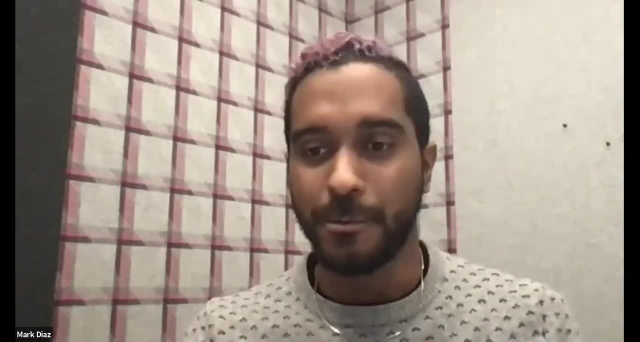 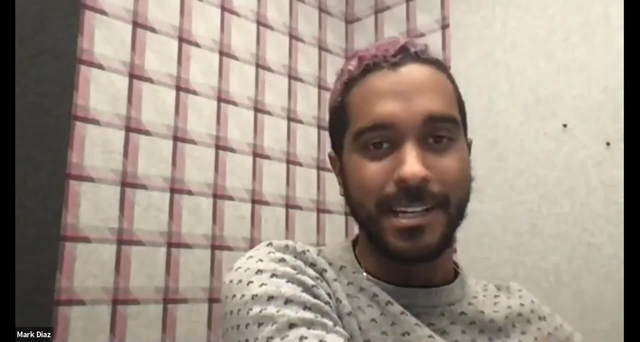 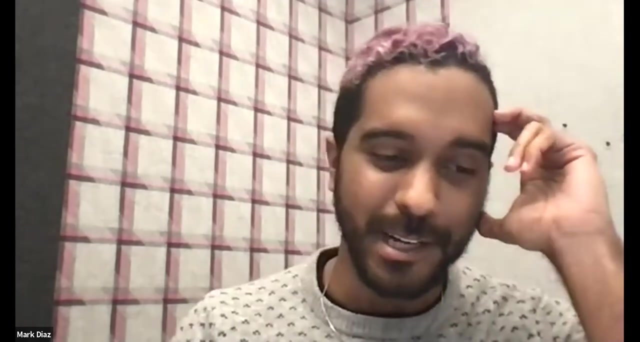 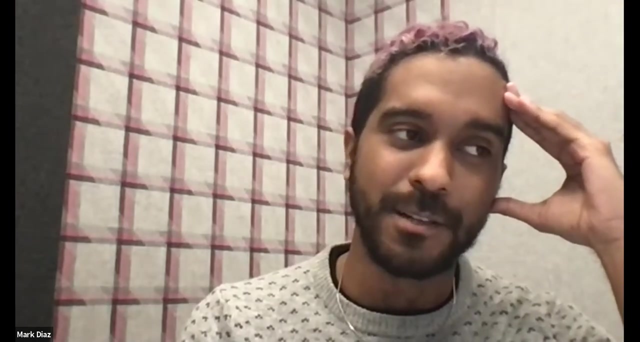 people of the importance of running participation, but also broadening participation earlier in the design and development pipelines. So I think something excited earlier for any exact words, but just like demonstrating to people is super, super important. I find myself currently So. Google a couple months ago, announced a sort of reorganization. 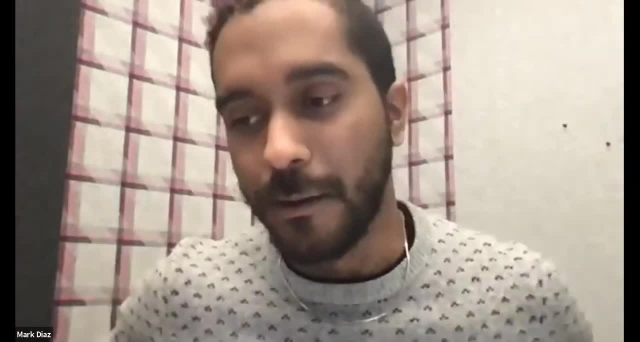 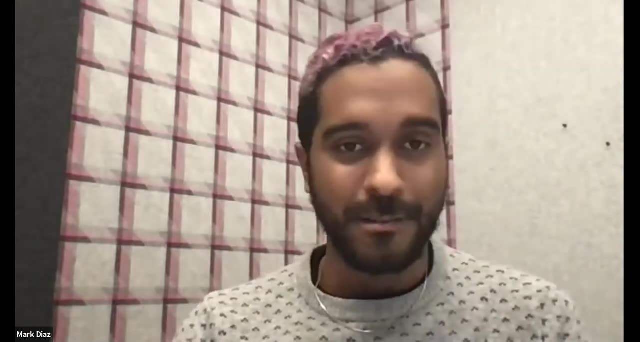 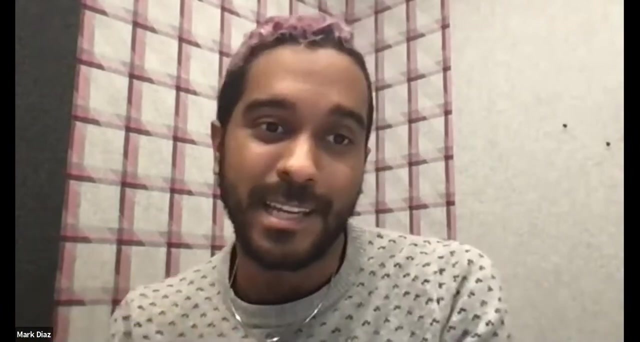 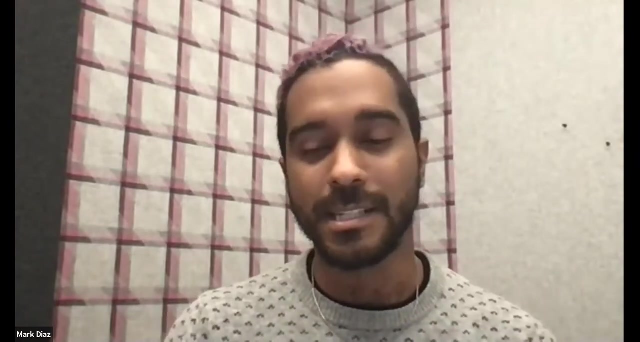 where we have this like responsible AI division And a lot of our work right now is like jumping in and sometimes getting up to speed at like at a crazy pace, to work with some teams to show that, hey, we can, we can help you do this thing, And we had so little time. Imagine if we did this from the beginning And using that as like currency. 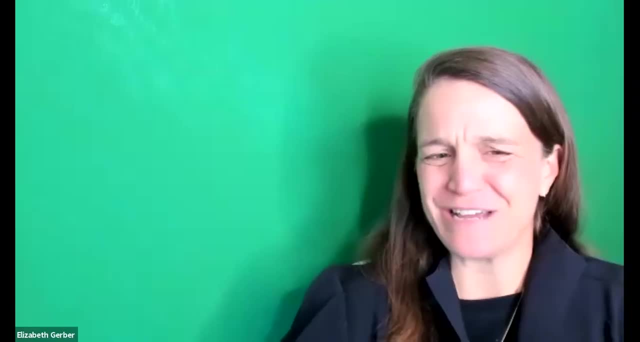 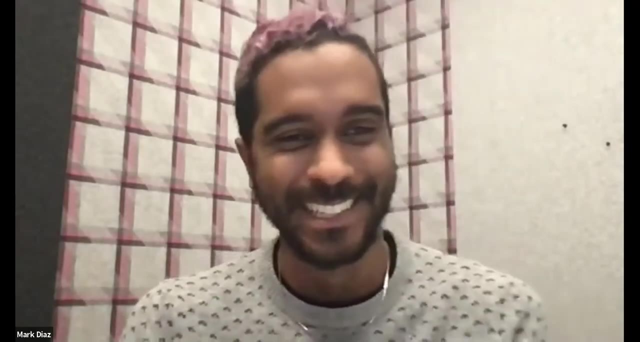 Yeah, so you have a concrete example you can share that mark, or Oh, uh, maybe not. So thanks, Lauren. Do you have anything to share on this? Lauren Poggiatiere? Yeah, so very concrete level. I mean there are some heuristics, that at a bare. 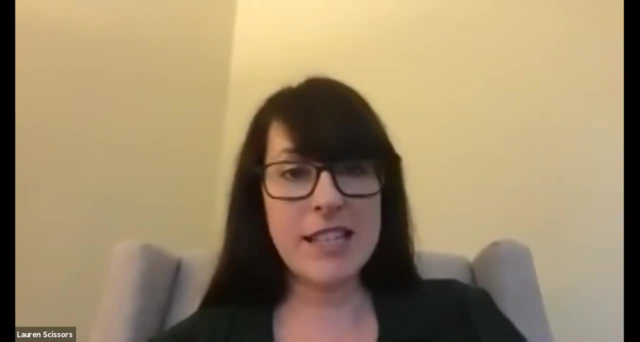 level. there are some heuristics that at a bare level. there are some heuristics that at a bare, bare minimum, folks can do so. for instance, um testing things out in a left to right language if you work at a company where you are designing and functioning in a, you know, right to left. 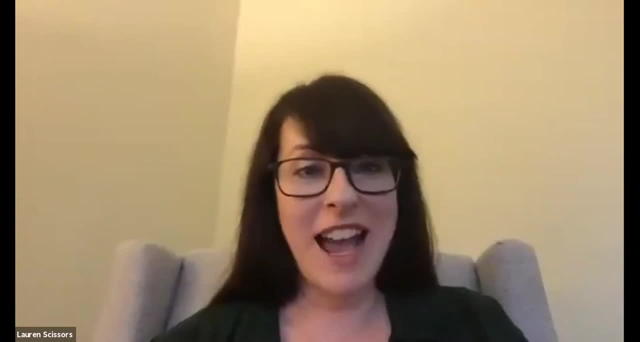 language or things like that. um, german had some really really long words. so a lot of times we're like, what does it look like in german? and we're like, oh, it looks really bad in german, like maybe we should change our design. i mean, those are very practical, like bare minimum things you can do. 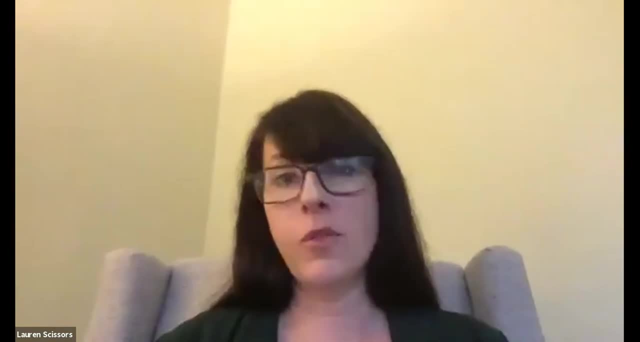 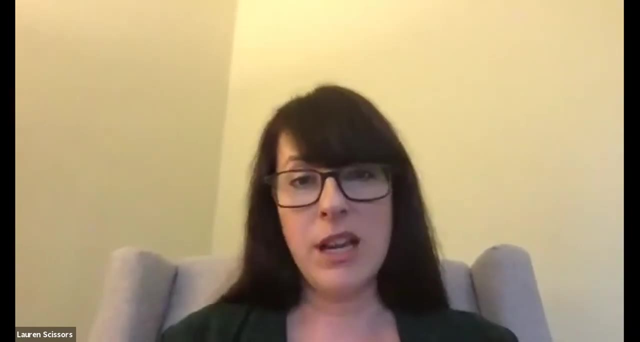 i think at a higher level, though. um, before the work even starts, you have to ask yourself as a team, how are we going to define success, uh, which could be some sort of goal metric, or could also be, uh, an absence of a bad experience, and so there are things that you can do to kind of uh hold. 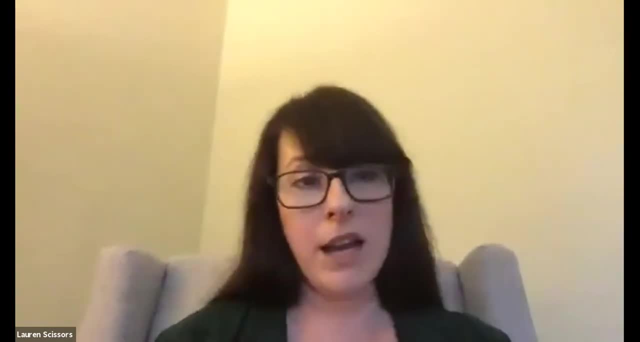 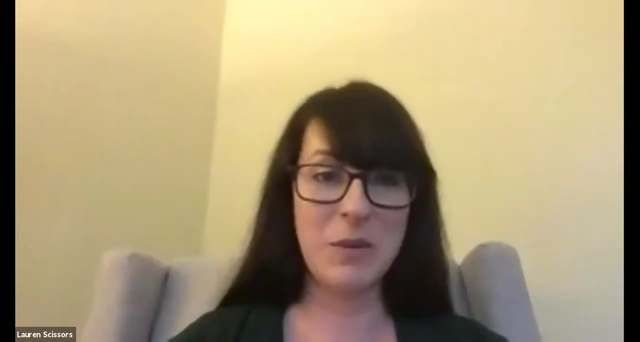 yourself accountable and to try that out. so you know, i i agree with mark like hiring plays a role. um, we're lucky enough at facebook to have a really uh large employee base where we can actually find people for almost every language who speak, or native speakers to say: hey, can you take a look at this? hey, can you, can we run this by you? there's a lot. 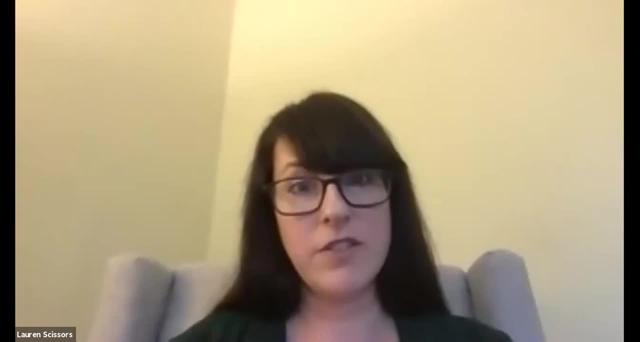 more things that you can do and you can take. you know responsibility for, for defining success and and having people help you think through. you know how should we define success, both in something added and making sure we're not adding anything negative- and then hold yourself accountable to. 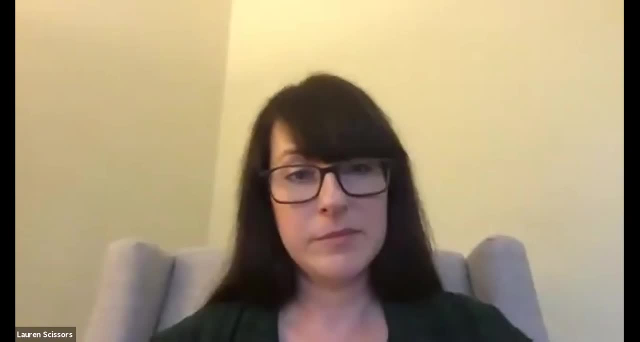 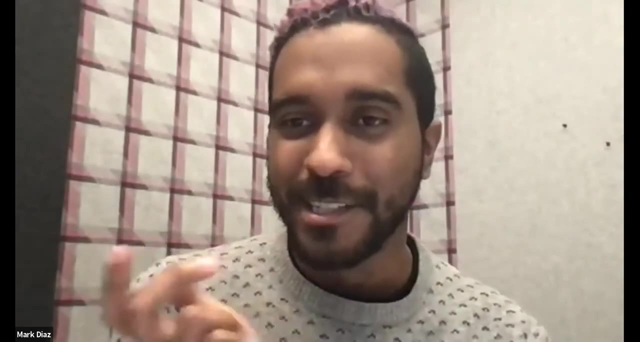 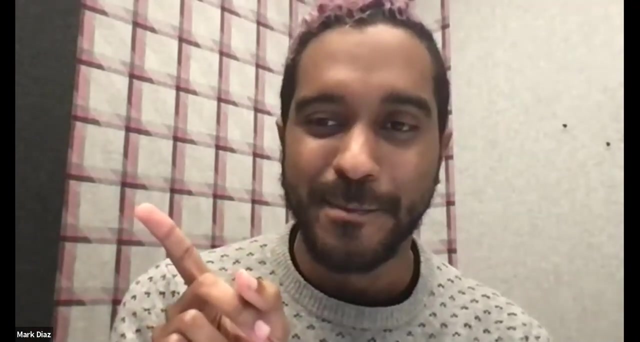 that you. thanks, lauren. i appreciate, mark, go ahead. i wanted to jump in. i was really curious, um, because i'm realizing i was looking at one of the questions. um, i wanted to one shout out: minsook, uh, your question, um, i have a lot of, a lot of, a lot of. 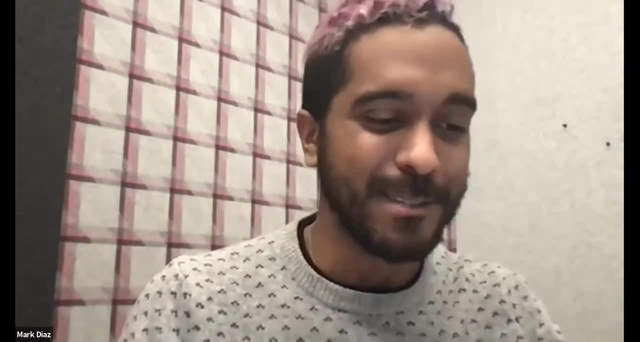 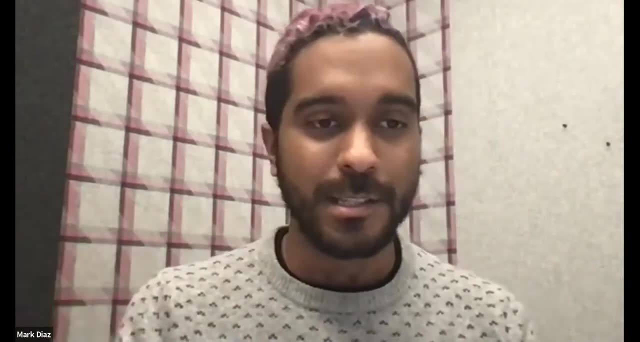 thoughts on that. um, so i just wanted to like flag that. feel free to reach out to me at some point, but um, in sort of in that question was this um note about like, whose participation? and so i was kind of curious for what the range of like. 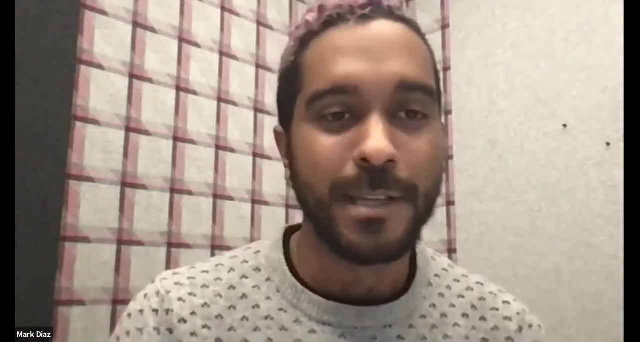 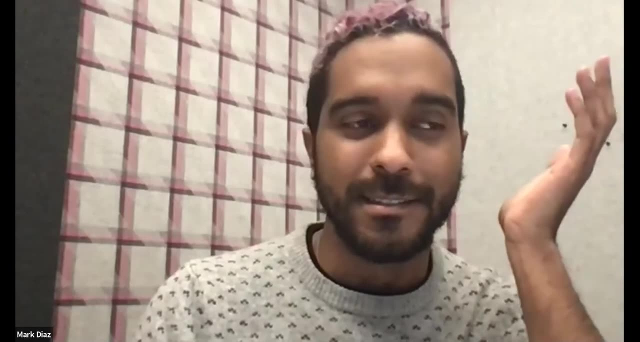 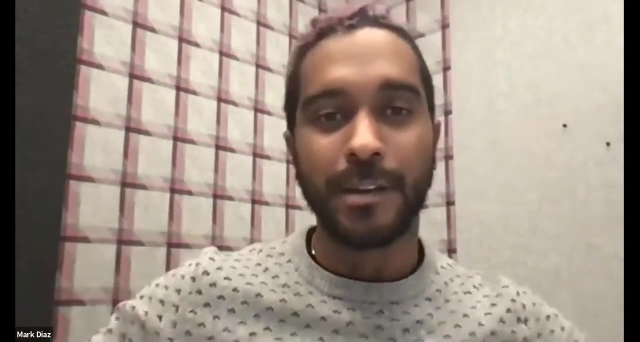 other other people, i guess, other than the researcher- participating looks like for different folks um, in your work, um when, like for me at least, to that's rude of me, i'm putting the question but i'm answering it first. but, um, i first think about like disciplinary participation, um which, fortunately, there's a lot of room for on. 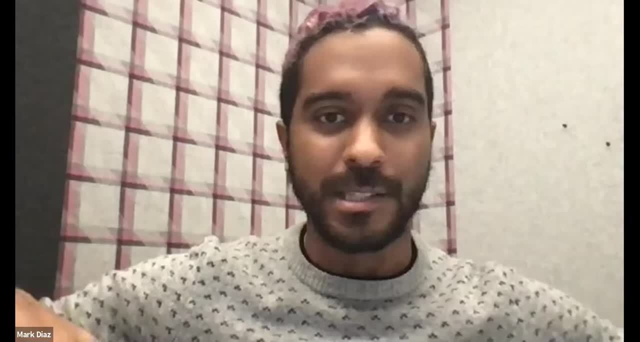 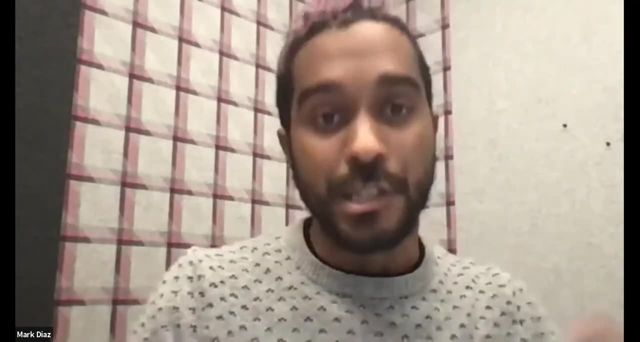 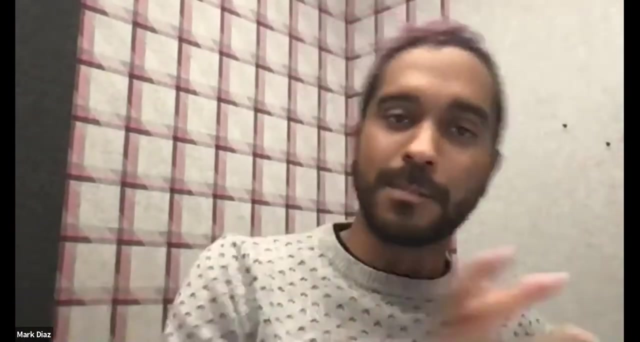 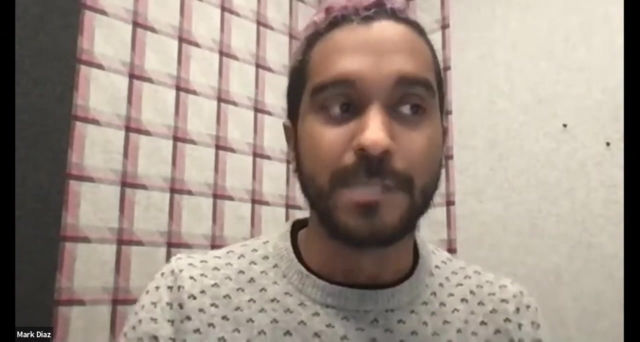 my team, my um boss is a sociologist, we have an anthropologist on the team um we have nlp researchers um in addition to like the user side of things and the people who would be using systems. so there's this like disciplinary bit and also um like non-tech worker user uh experience and 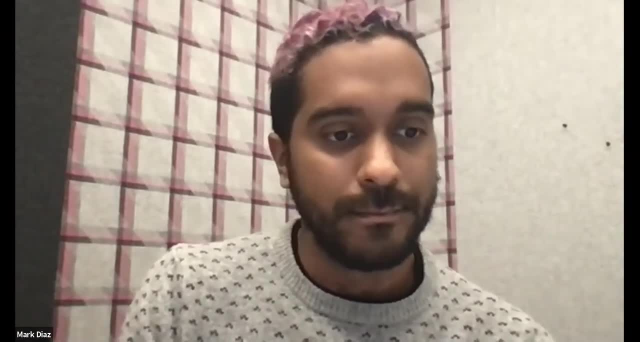 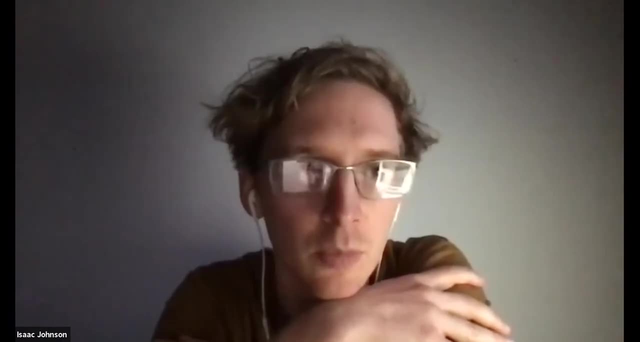 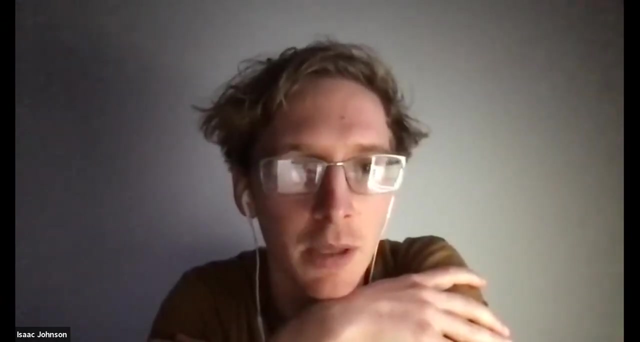 expertise. i would say i can, i can chime in on that. um so uh, we do a lot of things like very transparently to the like point of our work. so, for instance, like the tasks i'm working on are public and anyone could see those and like see my progress on them and go in and like comment on. 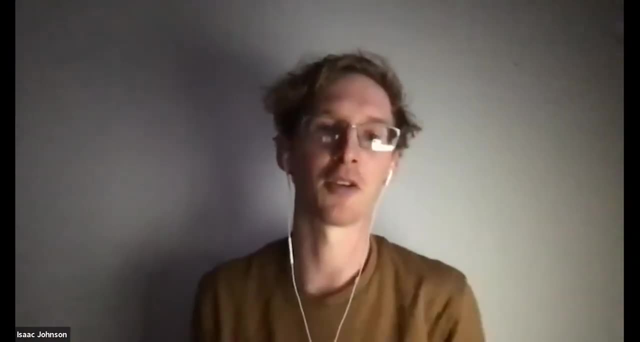 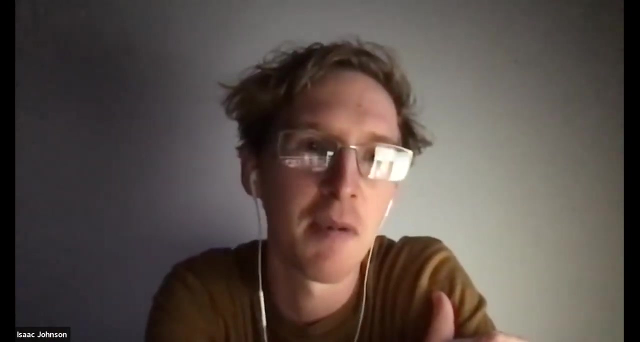 them and because there's like this huge community of editors who are really interested in a lot of these things, like people actually do go in and say like oh, i see that you're thinking about it this way, but like let me point you to this example: um over here and we actually, you know, 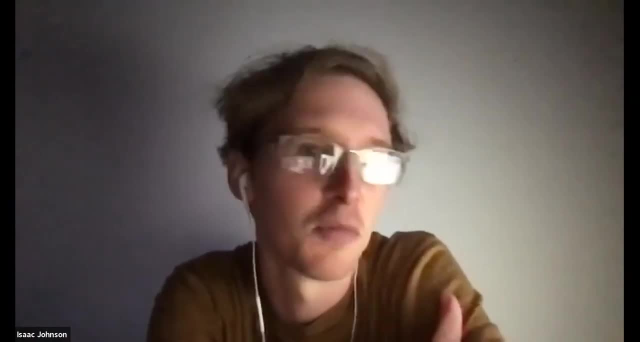 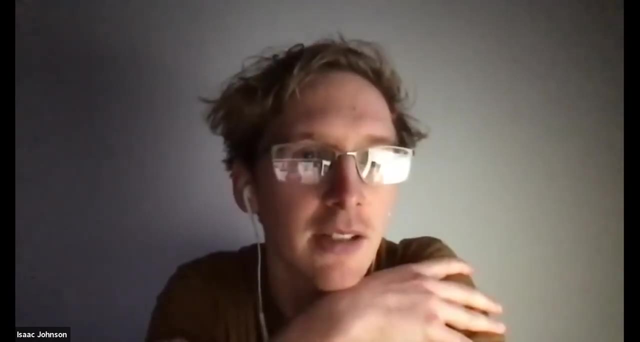 get a lot of and that sounds like chaotic but actually well in practice, um, and then we also have like community conferences that we attend and so talk to really engage kind of organizers and editors in the space and really get to have these like close conversations. so i think we're pretty lucky in that we have a- uh, not always a like. 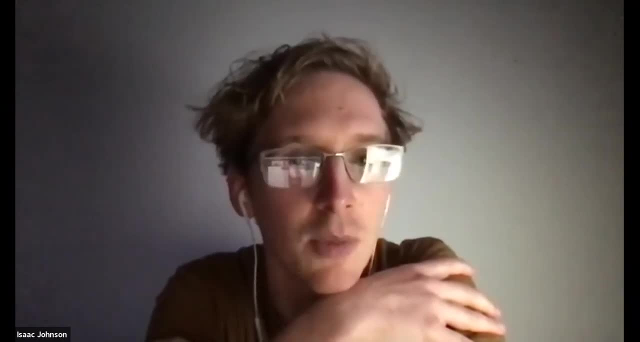 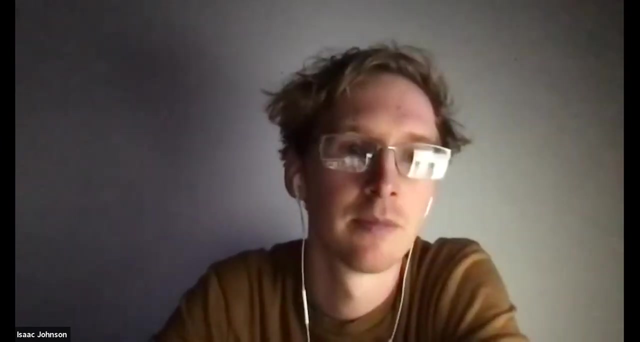 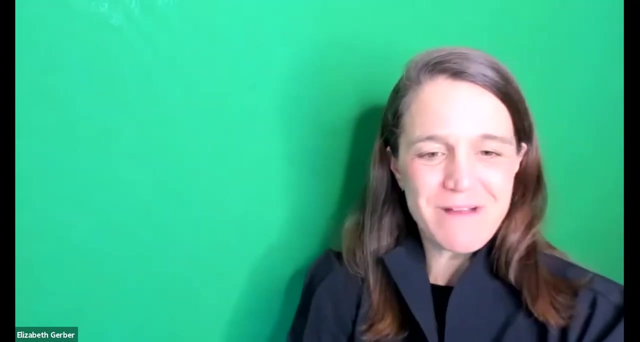 non-tense relationship, but we have a very strong relationship with the communities that we're serving, um, and so we get pretty direct access to a lot of very people willing, very willing to like and fill us in on what they're working on. thank you, isaac. um, there's a question here from the audience which is really around. 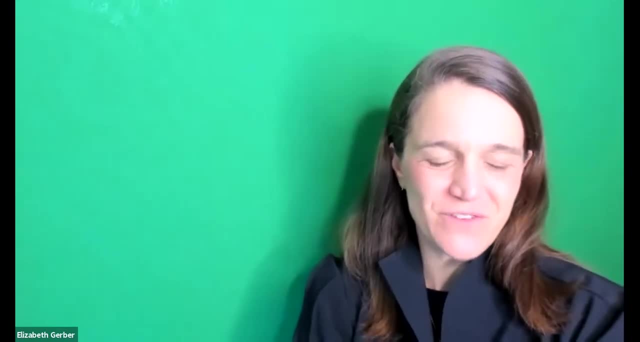 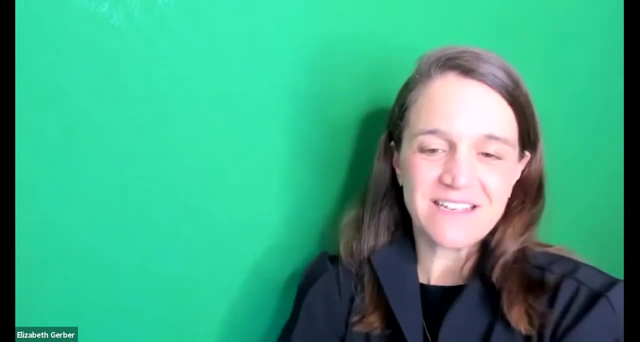 tech culture versus inclusivity- and i'm going to read the question directly. i think it's well phrased: um. so lauren lynn asks: how do you balance the fast mentality of tech companies, um, with the importance of moving, of moving slow, to ensure that you're intentional and inclusive when designing? 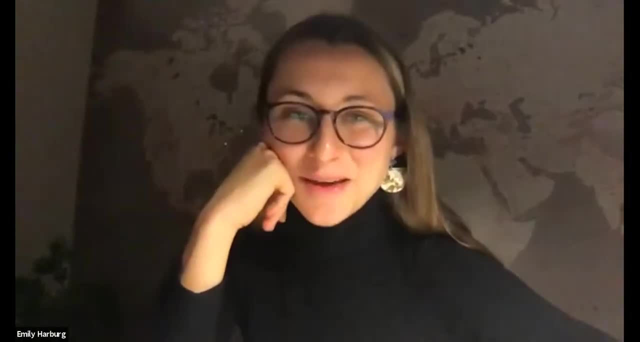 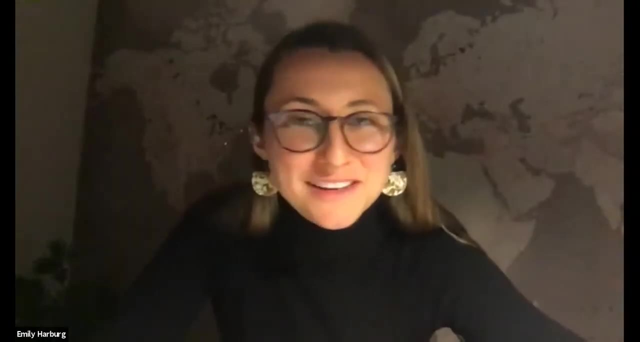 your work and what are the challenges that you face when you're working on your work? i would like to take that on. yeah, i'm happy to start there right. um, i definitely i was. when it come up as kind of the things i like about industry and also miss about academia, i will say: 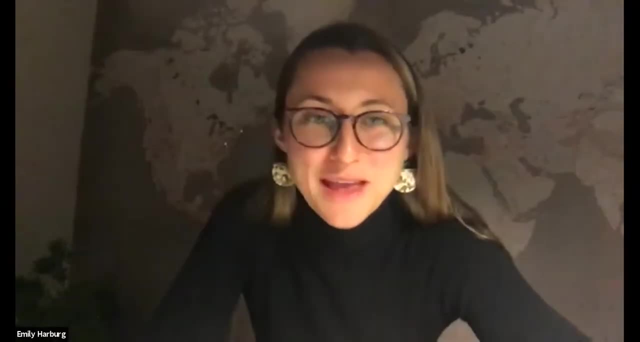 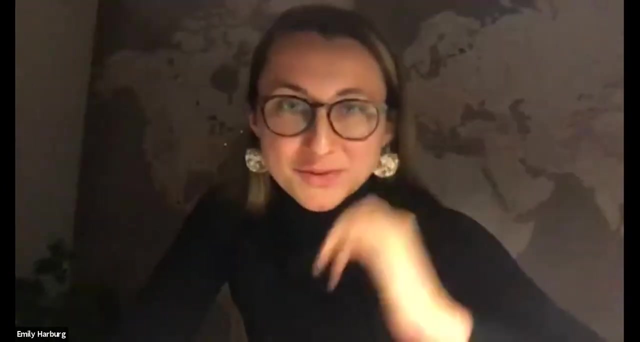 the thing i both love and also find super hard is that we have to move so, so quickly, um and so. sometimes you know we're pushing a feature out, you know without having done much research or and just kind of hoping that it works, or you know and- and certainly in that process a lot of unintended 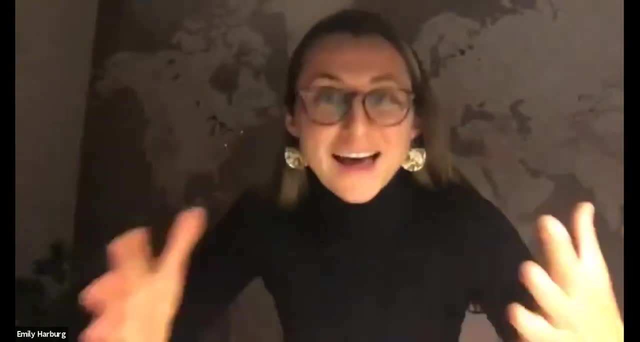 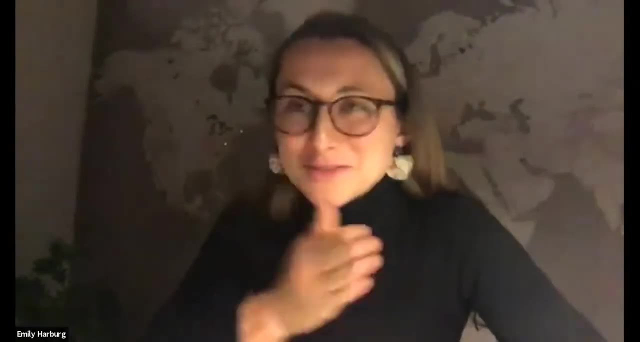 consequences can come out that as a you know, with research and time you'd really be able to kind of work through, and so i do think that that mentality is one that even as a team- just literally today i had a a timeline that we just pushed back two weeks just to kind of give the team a little bit more- 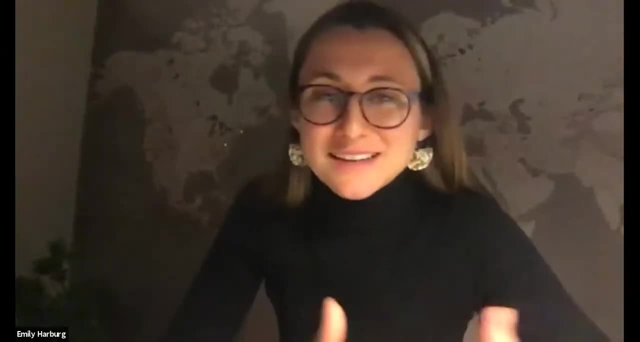 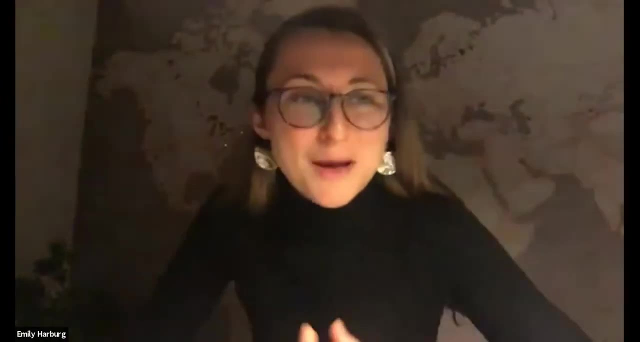 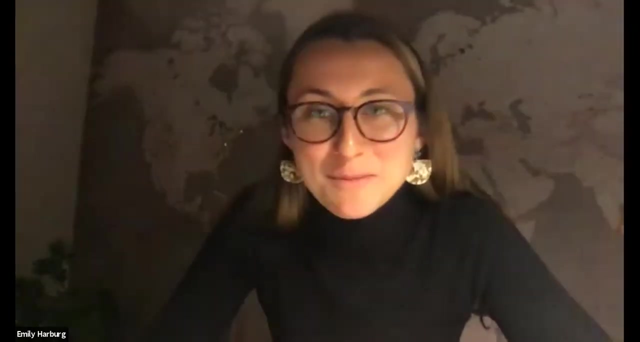 breathing room, the chance to actually like interview customers and get their thoughts about this feature that we were trying to build, and so i think i think there is something i like, such an advantage of coming into industry with that academic mindset and really thinking critically about what you're building, and i i think it's one of the reasons why i believe 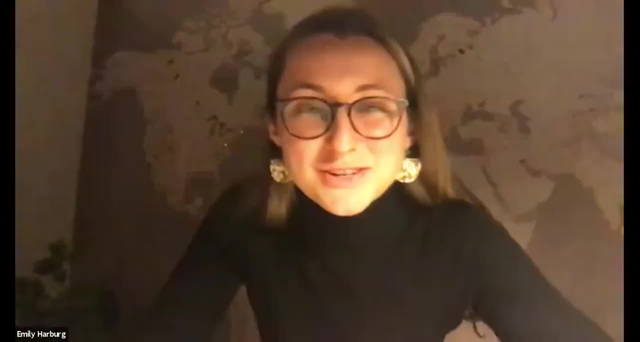 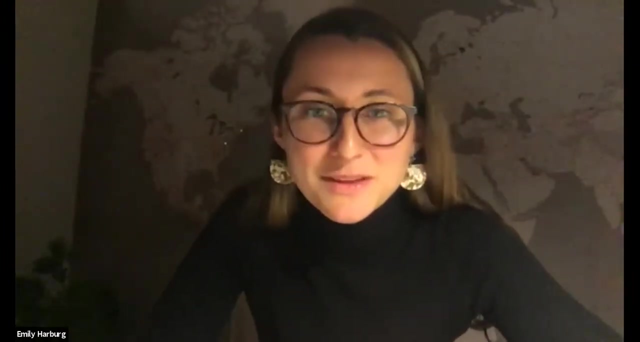 we need researchers going into academia and also, and also, going into industry, because i think, coming in with that mindset of you, know, how is this shaping the, the user, how is this impacting the way that they feel and engage, and i know we, i thought about that when i was at facebook. a. 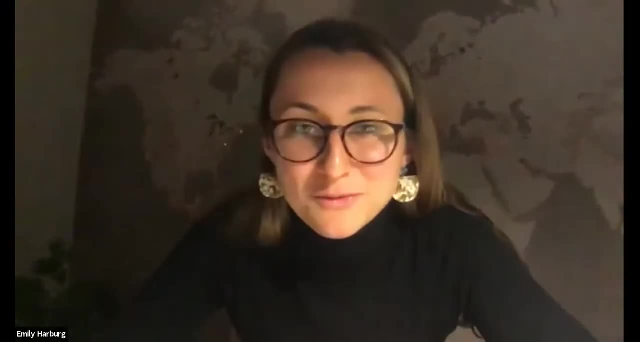 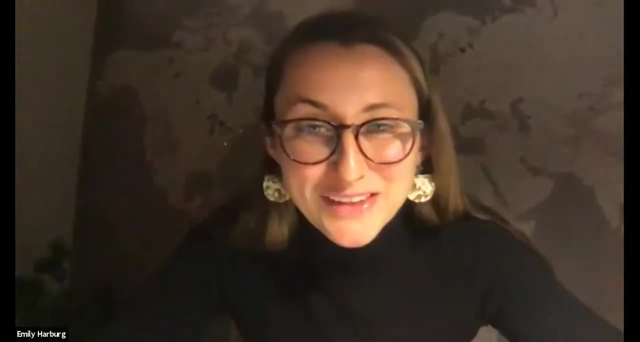 lot of them on the team there too, and i think just that mindset of really you know, the user first or user-centered design, customer-centered design, um, human-centered design, broadly i think changes the way you build. so i'm trying to, at least in my team, slow, slow the team down at moments. 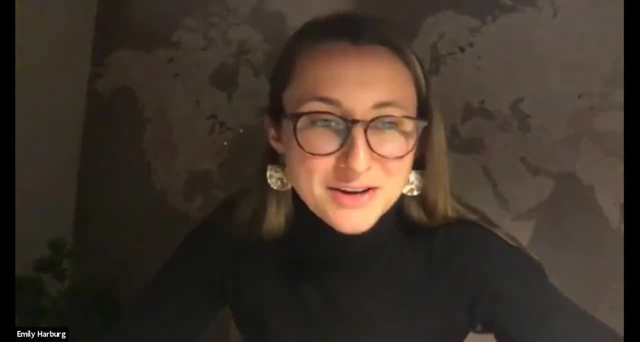 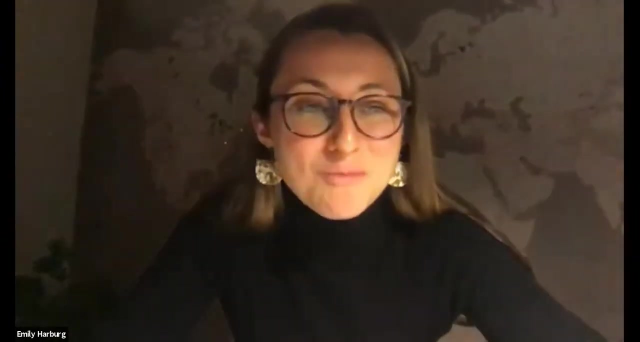 when we can just to give that breathing room to say what? how can we actually create this in the right way, um, and and look out for every unintended consequence that might come? to the extent we can control it, um, while also moving fast and not slowing too much that we miss. miss the moment too. 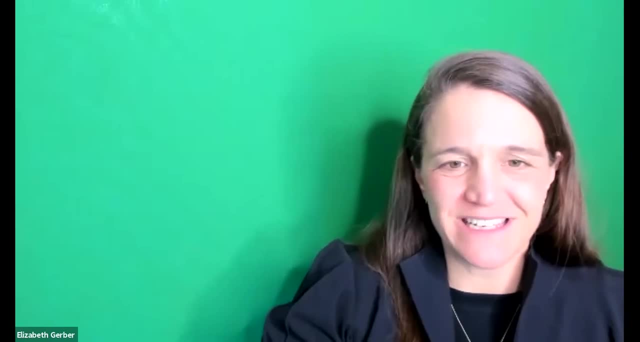 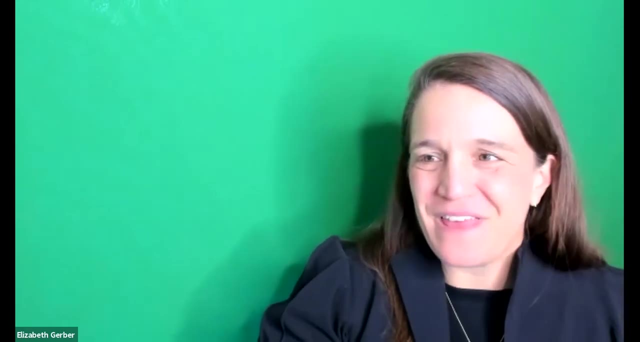 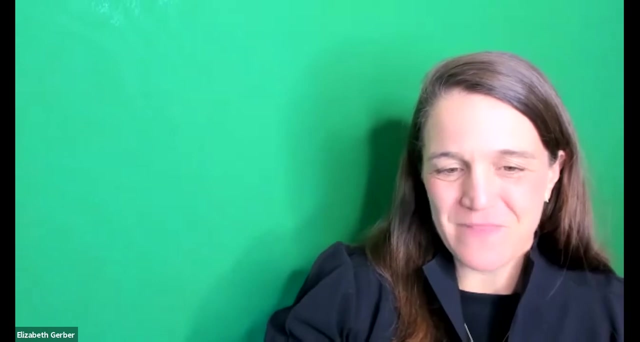 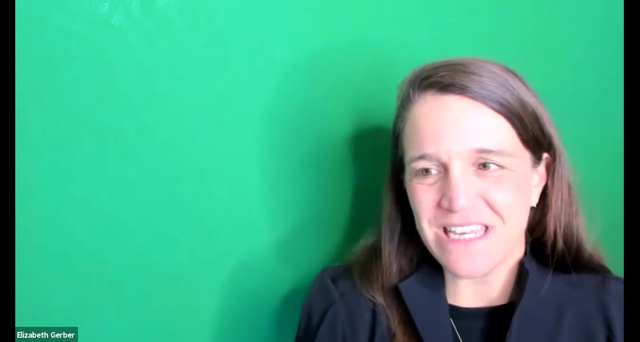 anyone else have a turn back time machine? any technical solutions? this, okay, wonderful, um. thank you. we're just near the end of time, and so i would love to wrap this up by hearing um some words of wisdom from each of you. we have many people listening in the audience right now, and i'd like um to invite each of you to speak for a minute or so. 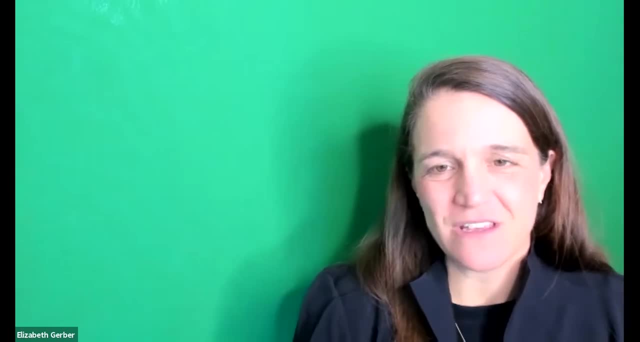 about what's something, um, after hearing this conversation, that you would like the audience to to do? um, based on this conversation and the needs of each of you, uh, to talk a little bit about your experience with this scale of the desegregation: what do you think? how do you think they can help? 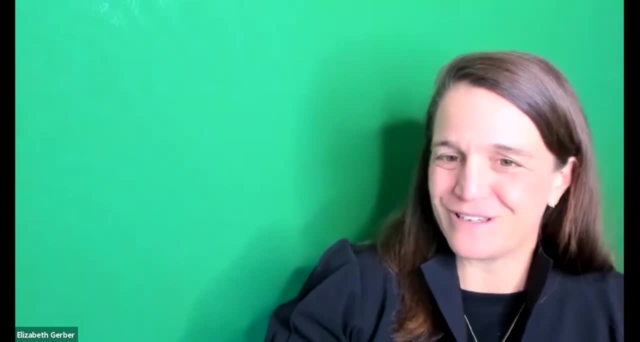 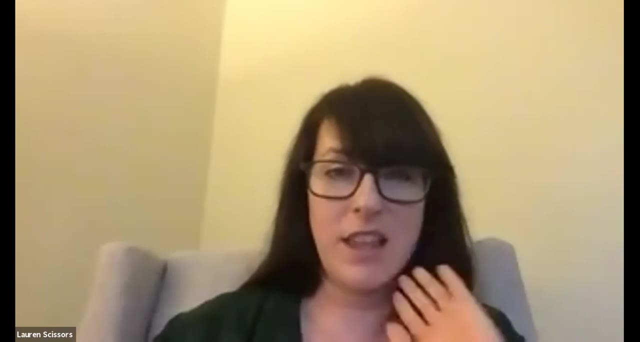 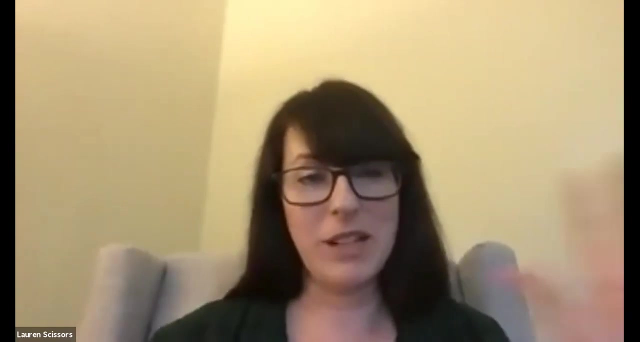 tackle these grand challenges and support you in helping tackle these grand challenges. and, um, i will let. uh, how about lauren? are you ready to go first? okay, let's start with lauren. sure, and i might be. i was trying to look through the questions. i might be imagining this. i thought someone maybe. asked like: what were the skills i learned, we learned in grad school that most helped us, uh, in our roles now? so i'm going to like parlay that question into my answer here, which is that when we are thinking about- we don't always, always talk about these things, we talk about it all the time. 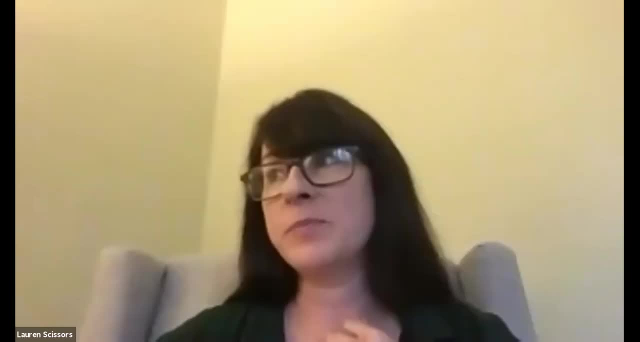 in a that. that's how i see, what i see. i see how we talk about these things. in my life, i'm not seeing them. it's all the time that we think about this one, i've been thinking about this one, which is that, um, there's no, there's no substitute for doing high quality research, um, 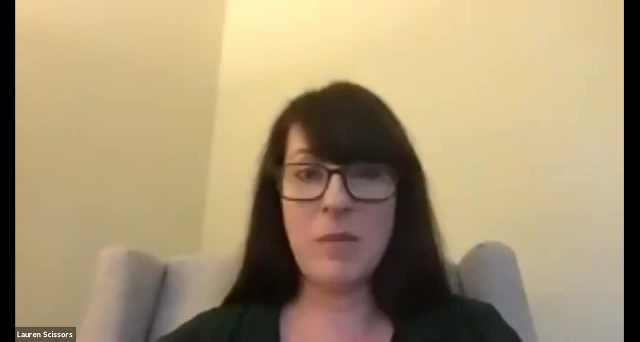 my, you know i lead a big team. uh, we do a lot of research, but i'd rather do half or a quarter of the amount of research, as long as it's done well, um, versus to just churn research out. and the reason for that is because when you do research well, that means you can rely on the insights. and when 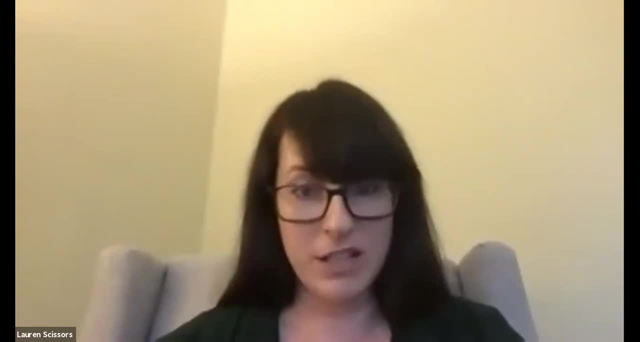 you can rely on the insights. it means you can really make good decisions. and so to me, like that's what i learned how to do in grad school, i learned how to do high quality research and that's taken me far, and it's taken a lot of folks on my team uh far as well, so that would be the 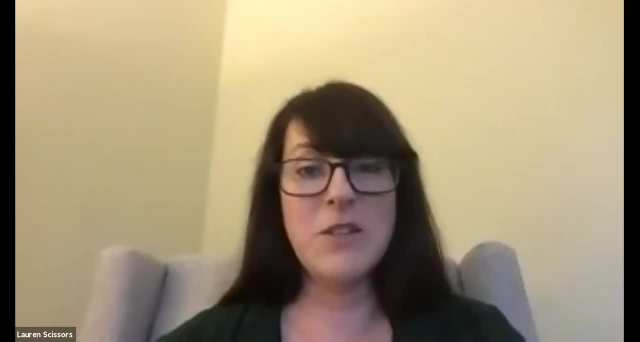 thing that i would want um folks to to know that there's so much value in doing whatever setting you're doing it in. i think it's valuable in industry. it's valuable, of course, in academia, um, and i think we won't be able to solve some of these. there's a lot of things that are going to. 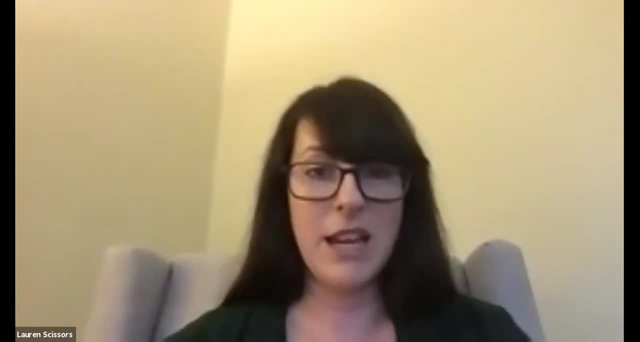 have to go into tackling some of the challenges that got brought up today, but i do think that in making decisions about how we go forward, we want to be informed by insights, and we can only get good insights if we're doing high quality research. to me, that's like the foundation of 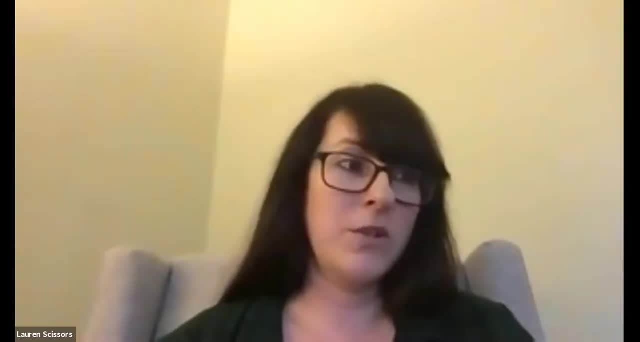 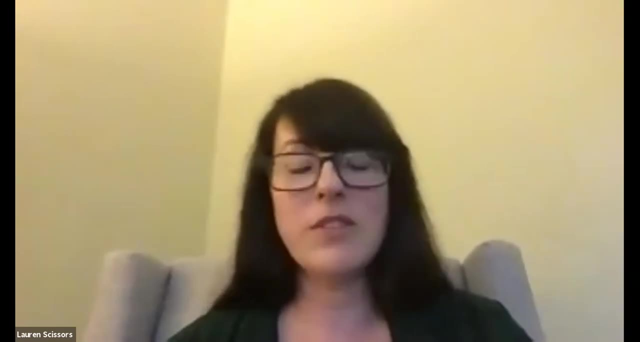 everything. yes, you need leadership. yes, you know, in order to uh uh get a strategy, you won't always have all the information. you need to be able to do high quality research, and i think that's like the foundation that you want. you know there's other things too, but but you have to have that. 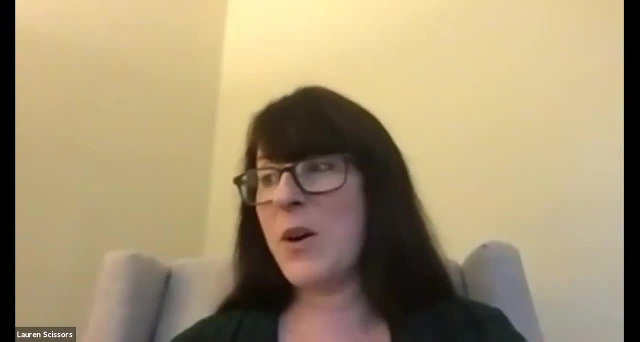 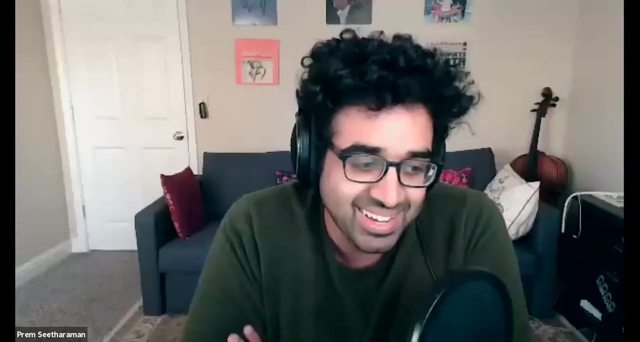 so if you're ever sitting wondering you know why am i in this, you know 10th methods class or whatever- uh, you know it's worth it. that's my opinion. thanks, lauren, for the shout out to methods. appreciate that. kream, do you want to follow? uh, yeah, so for me, grad school was kind of like it was becoming like uh. 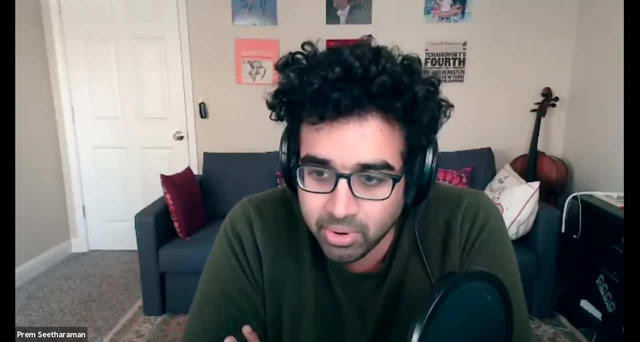 getting a style for research, and i think that's what i've been doing for a long time, and i think that's what i've been doing for a long time, and i think that's what i've been doing for a long time. research was like the most important thing for me, like getting a sort of unique perspective. 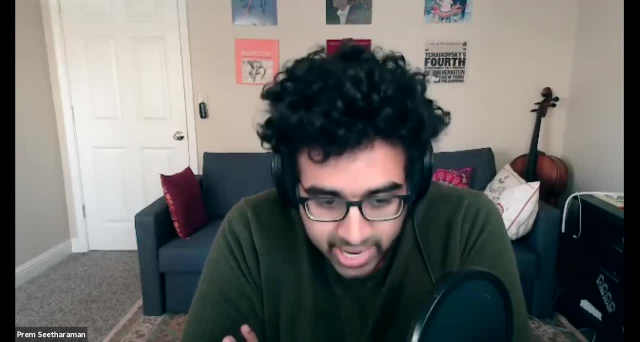 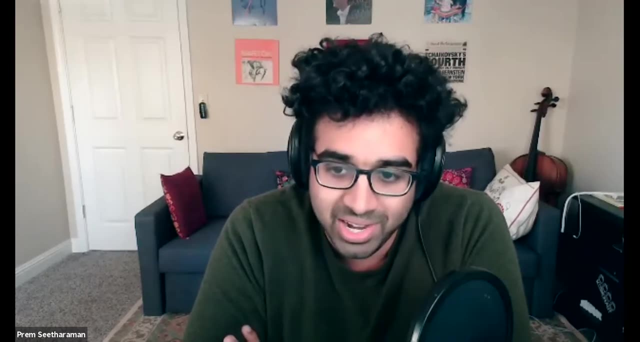 on tackling new problems, Because as you go through your career, I think, like tech changes, methods change, like a lot of things change, And the only thing that really doesn't change or really matures in a linear sort of fashion is how you approach problems, how you frame problems and 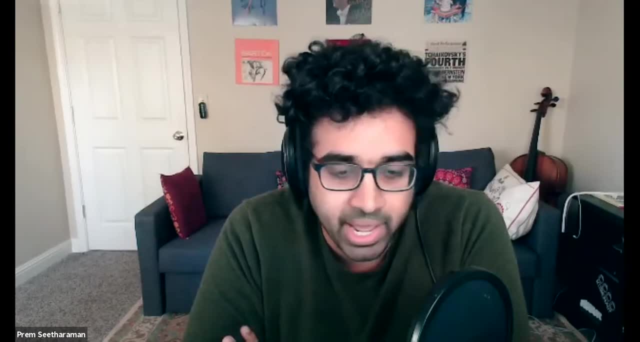 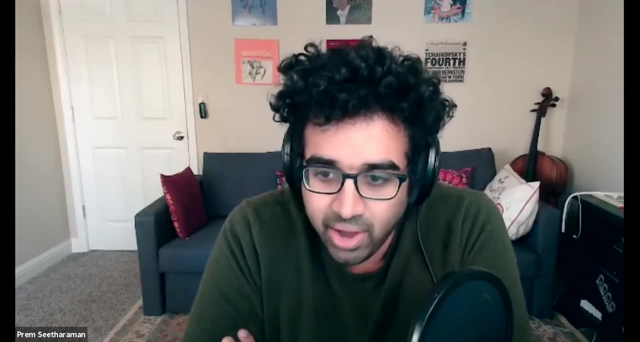 things like that And like for me- I mean the job I have now- it's just like getting a really good eye, for friction is like kind of what I call it, like looking at how somebody uses something or looking at some sort of maybe higher level thing that's happening is be like hey, there's. 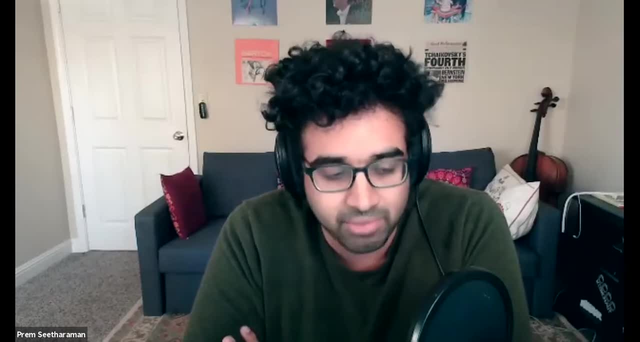 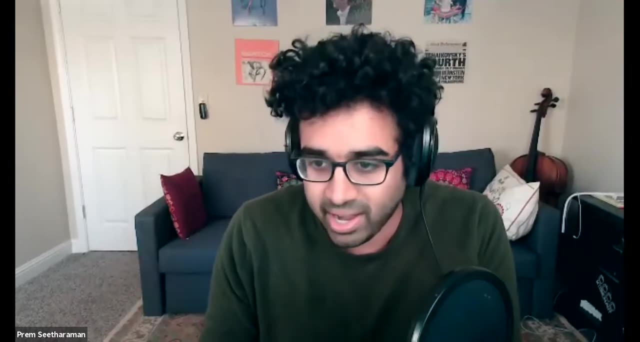 you know there's friction here, right. And then paring down all of that friction into things that that are currently in your tech skills bucket- right, Like I've got deep learning skill right now. right, Like that has been the thing that I've really improved on since leaving grad schools is 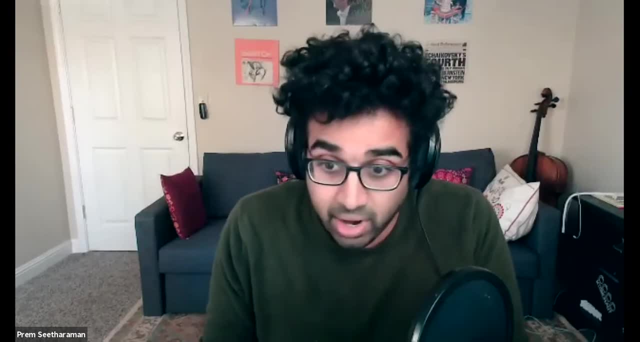 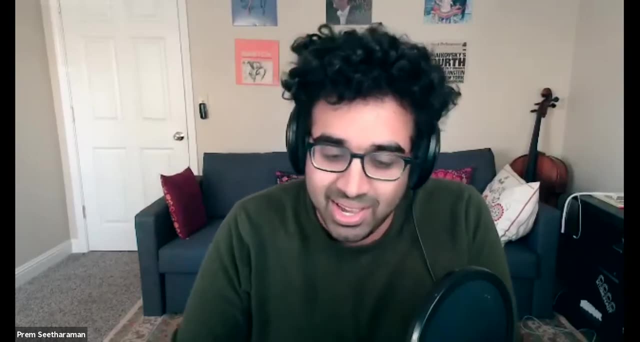 like my deep learning skills, like you know, very much higher than it was then. Yeah, Because of the people I work with and things like that too, And because of product pressure and stuff like that or like a lot of these things. really it's like a, you know. 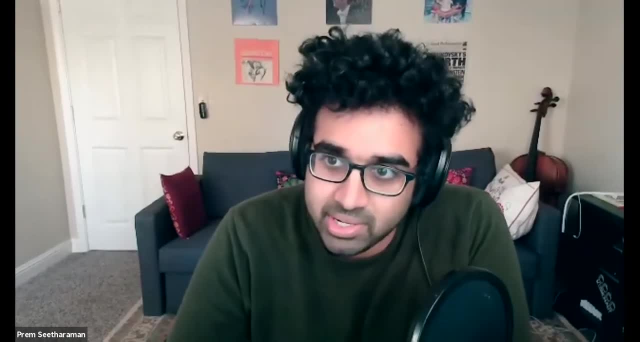 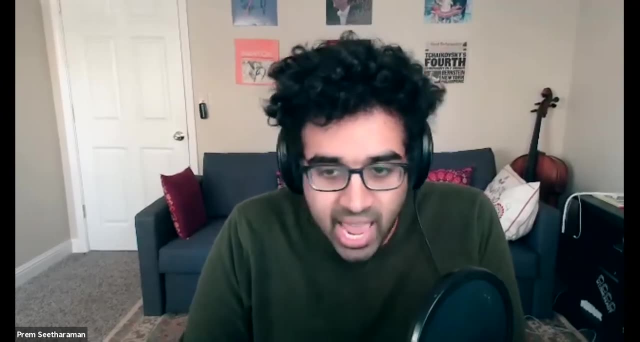 it's like a pressure chamber for your skill set in a lot of ways, But I would say that's like the most useful thing that you can take from grad school is developing a unique style and a unique way of tackling problems, Because at the end of the day, that's what you bring to the 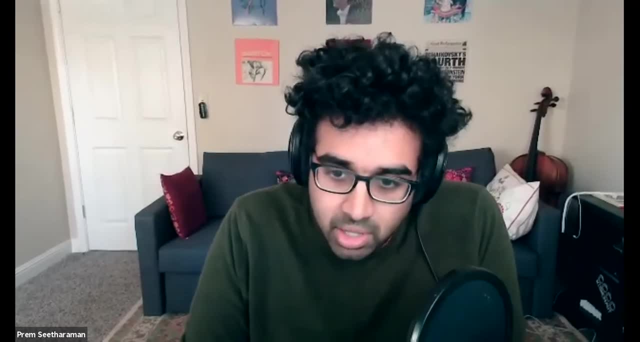 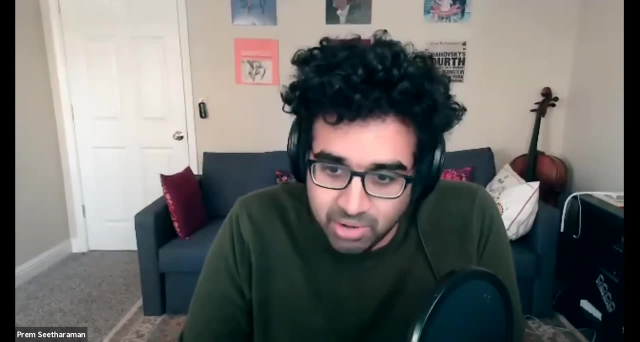 table is like your perspective on things And that's like the most important thing that you can have on a research team is a lot of competing perspectives and things like that, because it takes a lot of like minds to solve these hard problems. So 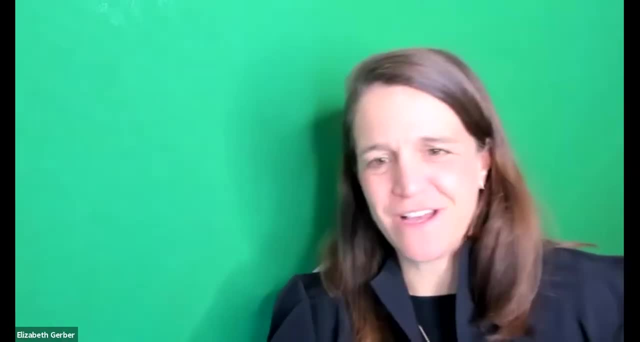 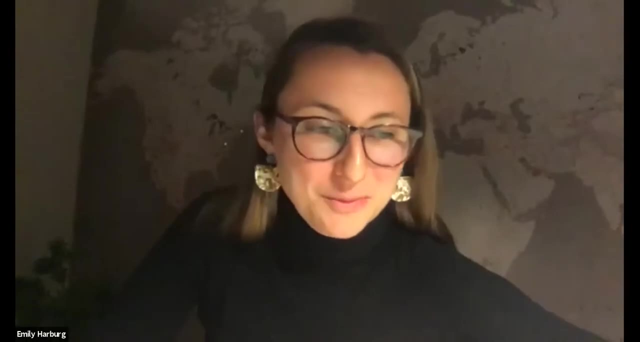 I love it. So study hard and trust in yourself. That's how I'm going to summarize those two points of view, Emily. Yeah, I would say I kind of echoing on both. I think you know, bring, bring your perspective. 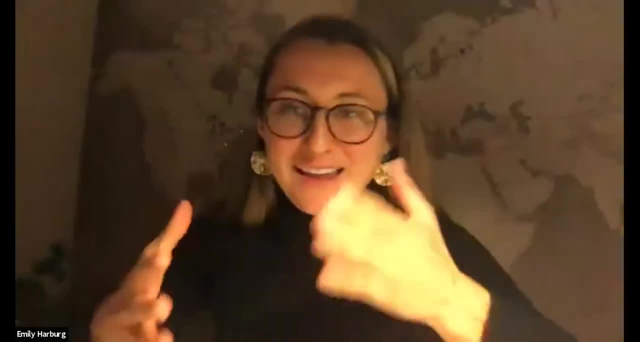 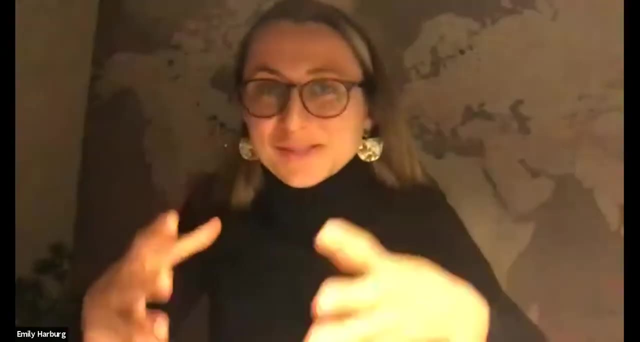 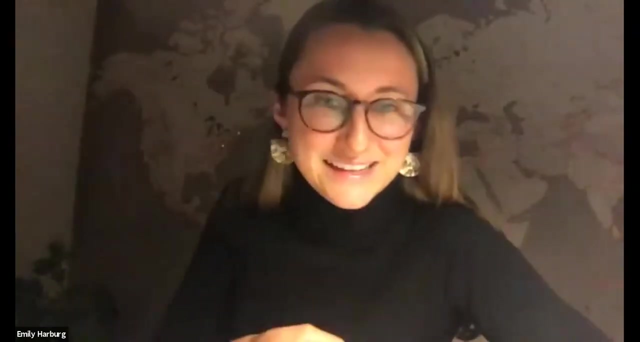 out into the world. I think what I've found is sometimes research can stay in the silos and we speak a certain language together and kind of connect and dialogue and grow and kind of those circles. But I think what I've found is when you're working on top of that, then yes, I welcome that new kind of perspective because 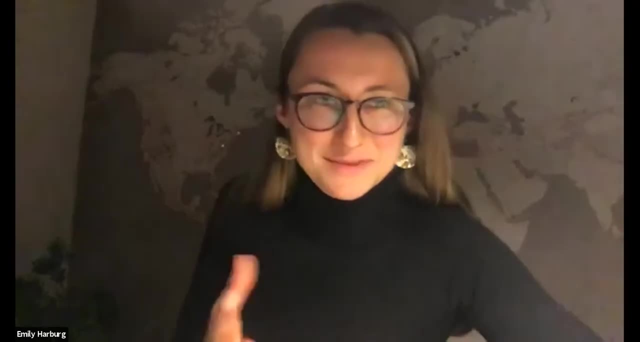 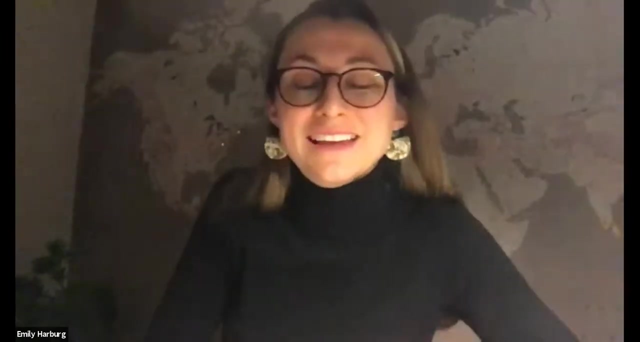 actually that can help boost your narrative, your project. So that's an important thing And I I think I would just add, and I think Lauren has resonating when you were saying earlier, like how much industry needs that research and wants to pull in researchers and 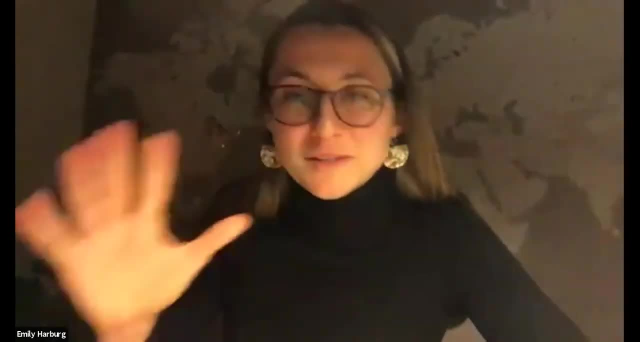 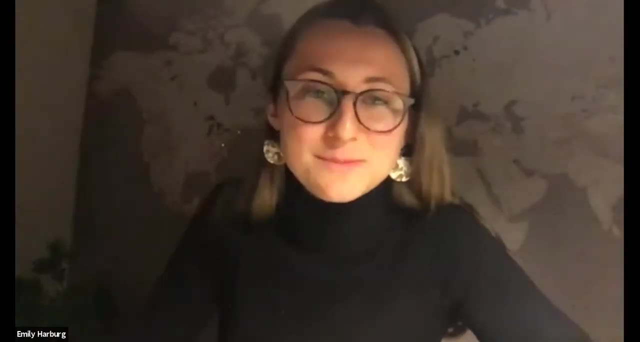 listen to them and learn from them and grow. grow with them, And I know my team is is so like dying for that, Like hearing what practices are out there, what's working and what researchers are saying about accessibility and belonging, et cetera. 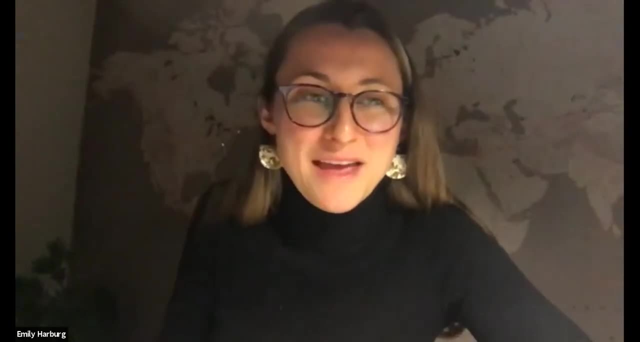 No matter if you go into industry or academia- like ensuring that you're kind of putting your car out there and and bringing in that unique perspective which I think you get to grow in building and grow and build in grad school, um, and and make sure that you're kind of not keeping that kind. 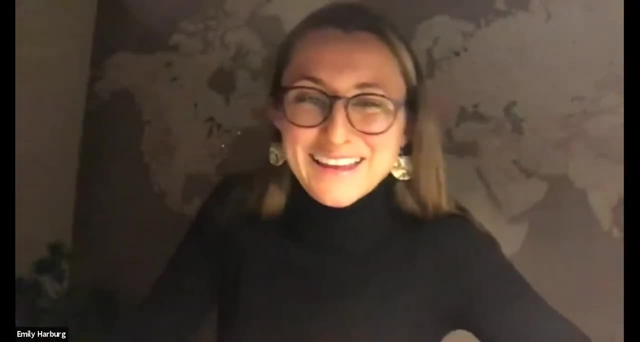 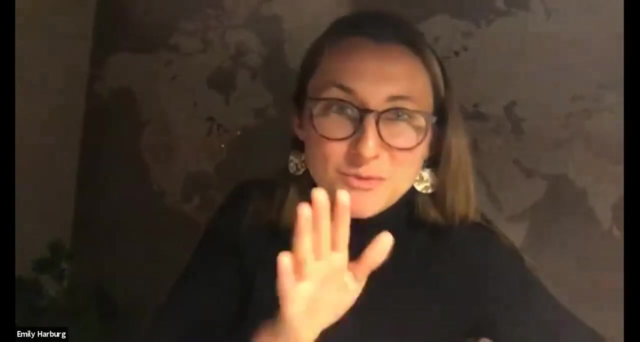 of been in, you know, one in a paper, but like getting it, getting out there and sharing it, um, because i, i truly think bringing that hci lens into what we're building and where technology is moving is so critical, um, and so i think, bringing kind of the diverse perspectives that we have, 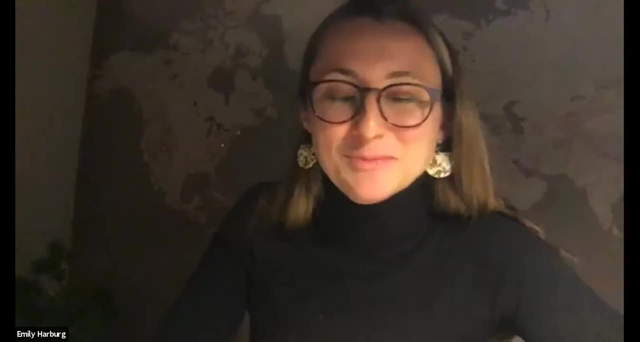 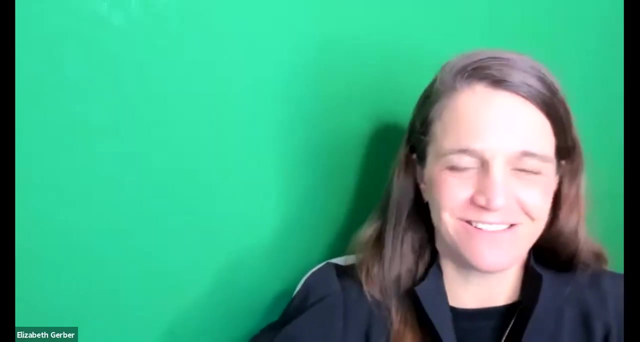 um, will make everyone everything kind of stronger. so i guess it'd be, in short, like: make sure you're sharing it and getting it out there, believe in yourself, study hard and share, love it. uh, isaac, are you ready? yeah, yeah, i'll come back to, i think, my point about constraints, because you know when you. 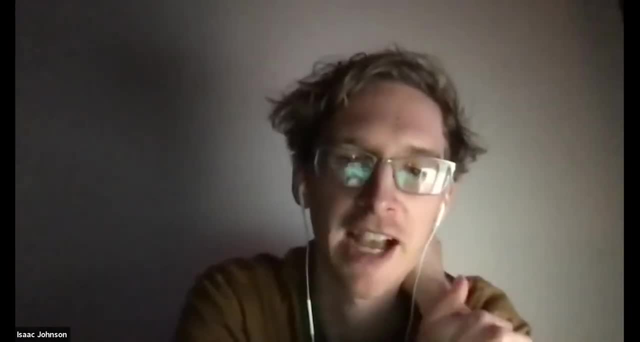 transition from academia to industry. uh, you often get access to like a lot more data and like power and all these things, and it's really tempting to just like want to build bigger and bigger things and, like you know, really just like use all this data you have. um, and i think in many cases it's 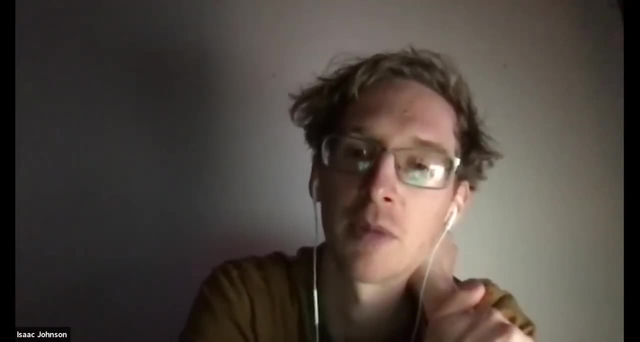 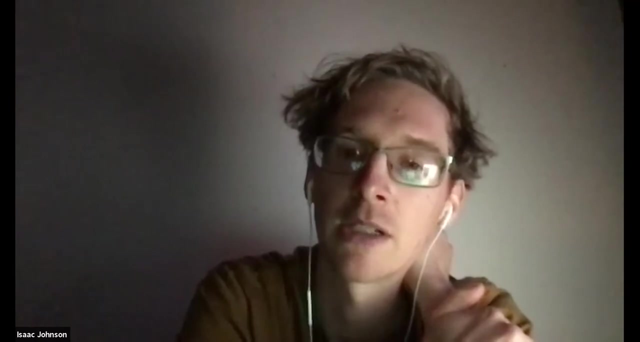 actually very valuable to kind of set yourself constraints. it really helps with the design. you know, for me i've talked a lot about language coverage and making sure what i'm building isn't just going to work for a single language, um, but you know, this can also be things with privacy, transparency, all sorts of you know. 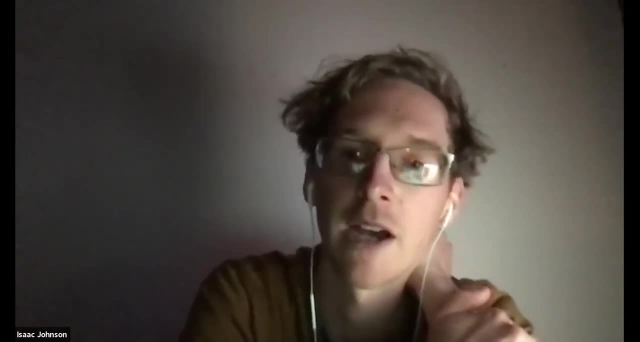 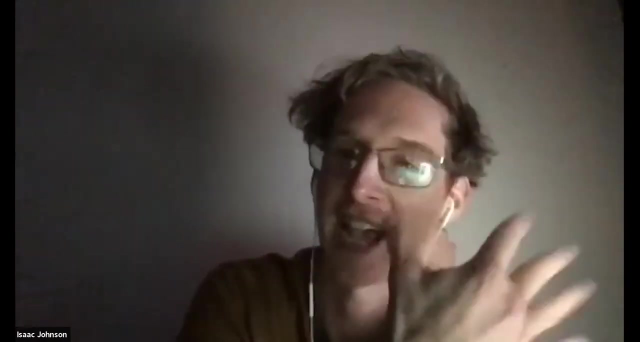 constraints that you can bring into your work, and i think they bring a lot of value. and so, just thinking about what are those pieces that are really important to me and like, even if i uh get all this access to data and things like that, like what, i don't need to use it though. right, you don't. 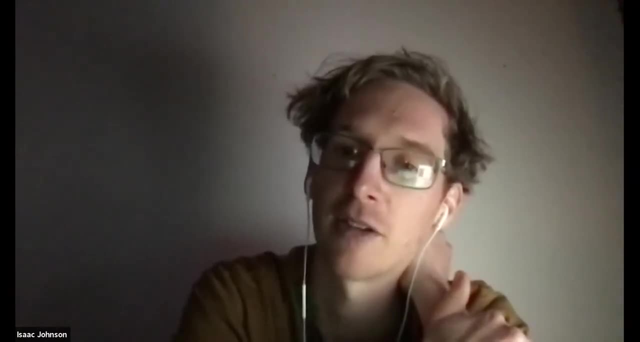 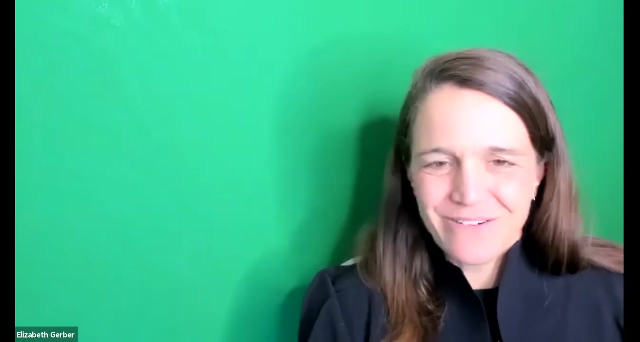 have to, you don't have to use it. you don't have to use it. you don't have to use it, you don't have to consume it. you can kind of push back at on some of that mentality. that's lovely. thank you so much, isaac. um mark, you want to wrap us up here, sure um very much on uh. 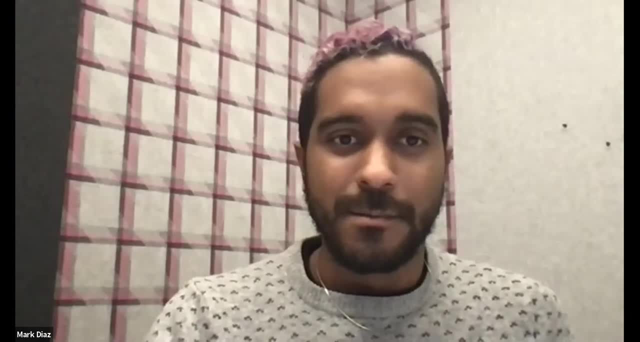 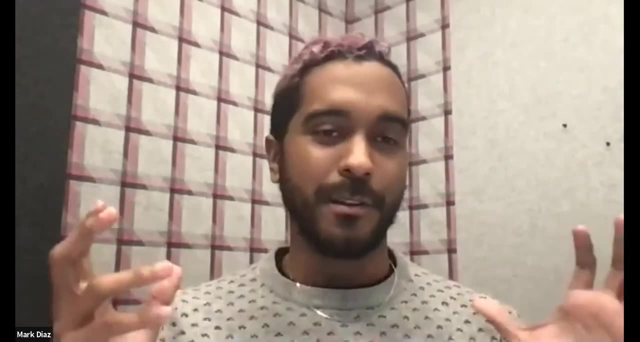 this, i think, a broader theme of like communication that's come up. um i like i jotted down a note which was ask yourself how to convince- like when you're thinking about a project you want to work on, or you're trying to convince somebody that a research project is going to work on, you're 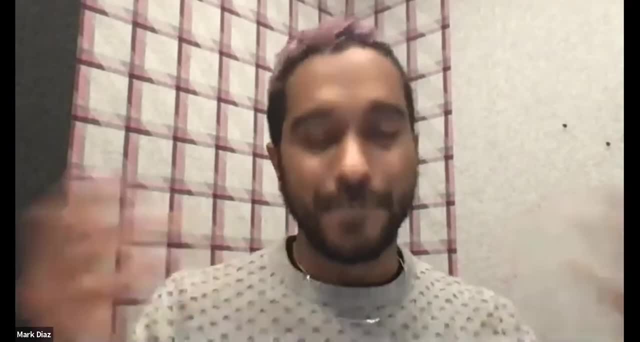 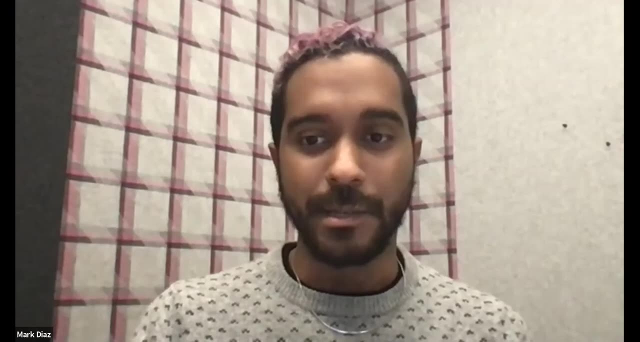 trying to convince somebody that a research question is important. i think it's really great to ask yourself- and if you're in, you know, interested in being an industry or at least working with people in industry or outside of the um academia, ask yourself how to? how do you? 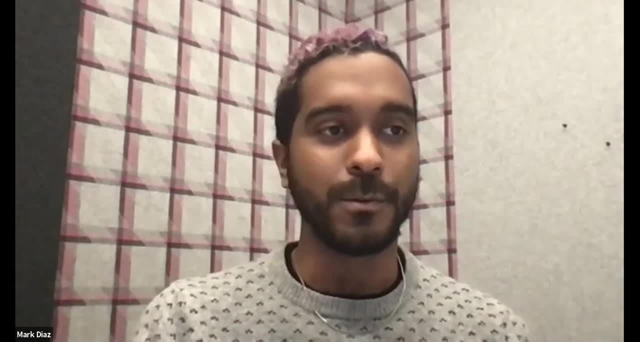 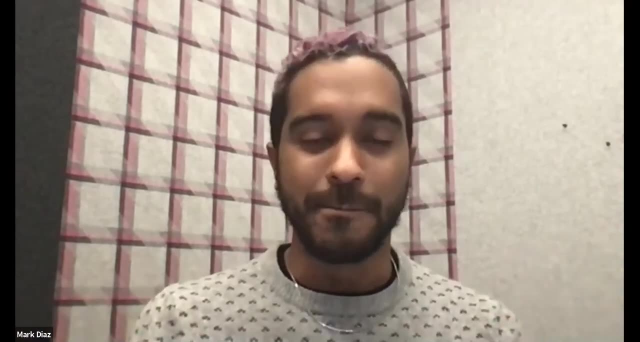 convince people. how do you persuade people? how do you get buy-in from people who aren't sitting at the university and i feel like that sounds. maybe it sounds obvious and or it should be, but i mean, we spend so much time refining our language and our writing for. 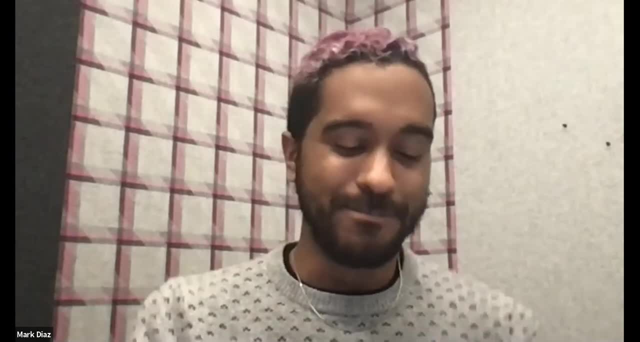 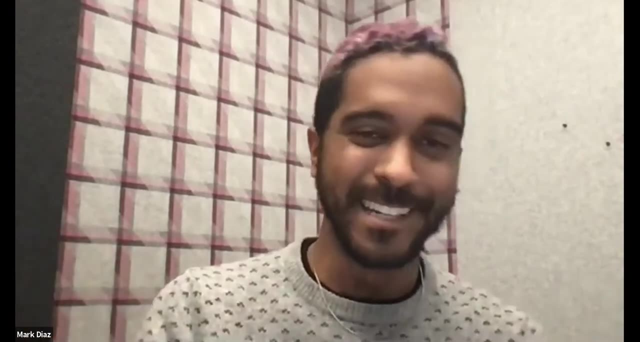 what we write, that we spend so much time on the journey of like, what's the way we say things about? what we do is change the way we think about science and the way we write about how we represent our world and the way we think about our questions and our 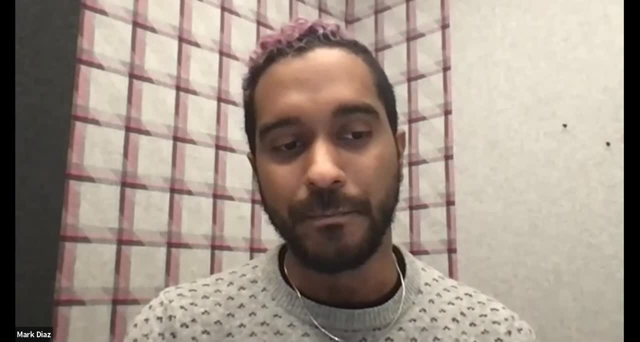 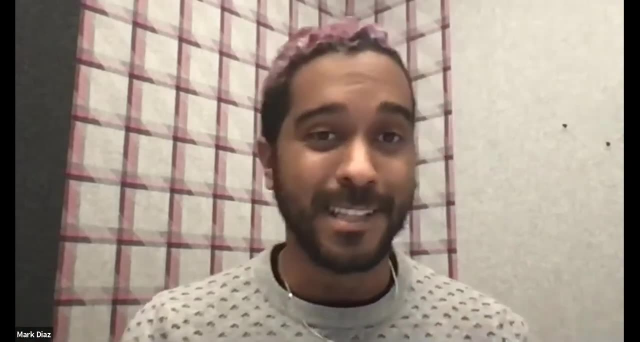 approach to our young years in general. so that's been a really, really good place to be and i think that's a very good way to be, kind of like a sort of gap where you are. you're not always there to be, so, um, i, i, i'll just, i'll go ahead and ask you to just throw. 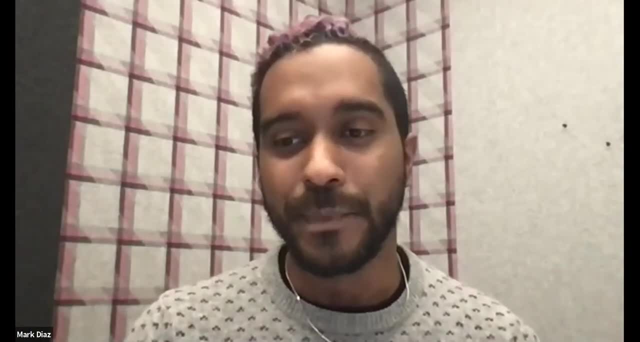 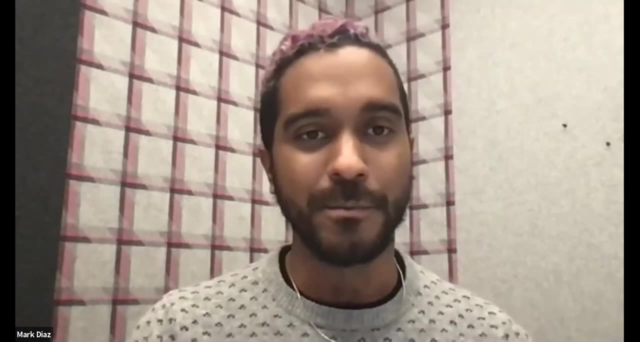 this out because i just want to um, to kind of give a quick segue: where do you like the? and? so I think, yeah, being able to articulate to different audiences, whether it's, I don't know, going home, Thanksgiving's coming up. if your parents are not academics, try convincing them. 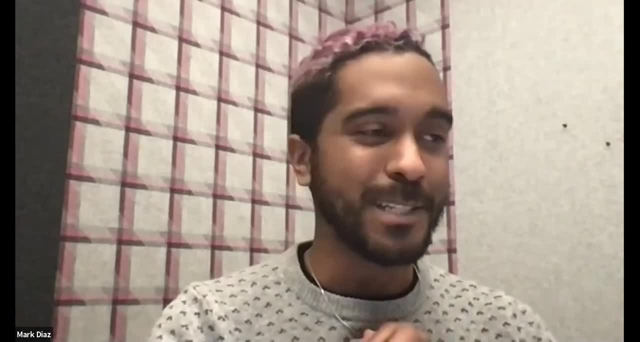 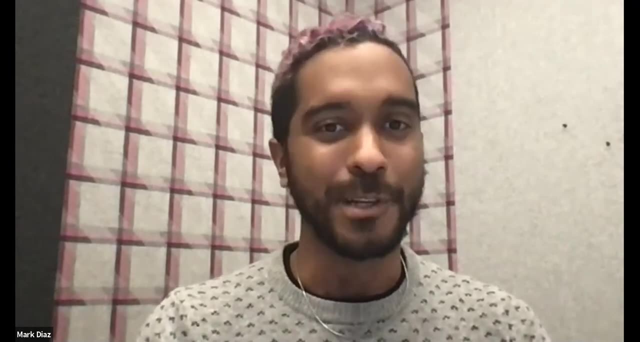 of your next research study and see what they think I used to dread going to parties with friends while I was a grad student. they'd be like: what do you do? what do you research? like, oh god, they're gonna be like: why is this important? and then I have to answer that question. 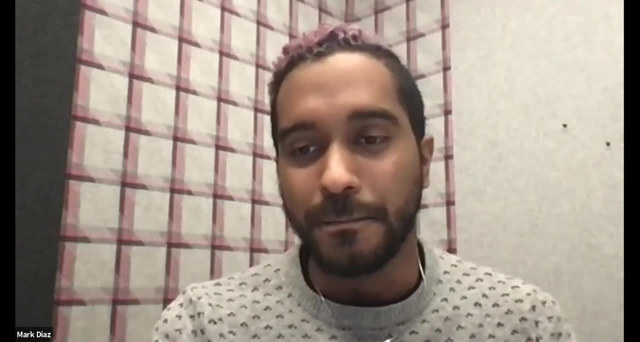 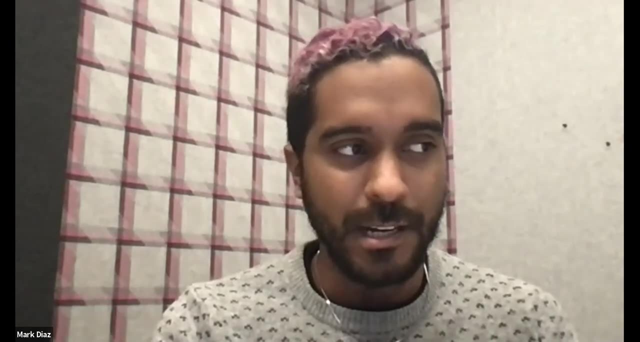 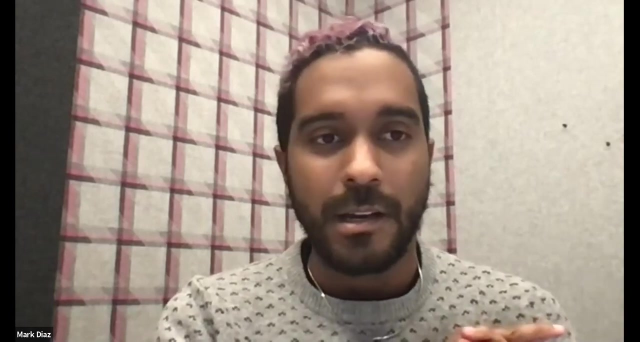 and it can be hard sometimes and I'll do a quick, give a quick plug to the center- oh, I'm actually forgetting if this is the exact name, but the Center for Civic Engagement. on campus I took their geo seminar which was sort of framed around how to be like a public scholar, but one of the 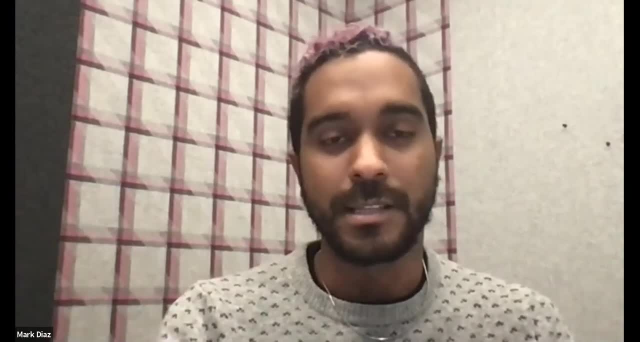 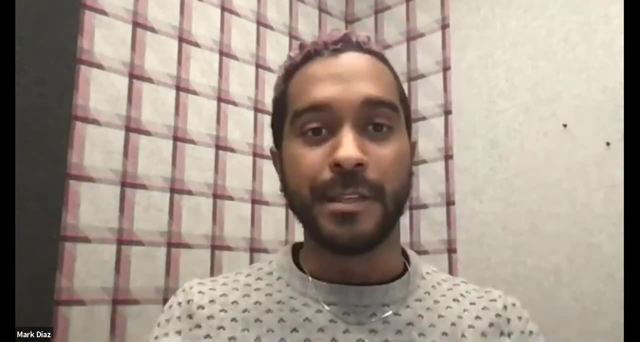 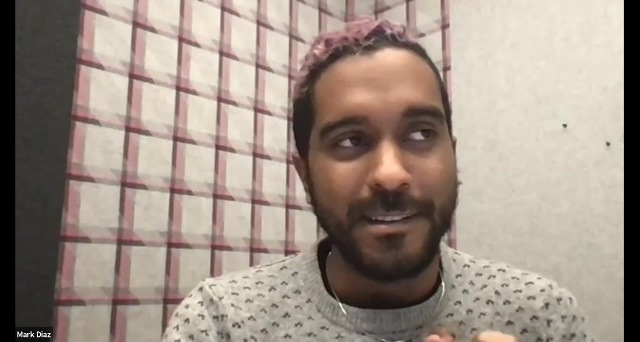 core points of that was: how do you communicate to people outside of universities, outside of academia, because you have important knowledge and and questions. you're researching for broader communities, so those broader communities should have an access point to those conversations. I think that's a very- it'll be a very- useful skill.